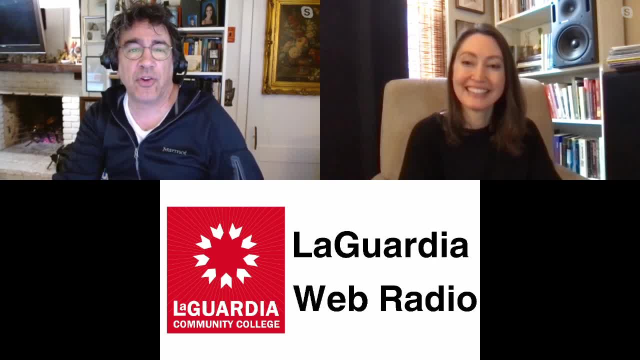 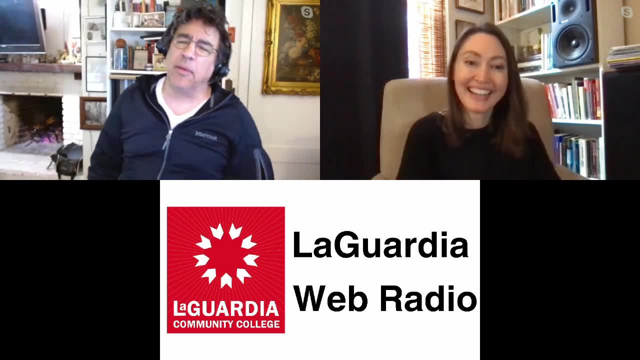 on to discuss her work in the area of philosophy for children, And welcome back Dr Carr, who is a regular on the show. How many times have you been on the show? I thought only twice, but I'm so happy to be considered a regular. Hi, Hugo. 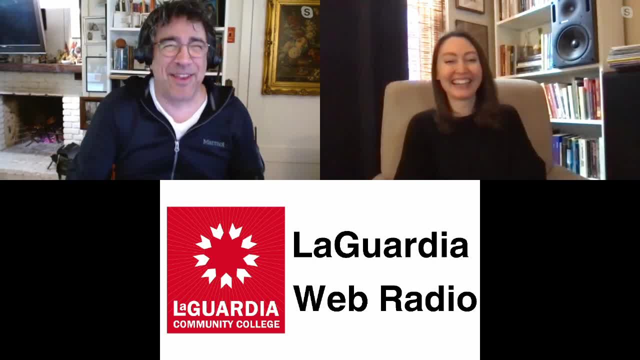 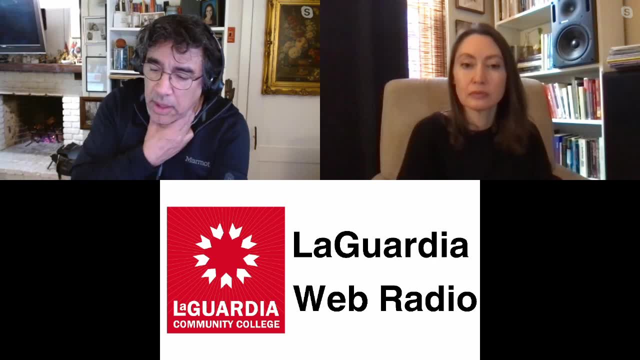 Yeah, If you've been on the show more than once, you're a regular, But you make a big impression. One thing that I would say, too, is you've been instrumental in helping me put together guests who have joined me for May It Please the Court when I was doing the shows about. 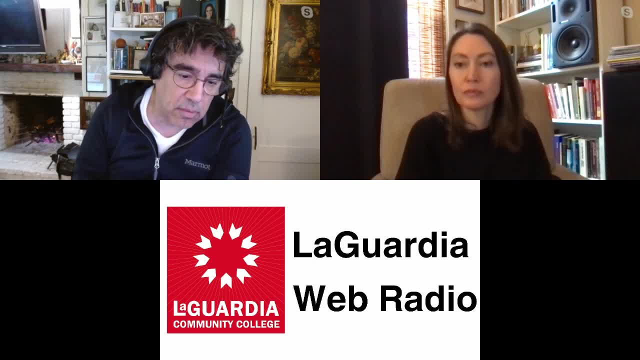 reproductive rights As they were played out in the Supreme Court cases over the years. we never got to go through all the cases And then, all of a sudden, Roe v Wade was reversed And I believe we did a show right around that time as well. But just thank you for that. And, by the way, 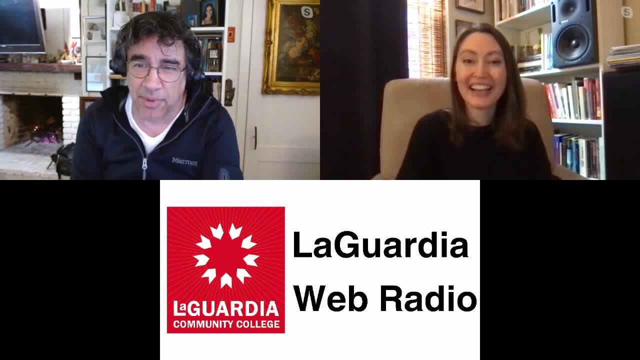 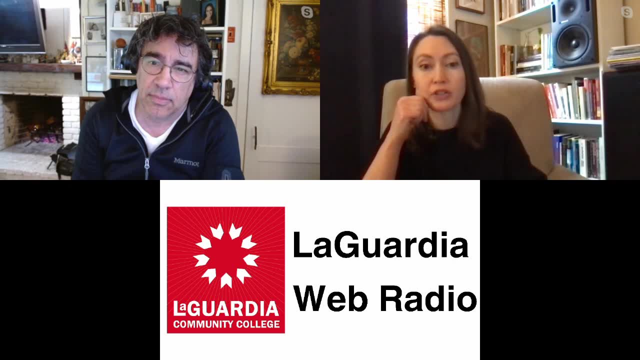 I would love to go back to doing that again, So we should talk about that at some time, Definitely, Definitely. I imagine there's a lot of interest in talking about, you know, the Supreme Court right now, not just with regard to reproductive rights. 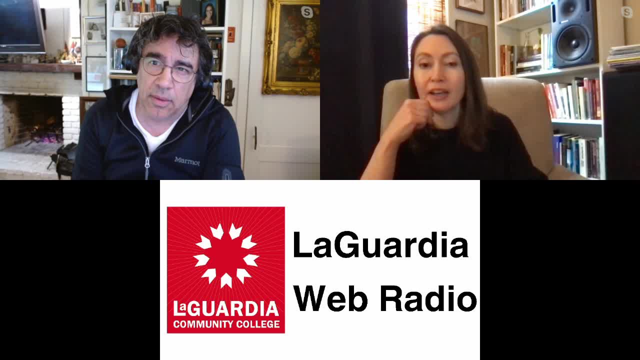 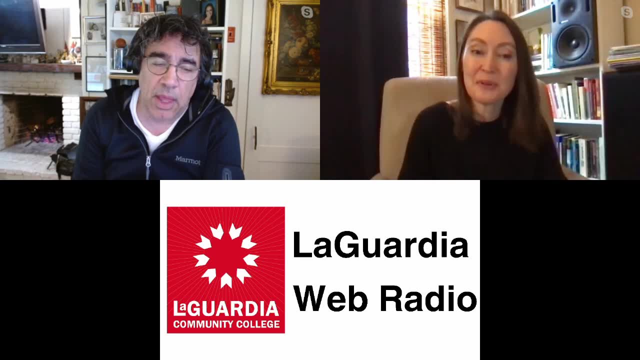 but also, you know, larger issues in the Supreme Court and our relationship to it. So we definitely have people who, I'm sure, are really excited to talk about that And, yeah, let's set something up. You know that's what they tell me, But you know, getting them on the show is something else. 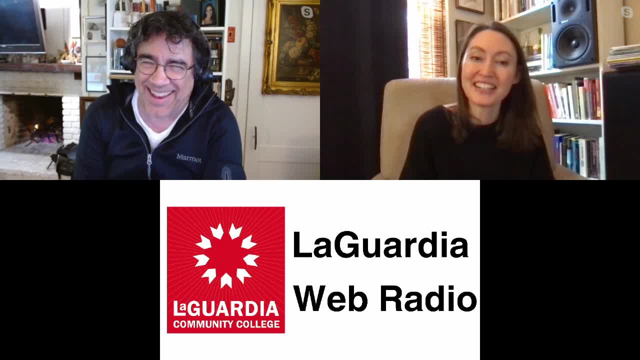 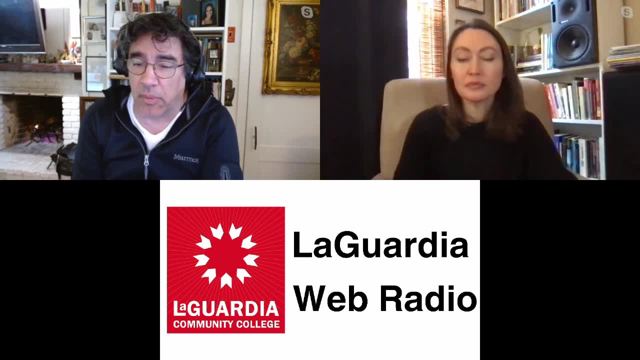 It's always a challenge, right. The scheduling is always a challenge, Right. My reach exceeds my grasp. So, but today I want to focus on something which is- you know, I know you've been involved with for quite some time- which is the subject of philosophy for children. So let's just hit the 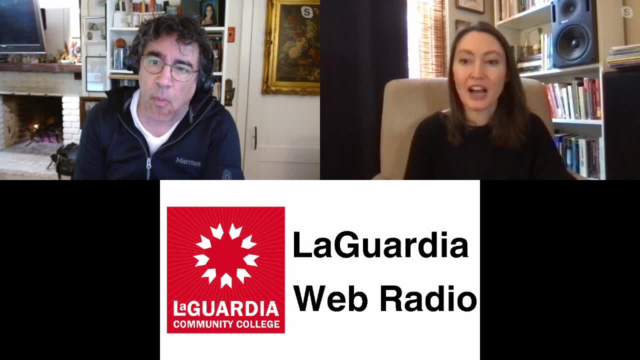 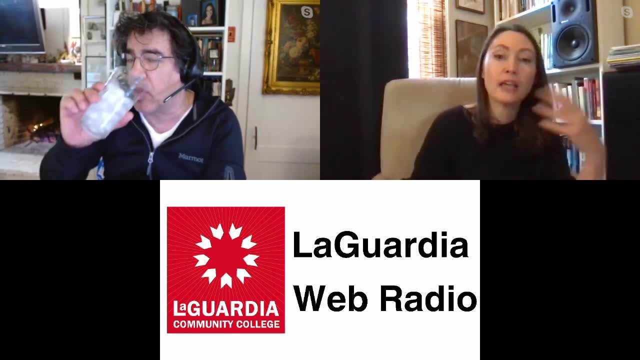 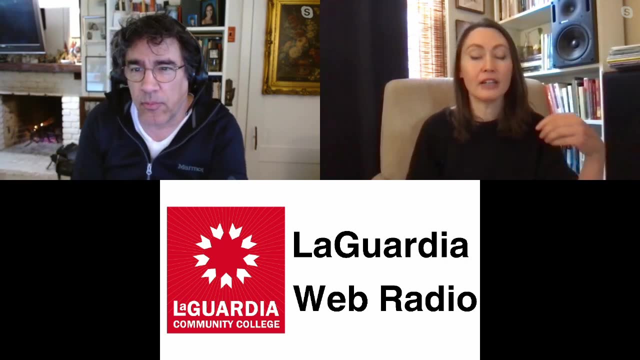 ground running and get started on that. Absolutely So. I'm Dr Sherry Carr. for those who don't know me, I came to, first of all, I came to philosophy as somebody who was, you know, interested in, interested in reading, interested in thinking, interested in talking. 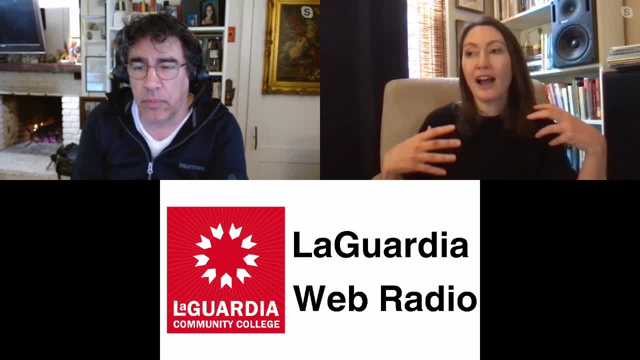 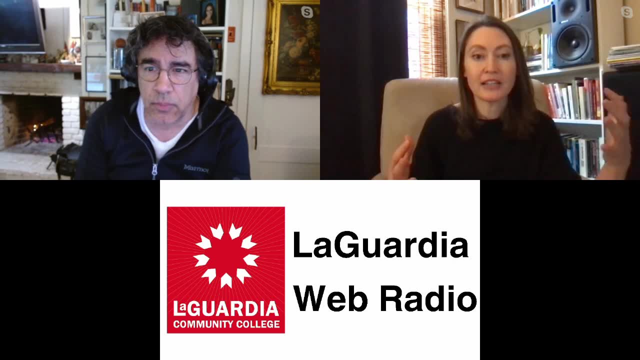 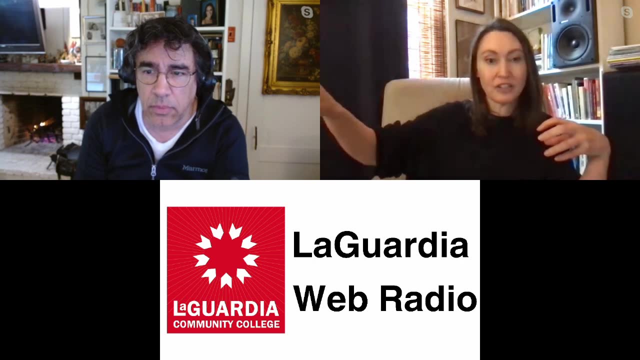 about ideas. I came to philosophy because I took a bunch of other you know classes in college and then realized that, oh, I get to just talk about ideas and philosophy And if I do philosophy it's just going to make me better at doing any of these other things that I'm interested in doing. 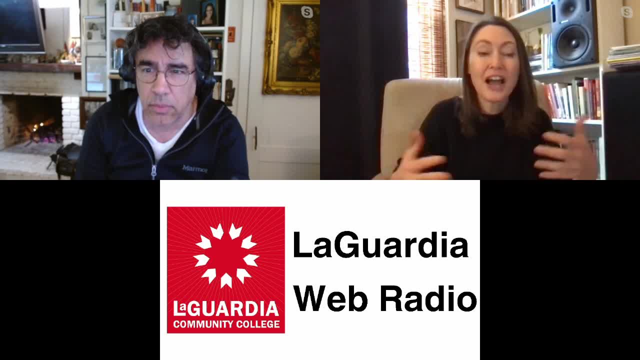 Because, you know, I didn't want. I was young, I didn't want to close off doors for myself. So I thought, oh, I'll start, And that way, when I want to switch later on into something else, I'll be in a good position to. 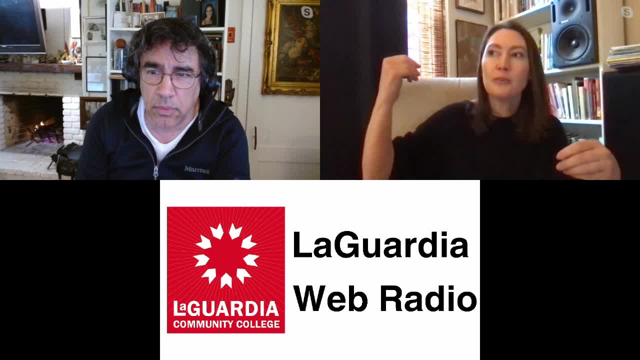 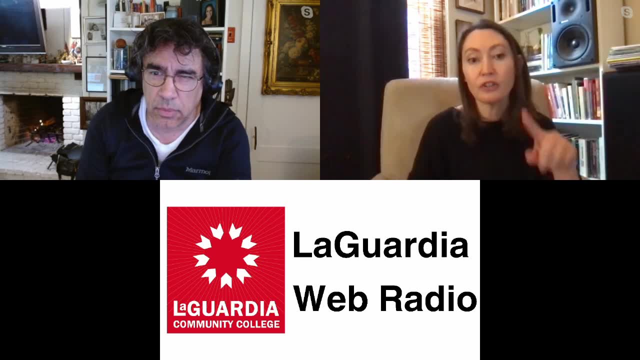 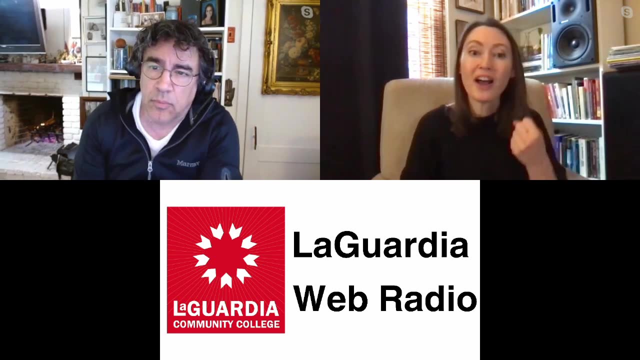 like understand what's going on and do a great job. And it turns out I just stayed in philosophy because I liked it, And one of the reasons that I liked it so much: the very first philosophy class I ever took was in the philosophy of fairy tales, And that was the one that hooked me into. 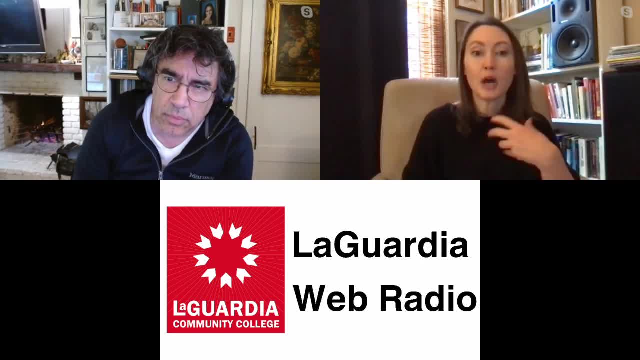 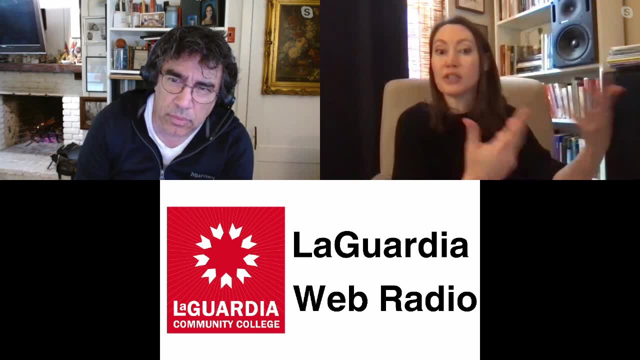 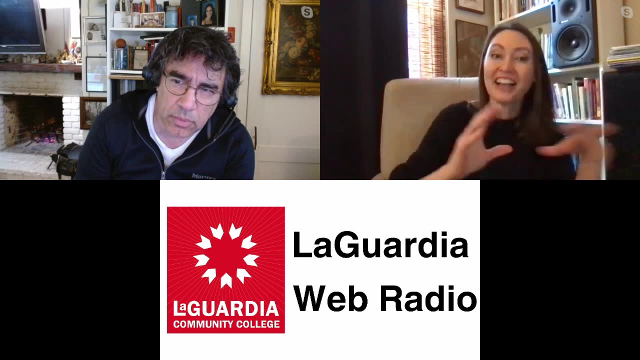 philosophy, because it was this beautiful class that was about how our relationships, our relationship to the mythologies that we tell to ourselves and to our children, has shaped us through the centuries. So, after taking that class, and that being the hook that brought me into philosophy, then I get to my grad school and I'm at the University of Memphis. I'm from Memphis. 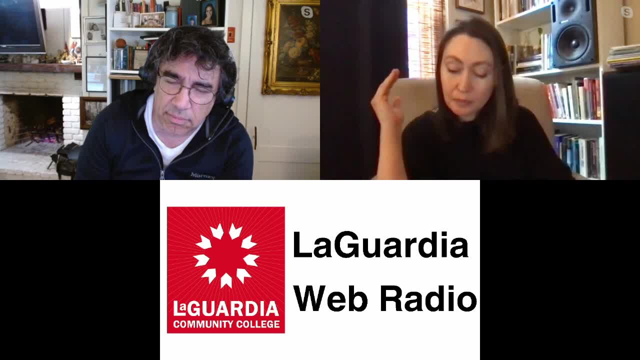 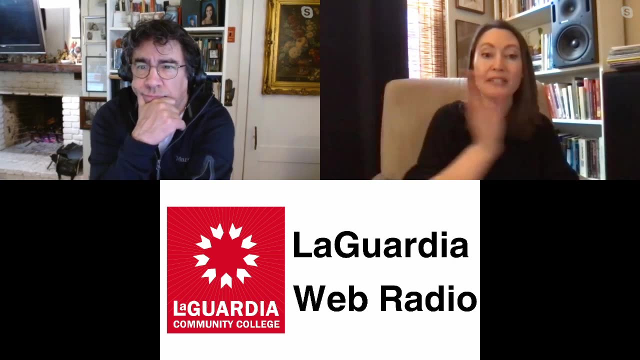 I'm sure you can probably tell with my accent- And we had- I had a fellow graduate student there, Michael Burroughs And Michael, if some of you might know his name, he's gone on to create a really incredible public philosophy ethics center down in Southern. 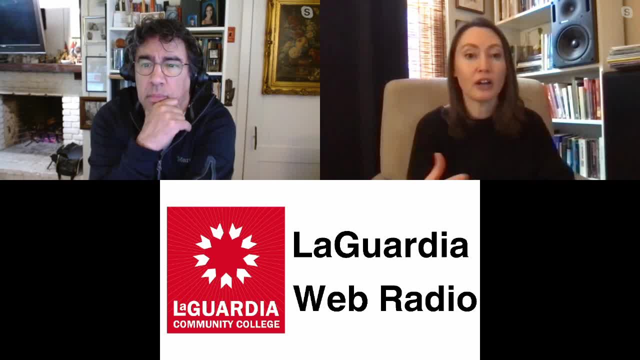 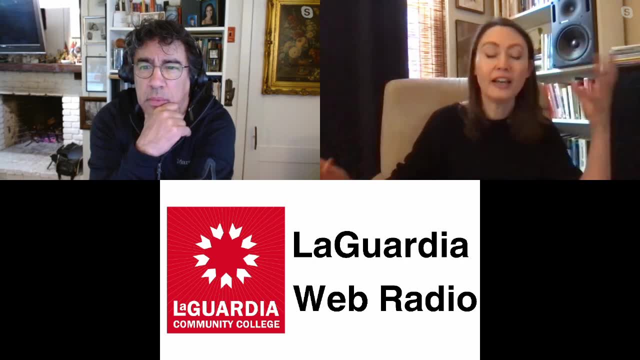 California. He was the executive director of the Philosophy Learning and Teaching Organization, which is the premier sort of philosophy for children organization in the country. But at the time he was just a graduate student And he pulled together a bunch of graduate students like myself to start to offer philosophy after school enrichments for the on-campus. 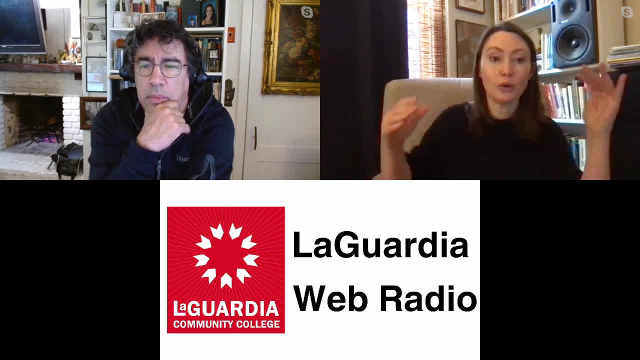 children, on-campus school children, So children who were in the range of like second to fourth grade. So it was really that introduction that brought me into philosophy for children And that allowed me to bridge that interest that I had had that brought me into philosophy in the very first. 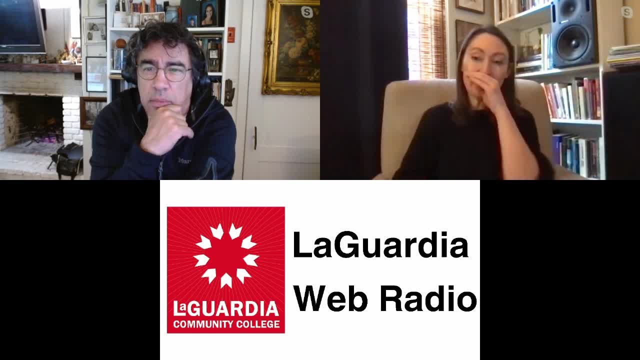 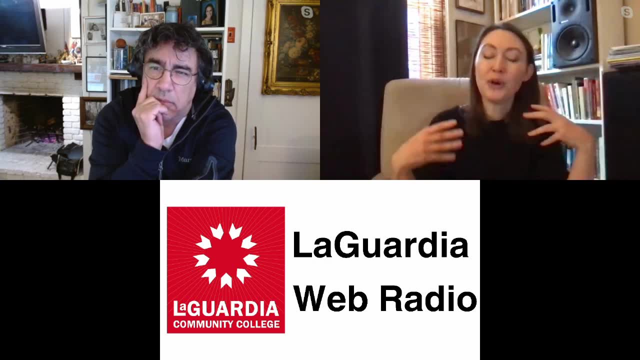 place which was philosophy and fairy tales. So that's, that was a little introduction about me in relationship to the field of philosophy for children. But you might be asking yourself what is philosophy for children? So I'll give you a little description of philosophy. 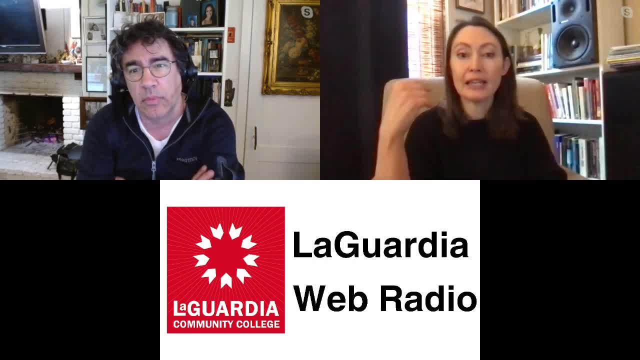 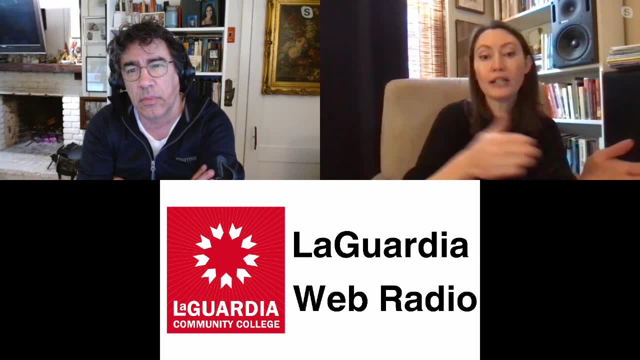 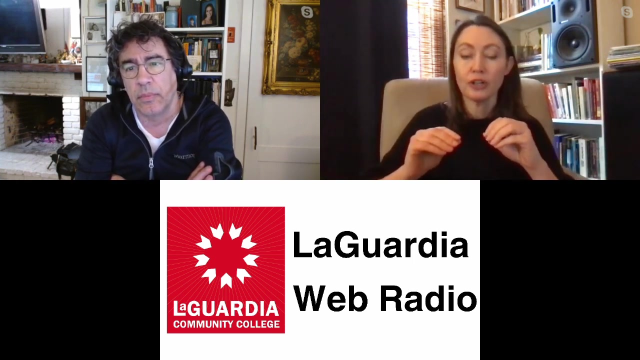 for children. Philosophy for children is an international movement of philosophers, thinkers, who want to introduce philosophical thinking to pre-college kids. Very simple: It's actually a very well known movement and the. it was a fight against racism, but that movement boosted it. 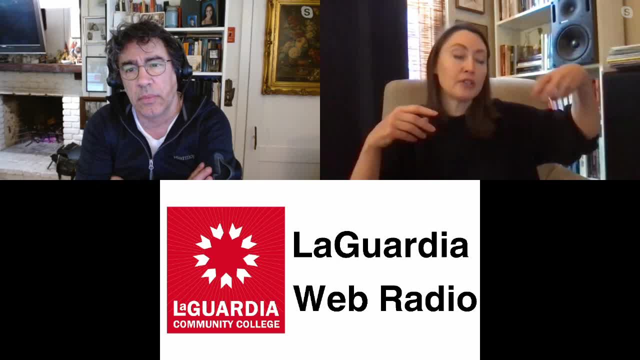 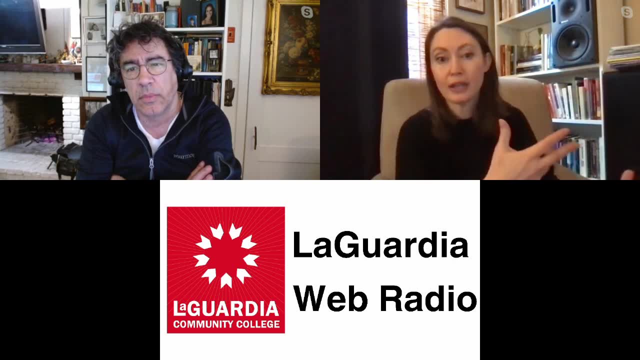 So actually, the origin of philosophy for children as a movement was actually locally. There was a professor- he was at Columbia at the time, Dr Matthew Lipman, who it was the late 1960s He started thinking about. oh okay, so he's, in this context, think of the late 60s of incredible. 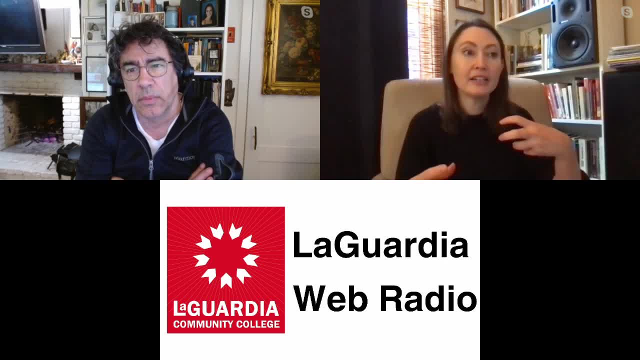 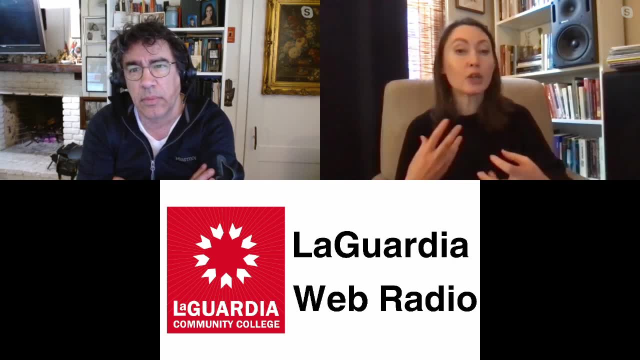 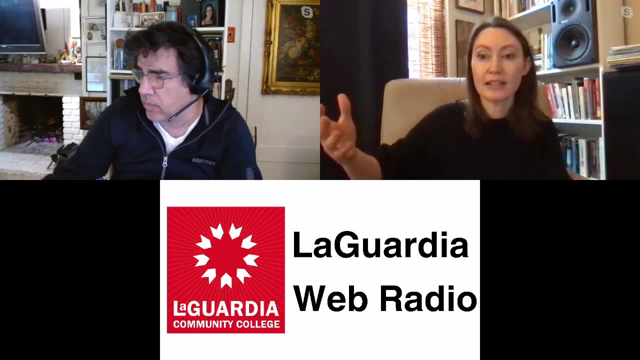 a lot of political division at the time and a sense amongst many people that there wasn't a lot of reasoned discourse happening right, And so for him he was like: okay, so how can I help, How can I wade into this dialogue? And he thought, hey, I can help to create better. 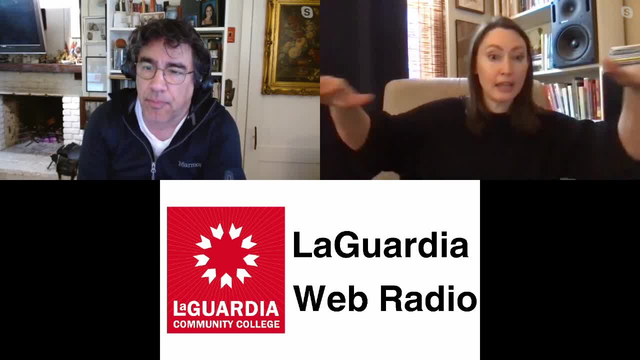 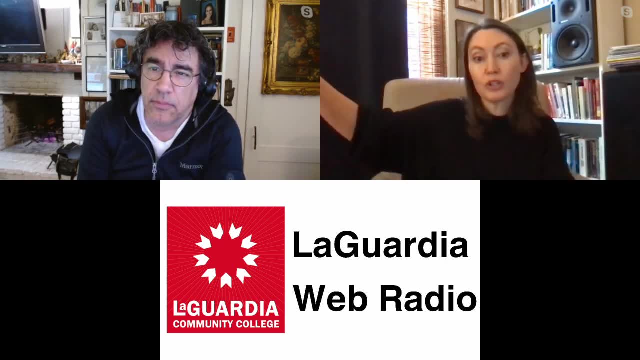 civil discourse right in the society by supporting people's thinking from the time they're children all the way up to adulthood. And he wanted to argue that, hey, this historical discipline, philosophy, been around for thousands of years, that we were in the best position. 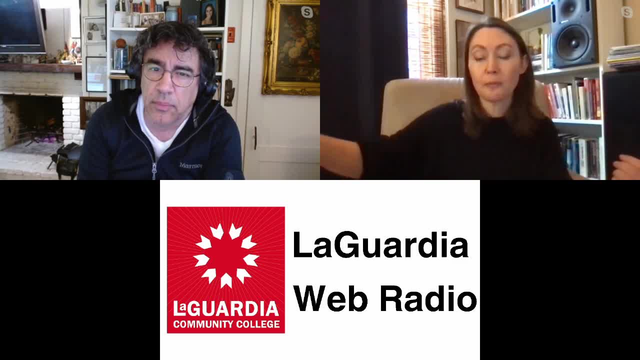 to be able to do this kind of work, And that one of the reasons why we saw this kind of partisan polarization, where we saw the breakdown of reasoned dialogue, was because we didn't focus on this type of education. when people are young, We wait until they get to college. 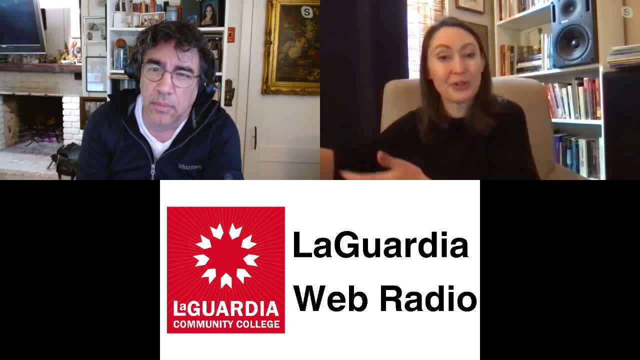 and then they get some philosophy and some classes in reasoning and critical thinking and argumentation and those kinds of things. So he wanted to back it up and started there. So originated in New York up at Columbia, Matthew Lippman, moved out to New Jersey. 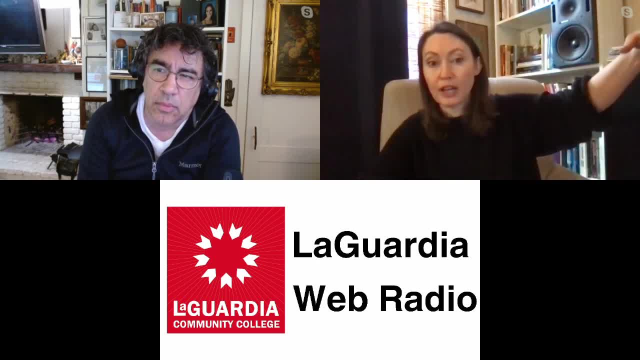 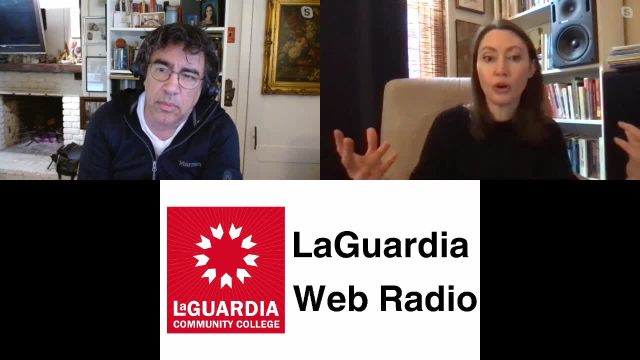 and then he developed his first, you know, sort of philosophy for children organization, which was based in Montclair And from there it's really grown across the world. So there's philosophy for children, organizations and outreaches, some of which are attached to. 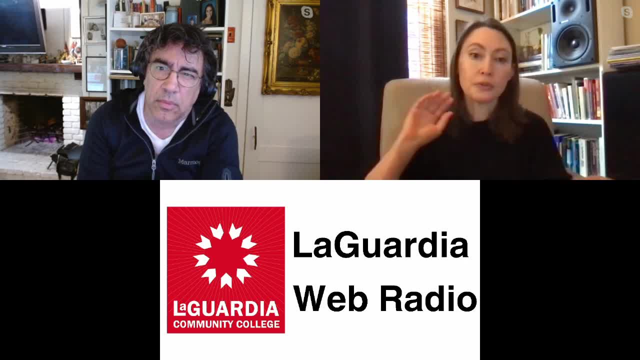 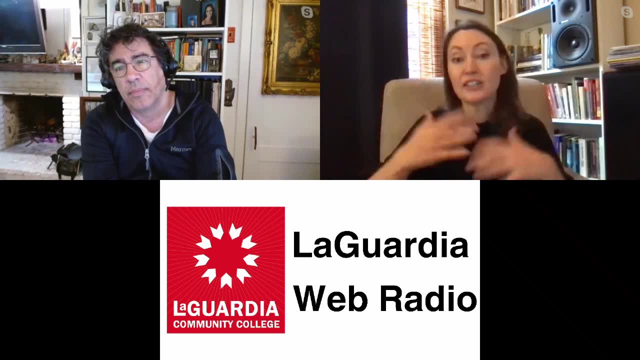 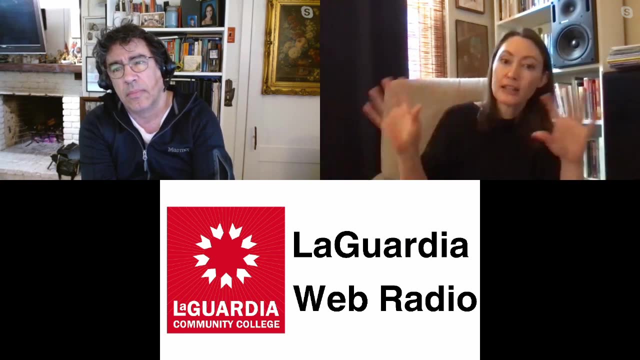 academic programs. some aren't. All over the world- Singapore, Japan, Italy, Canada, Mexico, Brazil, um- every place You can imagine, they've got philosophy for children there. Um, and a lot of these places have different models for philosophy for children, right? What does it actually look like to do it? 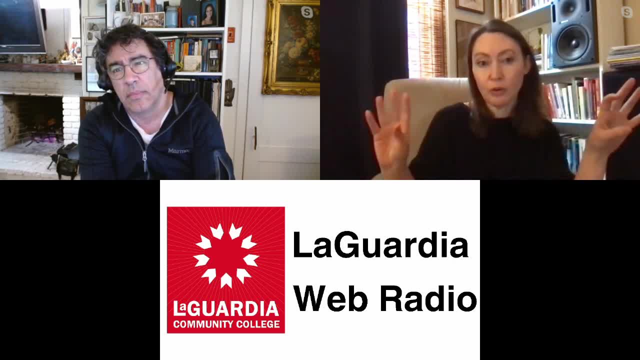 But a lot of them have in common and I can talk to you about a kind of structure for what a philosophy for children outreach session looks like. But I'll stop there for a second because I've been talking for a while. Hugo, do you want to ask me any questions about this? 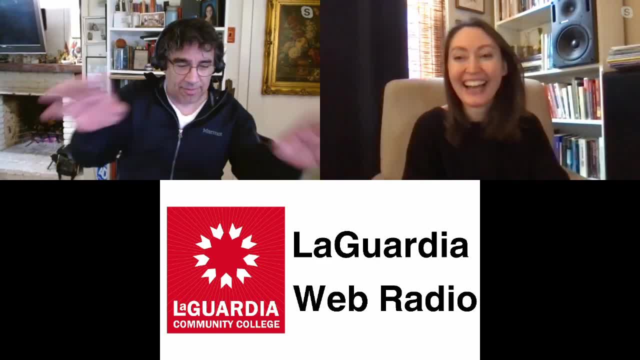 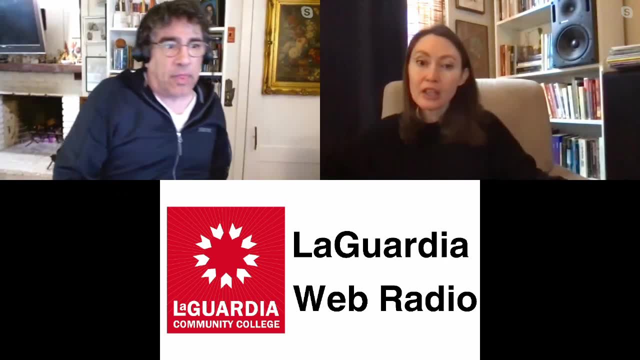 I have, I have a bunch, I have a bunch, but I was waiting for the, for the, uh, Yeah, yeah. I'll give an example. It just felt like a natural Yeah, no, no, it's a good, it's good. I mean, one of the things that I was going to have you define. 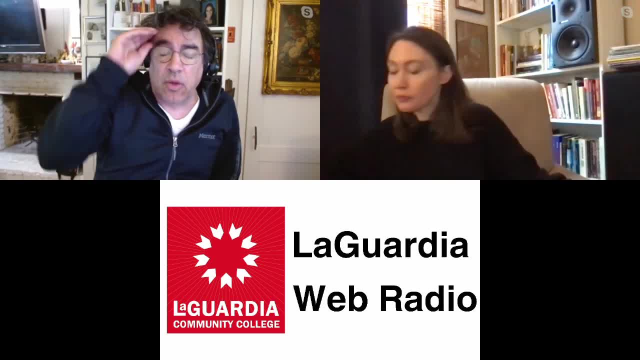 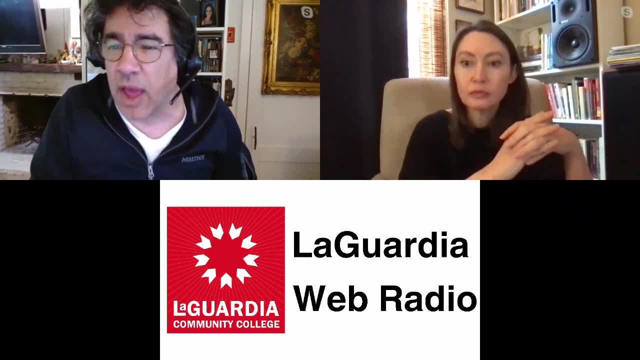 you know, use this term philosophical thinking, So I wanted to find, but you know, one of the things I'm thinking about as you say this is: you know, I've chose, you know, Crosby, Stills and Nash to open the show. Teach Your Children Well, And uh, because you know I'm an old. 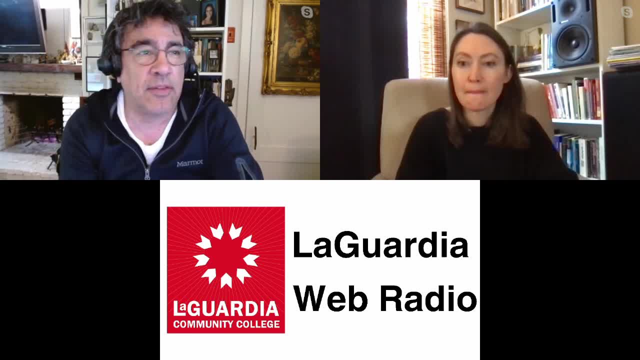 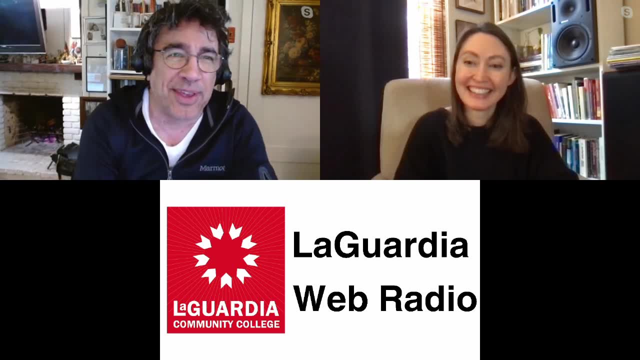 I'm an old hippie or hippie walker. I'm on the tail end of the baby boomers And they're, they're one of my bands. Uh, it's my friend. Peggy likes to say old man, old man music. I love it, But anyhow, uh. 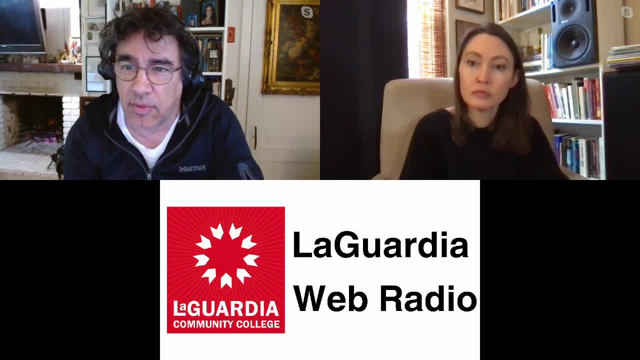 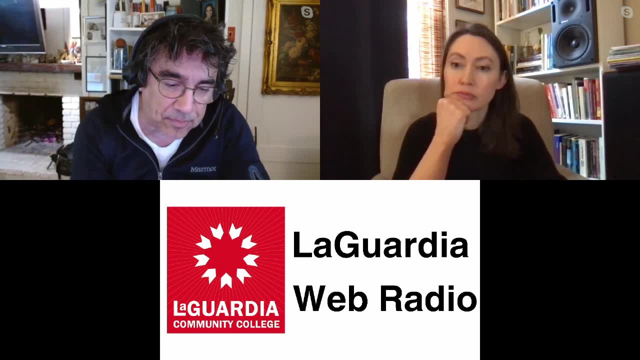 you know that it could have been the other song I could have played- is? you have to be you, you have to be taught. I don't know if you know that song, And so I would think that there are- I mean, you know, there are- parents that are that are questioning what's being taught. 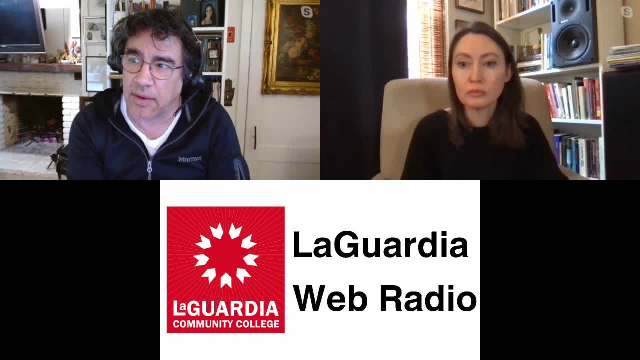 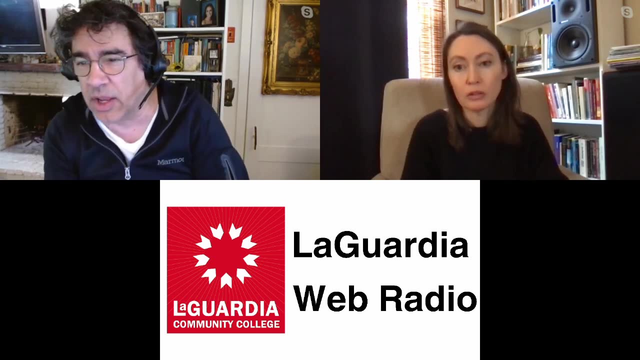 at the college level. So I can't help but think you know cause I? I think of the. there are very different schools of parenting And in one of those schools you are, you are basically told to not ask questions but to do what you're told. uh, children should be seen and not heard. 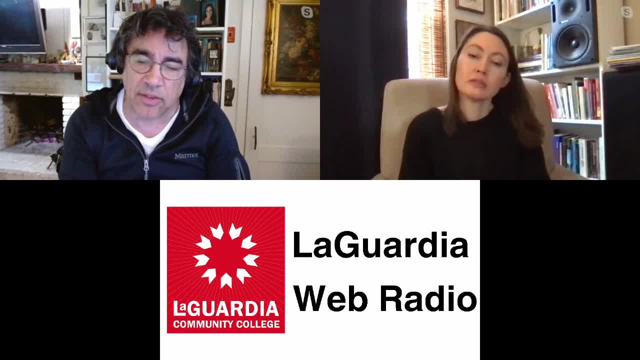 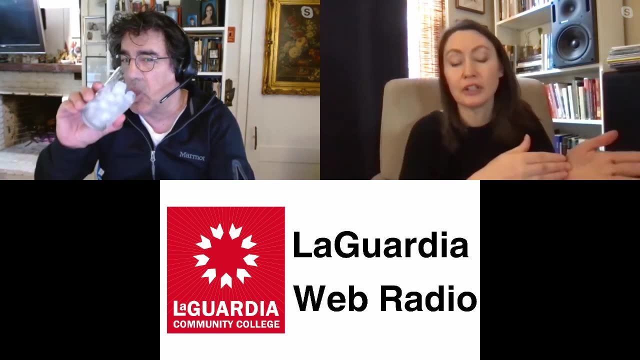 So what are your thoughts about that? Cause I'm I'm guessing that this, you, this, this, this kind of movement has, has found pushback in various, various realms. It's interesting, Um, because I think that I have two thoughts about this. So, first off, that is definitely. 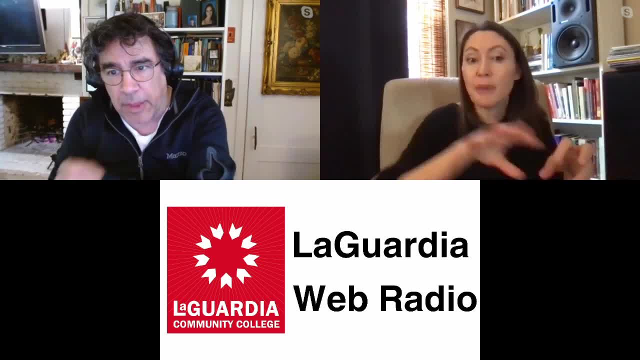 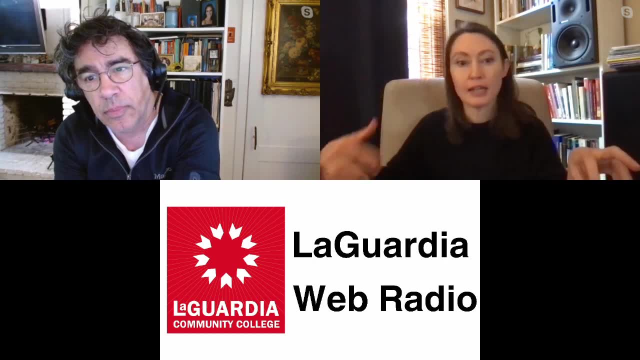 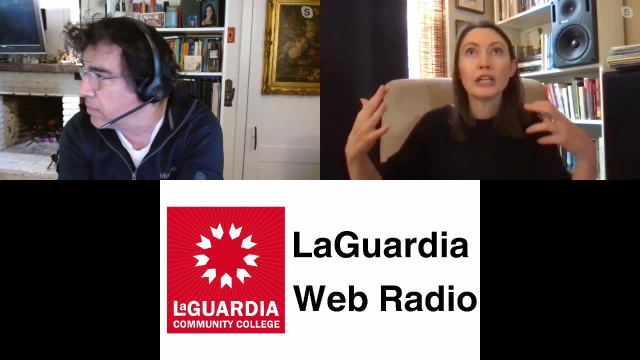 a strain in education, especially education of children, that when Matthew Lippman was developing this model in the 1960s, 1970s, 1980s that he was having to push it back, push back against this kind of um learning, rote, knowledge memorization model of education that had come. 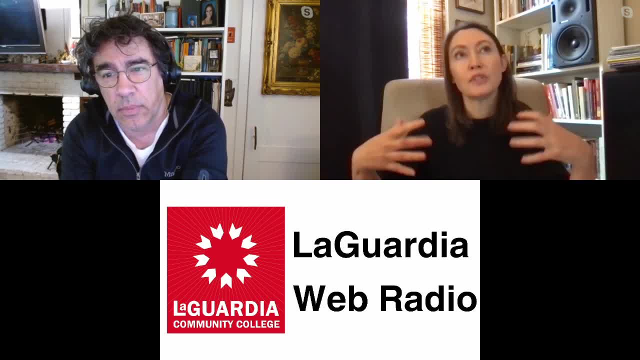 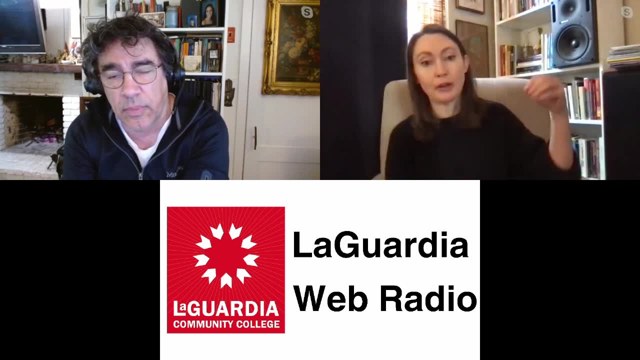 to be so prevalent um in the United States during that time. So he was definitely pushing back and he was really explicit about it. The way in which we're teaching children encourages them to develop a passive relationship to thinking where they're going to be getting. 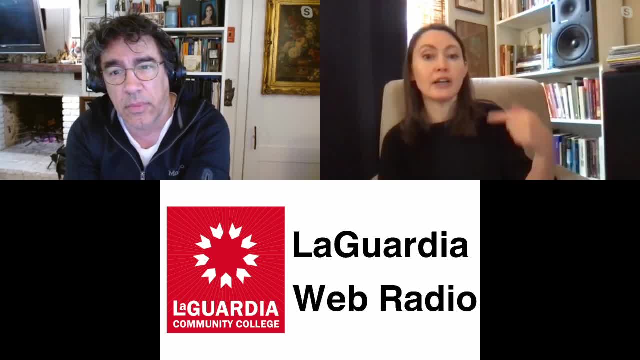 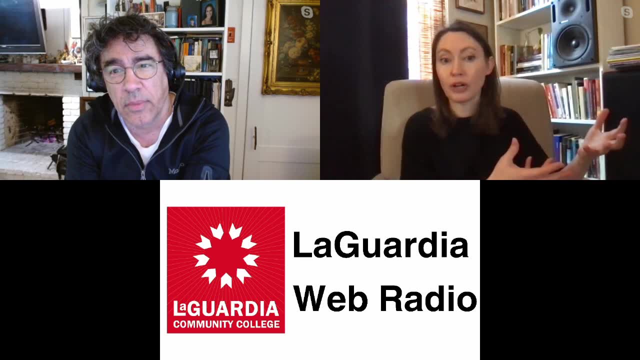 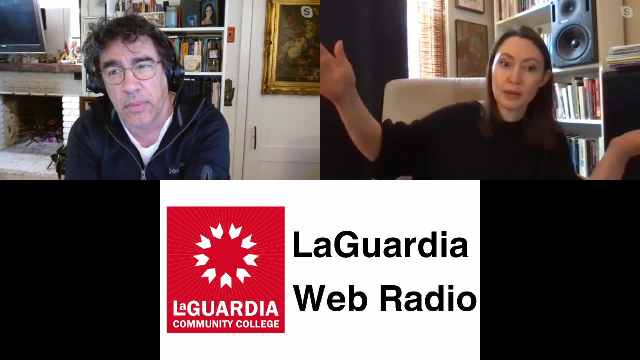 the right answer from somewhere else, And they don't need to develop the skills to figure out what the answer is themselves. They just have to you know, memorize it or look to the correct authority to know what the answer is. And he wanted to say: listen, that's fine for some, for some things, but if we want to train, 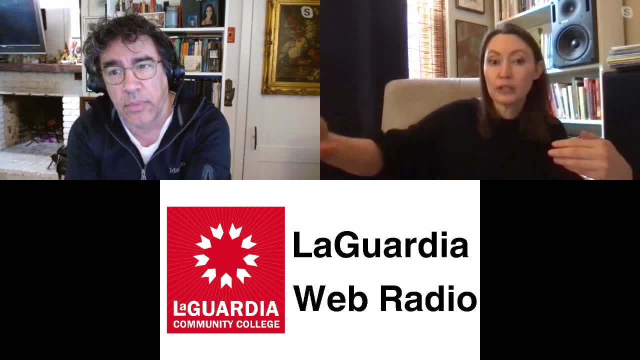 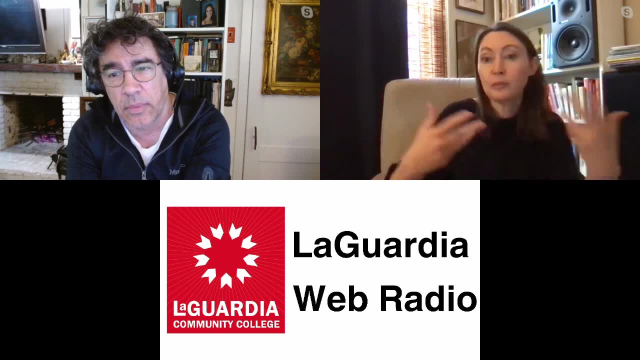 people in the capacity to problem solve and critically think and engage at a high level in this kind of public discourse surrounding things like: should we be part of a war? What should our relationship be with the environment? environment- who should I vote for? right then, we need to train people not just in that kind of 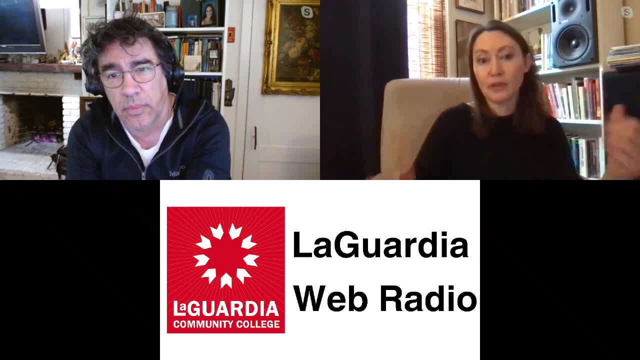 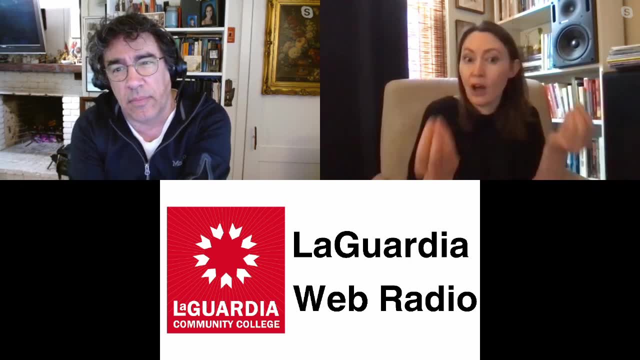 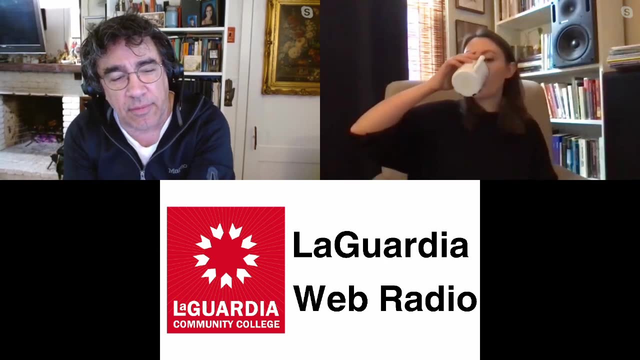 memorization model, but in something that's much more creative and active, which would be more philosophical, or at least so right in on that model of philosophy. go ahead. well, I was going to say so, do you? so you don't think that that there are political consequences? 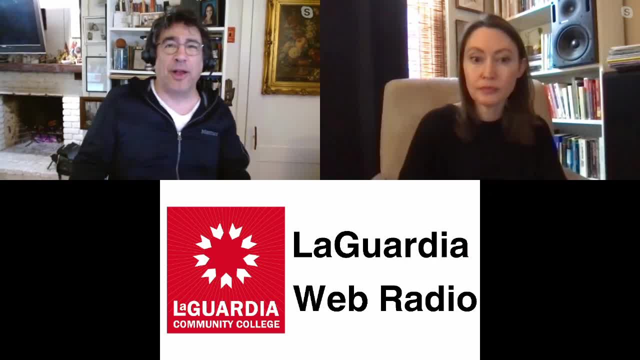 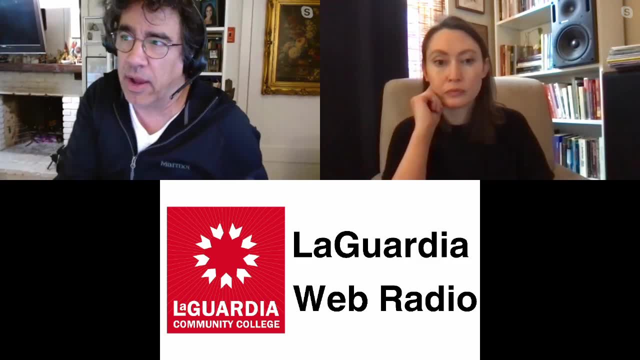 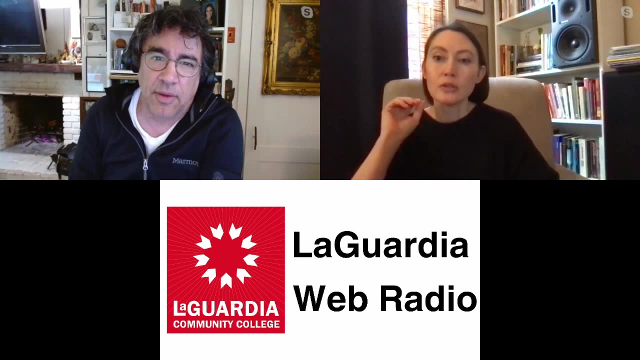 to this approach because I just keep you know, as you talk about this and this notion of deciding who to vote for, there are factions that are trying to encourage you to vote for somebody you know, without questioning yeah, and to just, for whatever reasons, like their vote. it's funny. 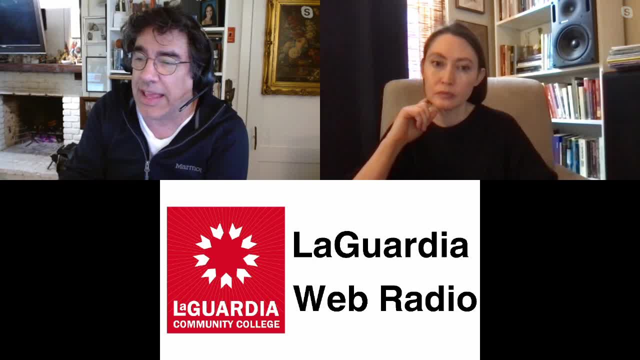 because I've heard two ways about. you know, some people think that it's a lot easier to govern- uh, the educated that actually you want an educated body, They're easier to govern. But then there seems to be this encouragement, at least in the public school level, to undermine education. And you know. 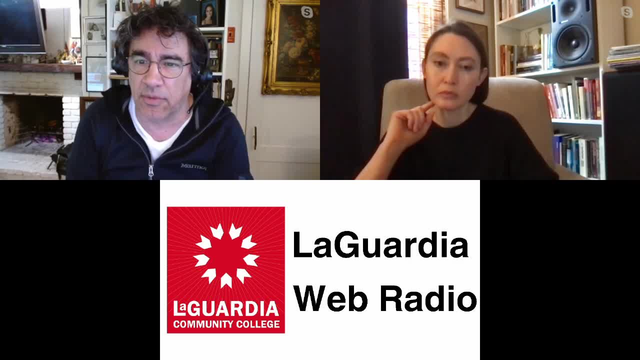 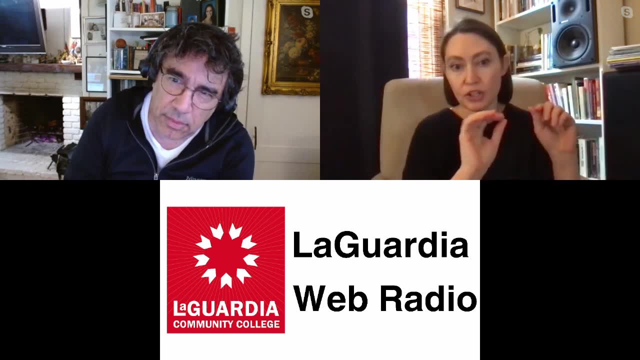 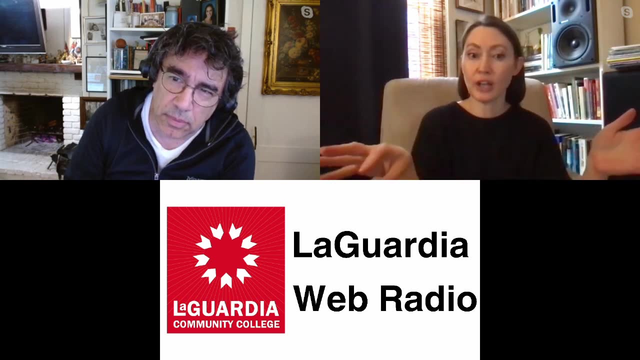 again, people are not capable of making these decisions for themselves. now, Right. So I think I want to actually touch on the second thing that I was going to say, which is I do think that there's been a pretty broad ranging movement within education to take those. 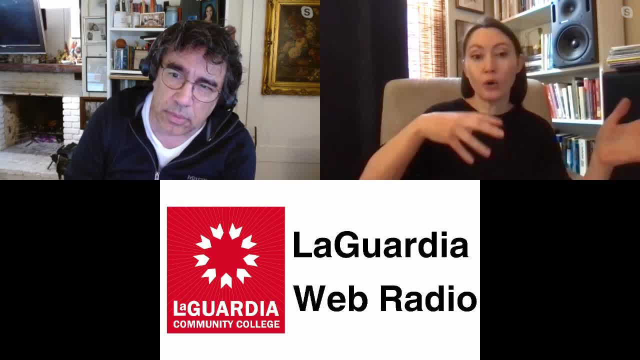 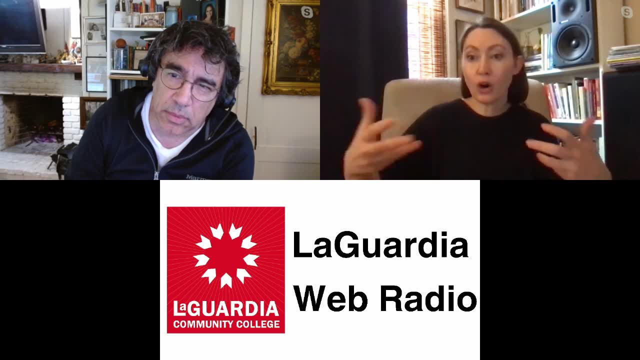 criticisms to heart And so, for example, in my children's school that they go to critical thinking is actively taught, right? I mean they are taught from, I mean their kindergarten and second grade- no third grade at this point- And they are being taught principles of debate, right? 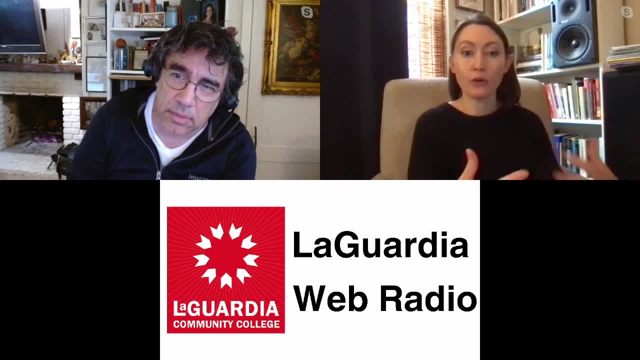 Principles of civil discourse, right. They're being taught how to analyze an argument and how to make an argument themselves. right, Very simple, basic level stuff. But it is a more active model of thinking, not just that kind of rote memorization. And even in their mathematics. 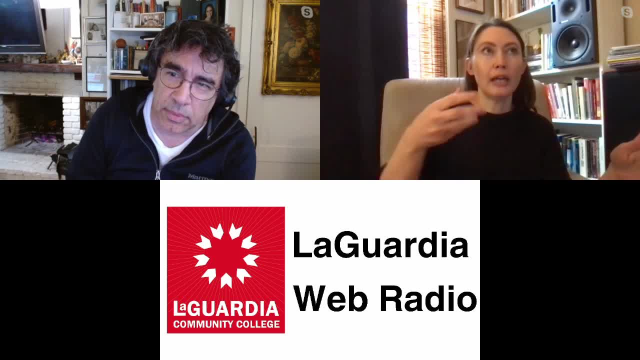 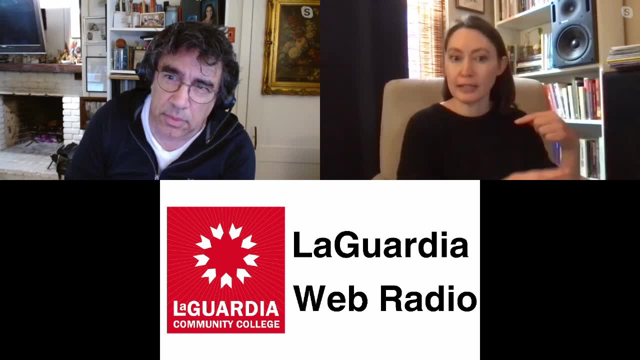 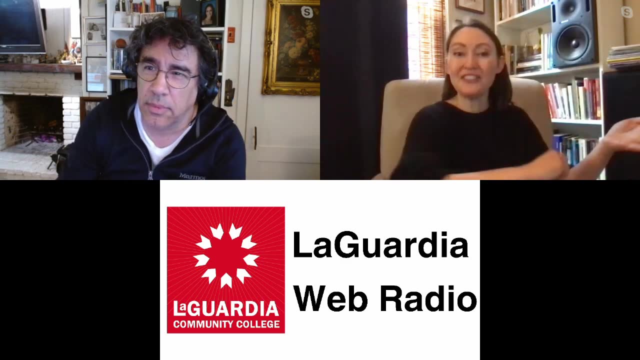 you know they're getting something that's much more embedded in. well, what are the reasons behind this? rather than just I have to repeat the correct answer, And so I do think that it's like, simultaneously a little unfair, to sort of paint all of education. 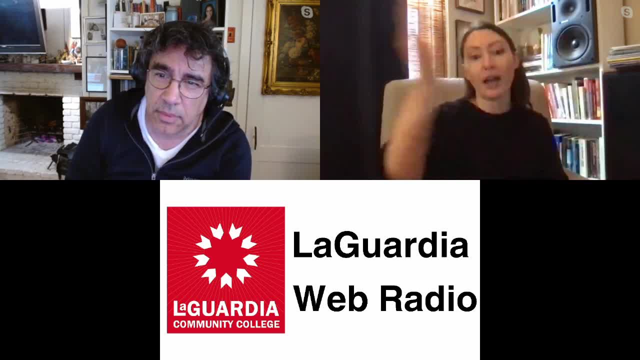 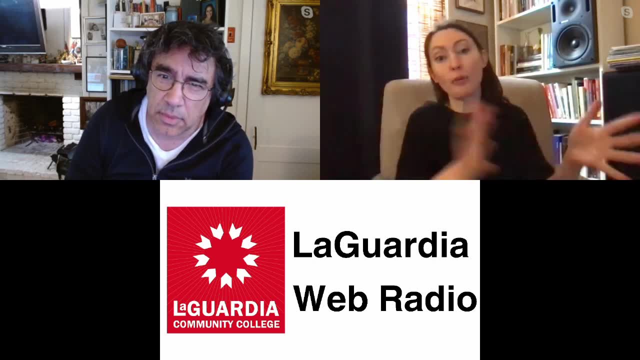 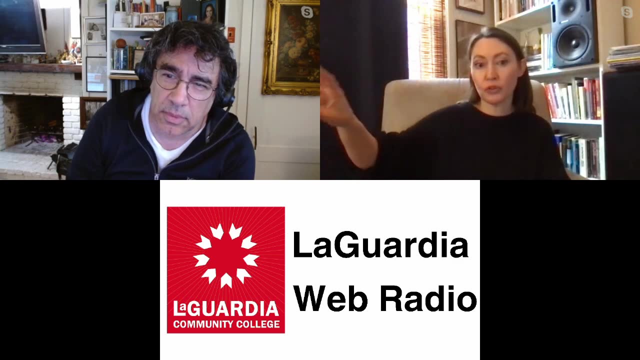 with this broad brush of like. well, you're not, you know, doing students justice by having this kind of rote model, when so much of education really has turned in a different way, And that's one of the reasons why this kind of culture war thing that you're pointing to has become so. 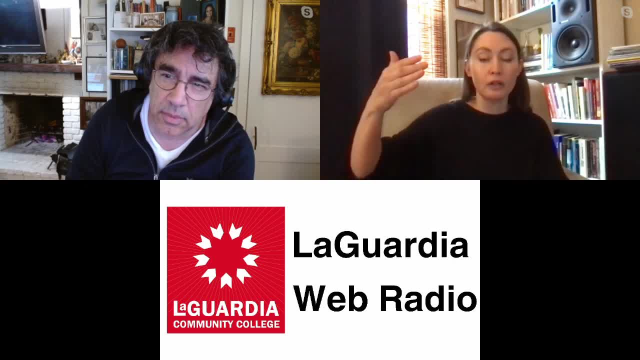 um, such a touch point. Yeah, I think it's a touch point for parents, right, Because they're worried like okay, so if you're teaching critical thinking, like what are you teaching right, And is it something? 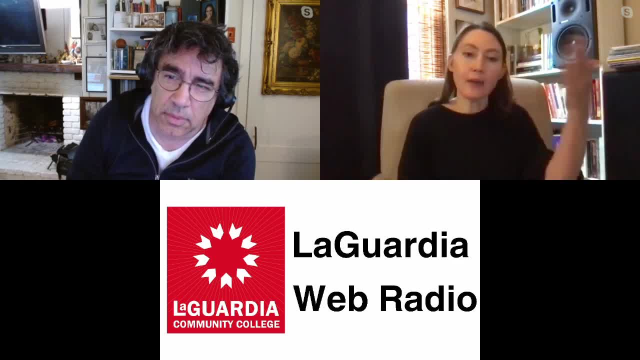 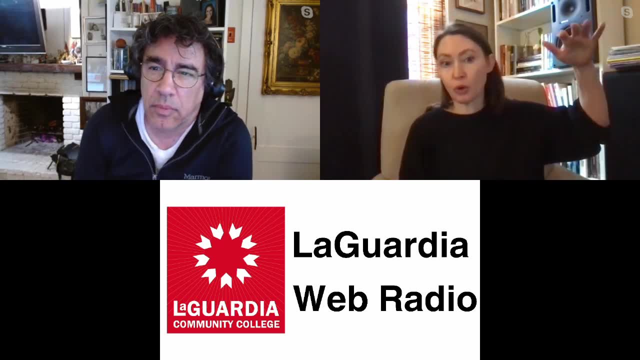 that would align with my values, And it is the case like I'm not one of those people who thinks that that philosophical thinking is somehow like above and more objective than other types of thinking. you know, we come with a set of values, And one of the set of values, one of 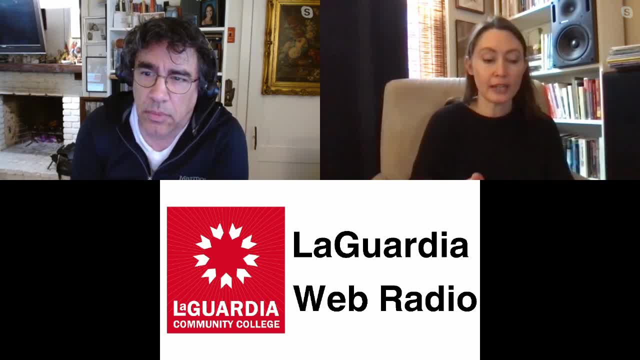 the pieces of value that we that we bring to this conversation is you know we come with a set of values that we bring to this conversation. is we value looking at what it is someone's trying to purport right? What is your conclusion And what are the reasons that you're using to support it? 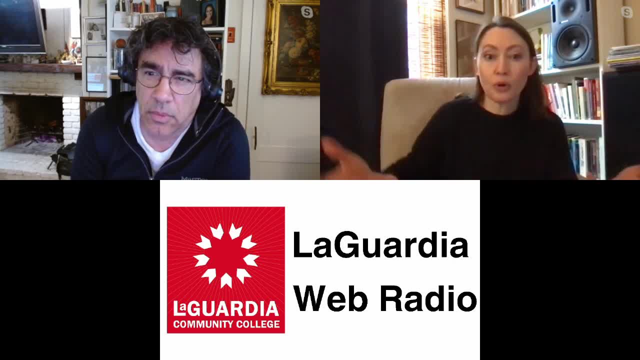 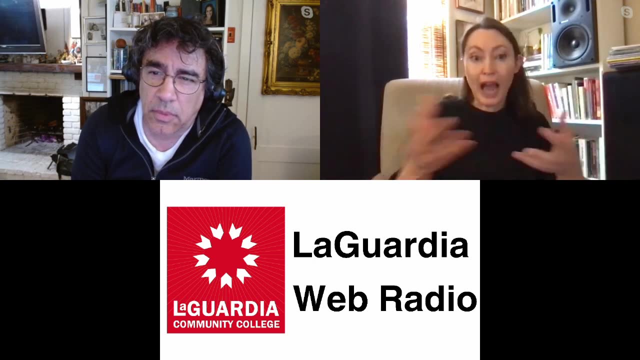 Do those reasons hold water? Do they support the conclusion that you're asking them to support? And that's one of the foundations for being able to have dialogue across differences: we have to agree on something. So let's agree that If we have a difference of conclusion, let's look at why. 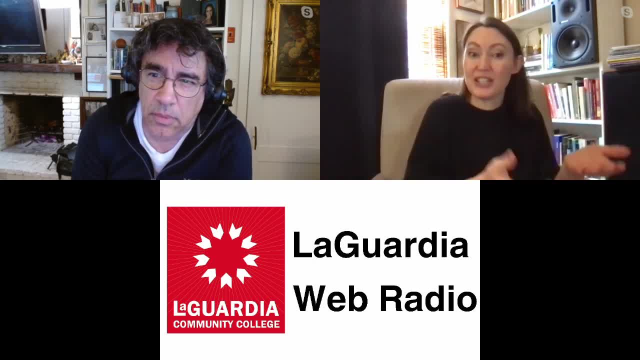 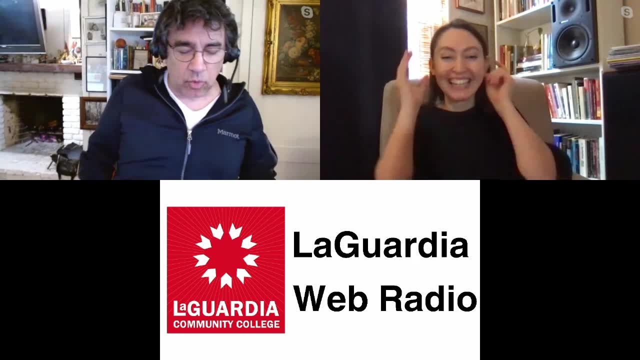 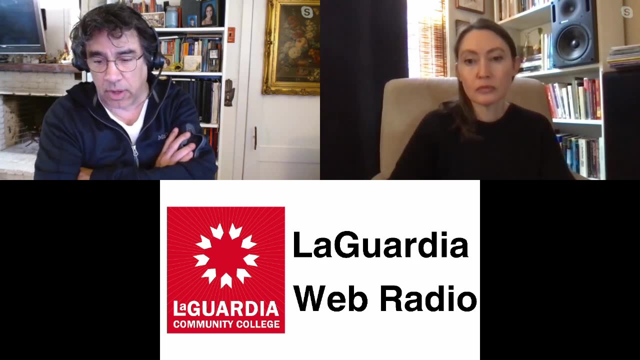 And we have to be able to say like: well, do these reasons that are used to held up these conclusions, are they good ones? That would be helpful. Right, You want to talk a little bit about how your you know this interest for you in philosophy. I guess it's more than interest. 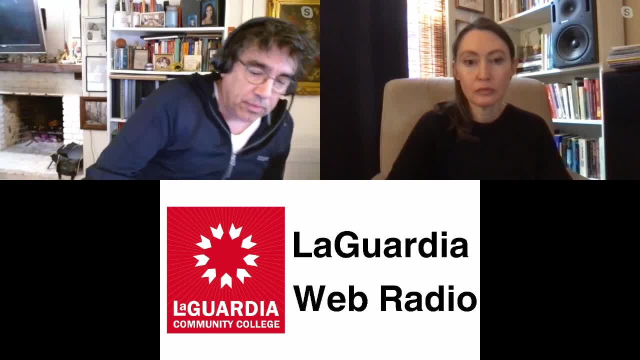 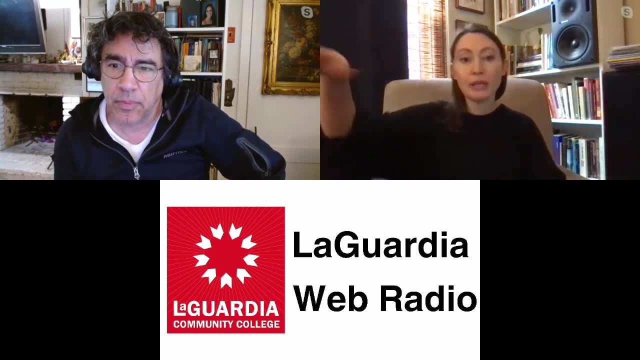 It's your field of study, you know plays out in the work you're doing here at the college. Yeah, absolutely. So let me talk. let me come back to that description of what a philosophy for children session looks like. It looks different. 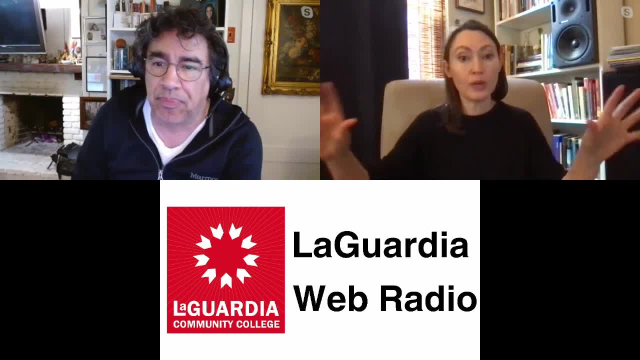 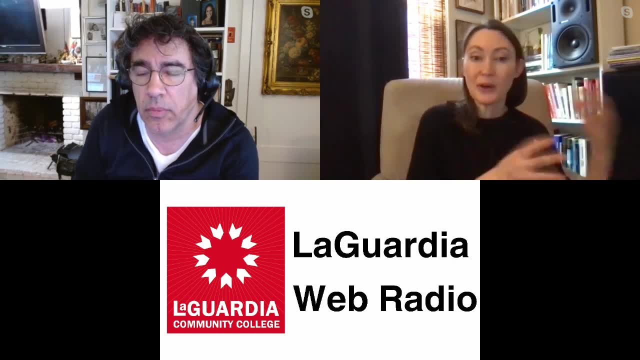 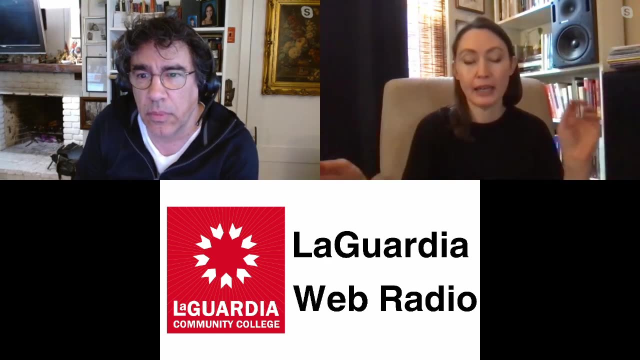 Obviously there's different all over the world. They're doing different types of things that are especially inflected culturally In the United States, right here, so close to New Jersey and Montclair and Matthew Lippman, the model that we tend to take is actually a pretty simple model. 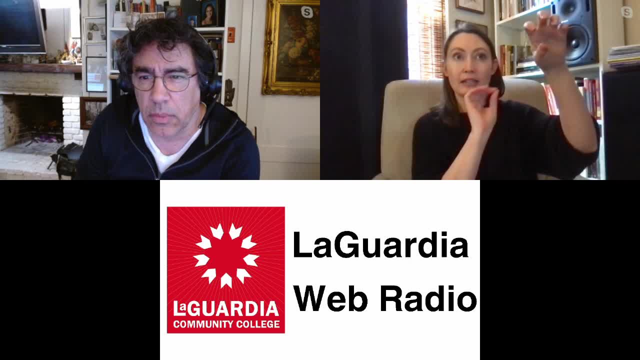 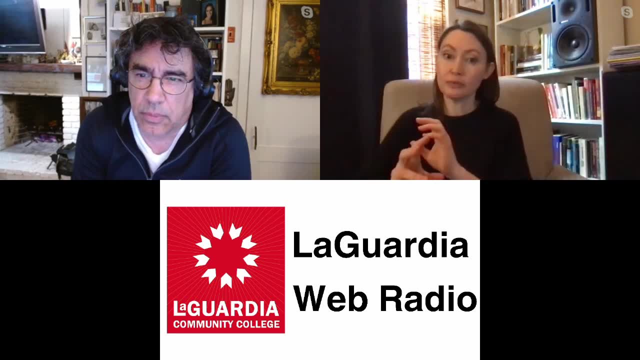 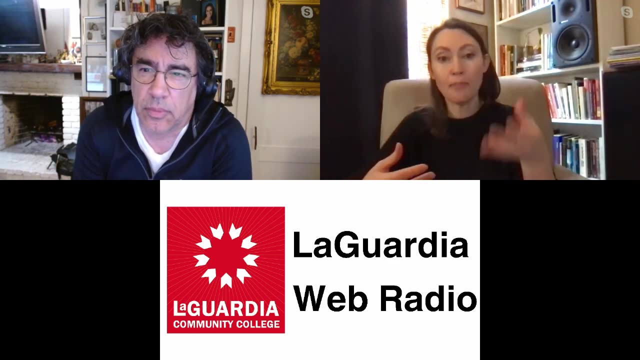 Where you have a problem. You have a prompt, you have a series of questions that are asked, usually by the participants, and then you have a discussion of those questions that's attempting to answer them and engage in a kind of back and forth dialogue about whatever the questions are or some subset of them. 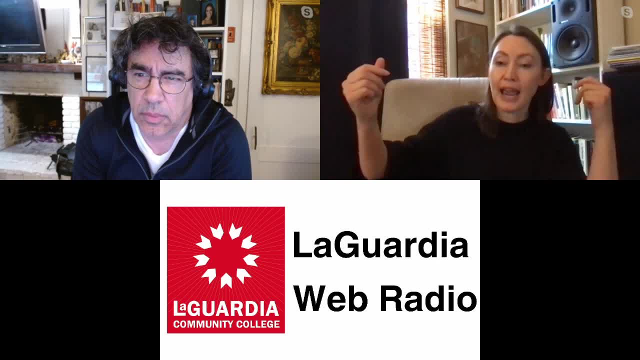 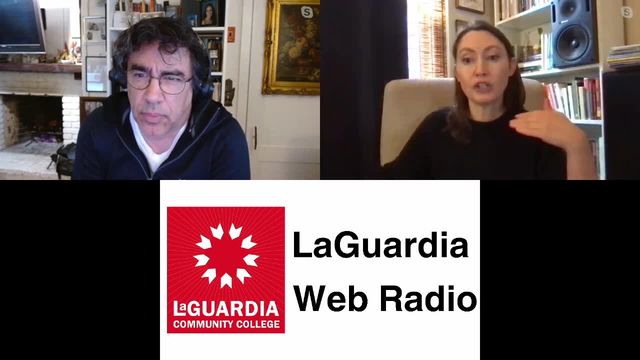 So prompt, questions, dialogue And usually the prompt. not always the case, but for me especially, the prompt is a storybook. So you might choose something usually a little bit below the level of the readers that you're working with. 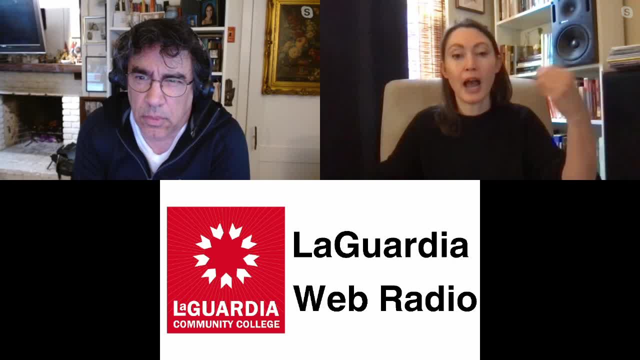 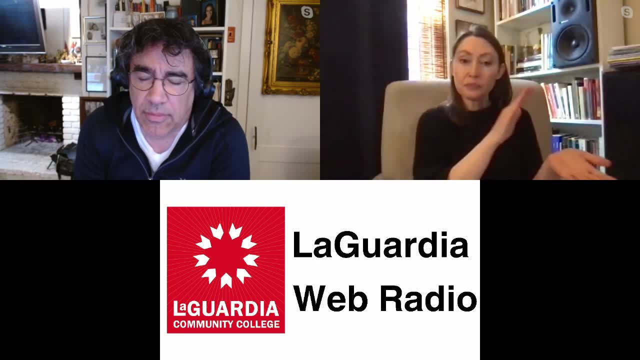 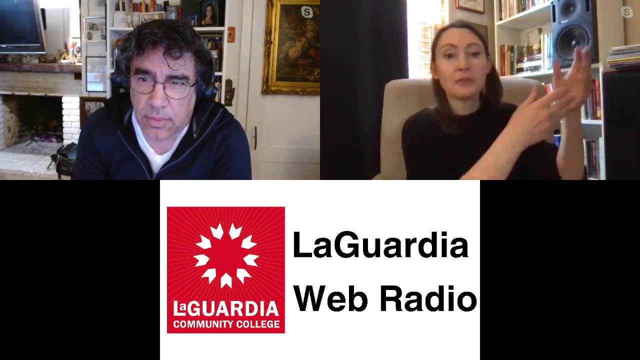 So if I were working with second graders or first graders, I might choose The Giving Tree Famous book. You've probably read it before The Giving Tree. you would read the book out loud to them, Walk them through. We're all crying at the end. 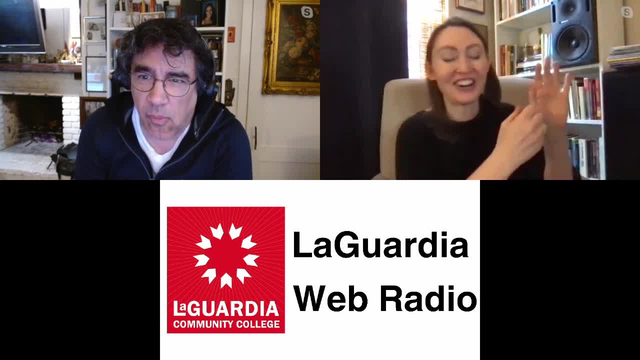 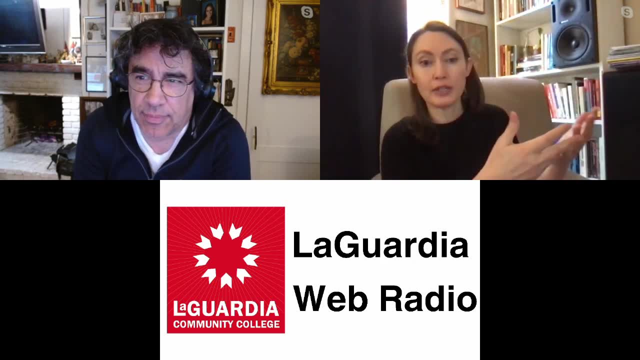 And then hopefully not, but you try to keep yourself from crying. I can't do the Velveteen Rabbit, So you get through The Giving Tree. Then I talk to the students about okay, so what happened in this story. 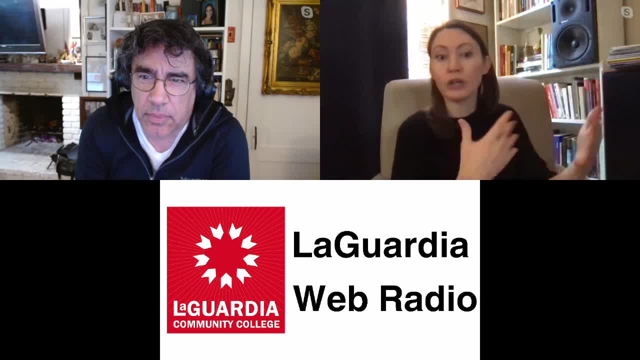 Like what was going on, So that we get a sense of like, okay, so we agree on the state of affairs And then we talk about the questions that we came up with in thinking about this story, Like, what are our questions? 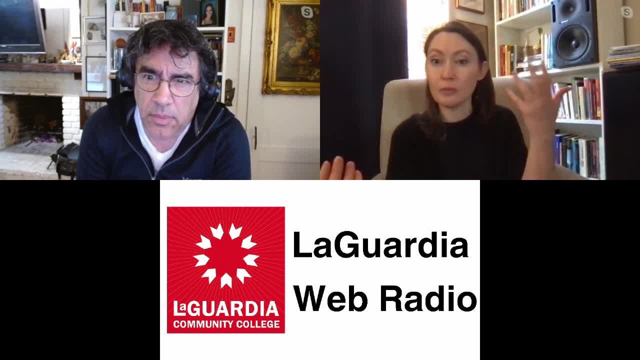 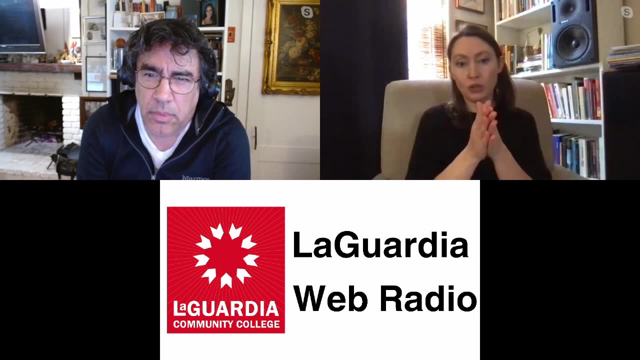 A lot of them are going to be empirical questions that students will come up with where they'll say like, well, why are the apples ripe And not green? But they'll also come up with philosophical questions, And particularly for The Giving Tree they tend to go in a couple of different directions. 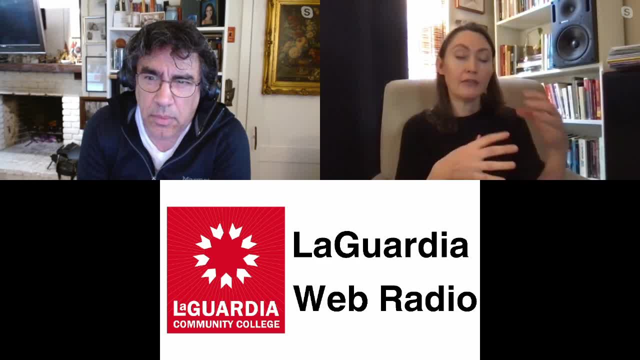 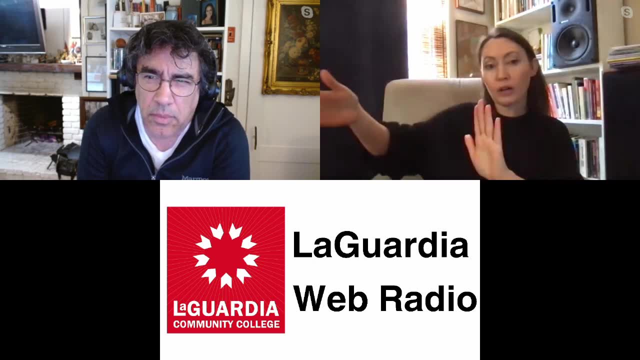 They either are going to be focused on the kind of environmental ethics of the story- So like what is our relationship to the earth and to the trees- Or they're going to go in the kind of familial ethics relationship which is like: okay, so how do we treat our parents? 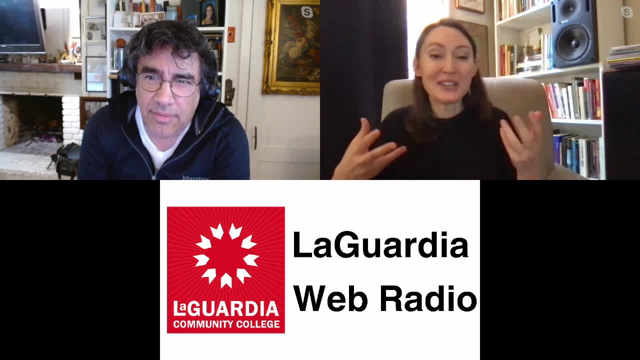 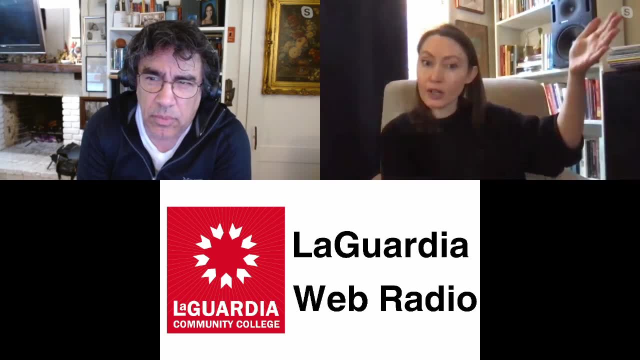 Who give so much to us. What's the right way to do this? And depending on which way they go, then you're like: okay, so let's vote on our questions, Let's decide what we want to focus on, And then you have the discussion. 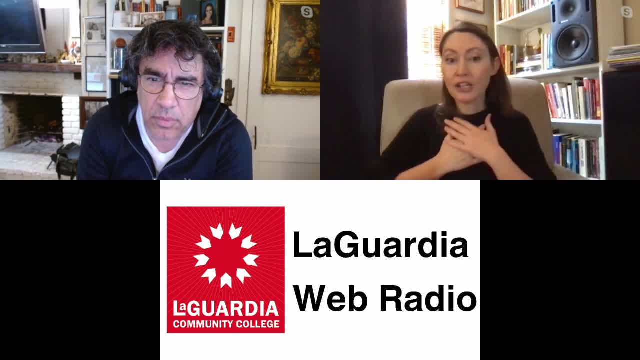 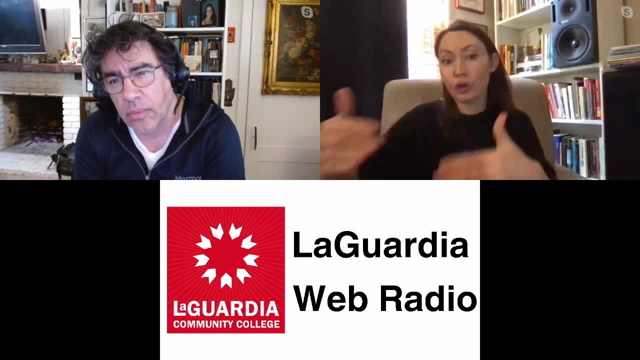 And the facilitator like me. my job isn't to answer the questions for them. My job is to help push their questions in a philosophical direction- if they need to be Okay- And also to then just Facilitate the dialogue. 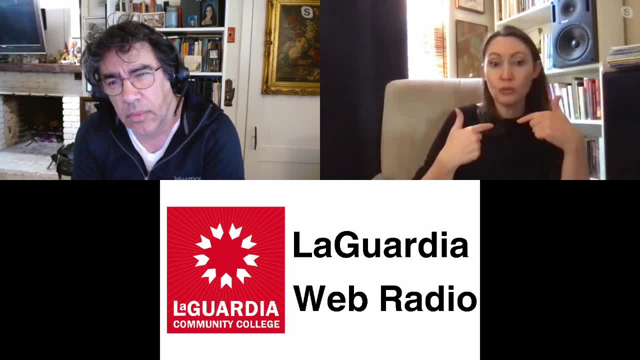 So it's not one student asking a question to me that I answer. It's a student asking a question and then me saying, if I need to, what do you think about this? And if somebody answers, say, oh, what do you think about this answer? 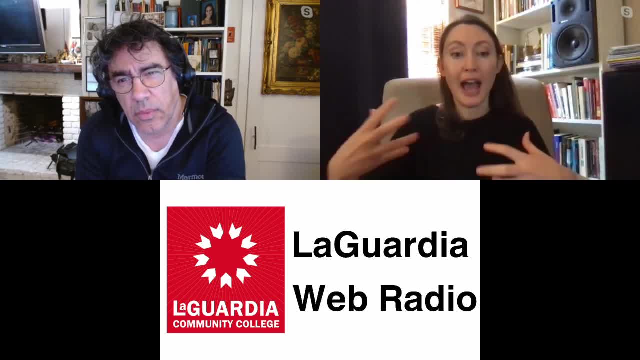 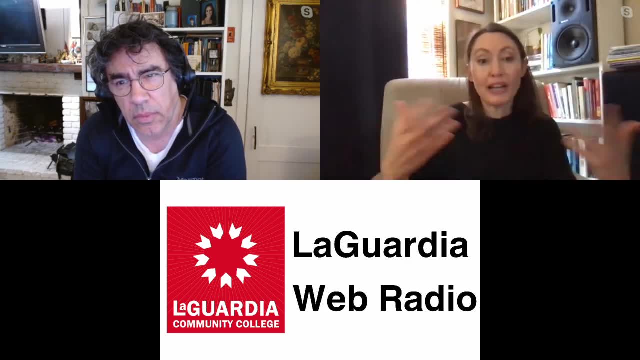 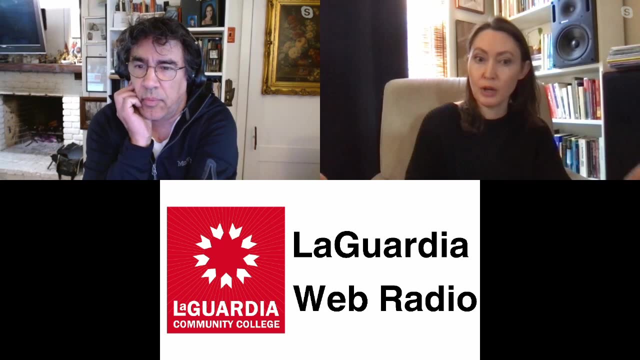 And eventually, through practice, right, they get much better at sort of self-facilitating that discussion. You know I can bring in, Right, It's meant to be, It's meant to be something that is cooperative, right, So I'm part of the discussion but I have to make sure that, given that I'm in a position of power, right. 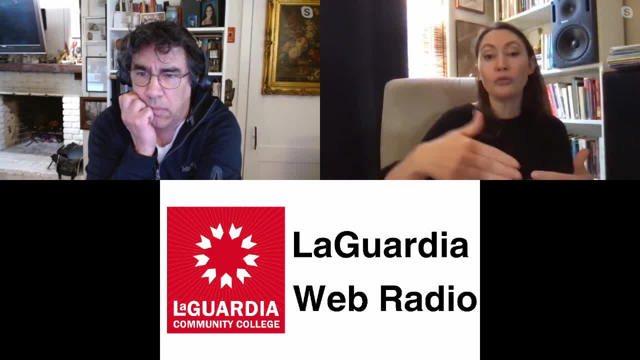 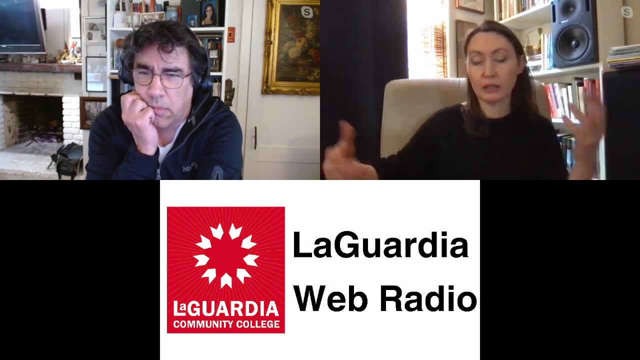 I'm the adult in the room that I'm not overstepping into. hey, I have the answer and you just need to listen to me. That's the. It's that Okay, So, and it sounds like you're using the tools of philosophy. 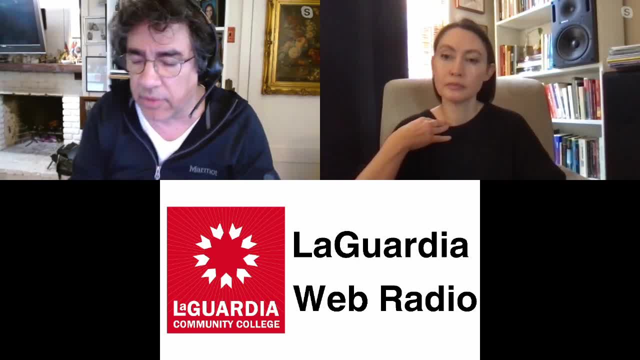 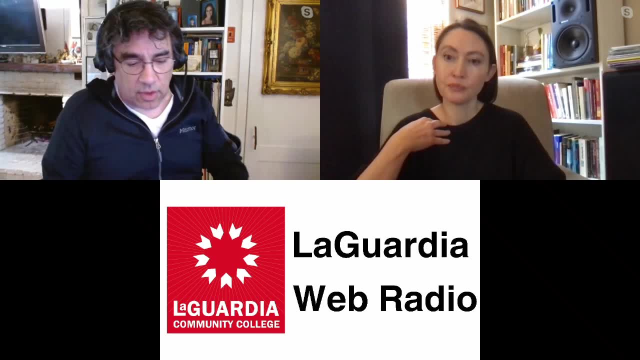 Yeah, You pick, You pick, let's say, a content area like you said, that is a couple of years below their level, to just use as a as the whatever you want to talk about, as the armature to build the whole process around. 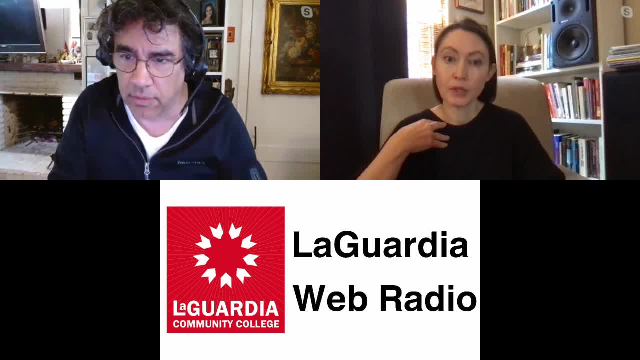 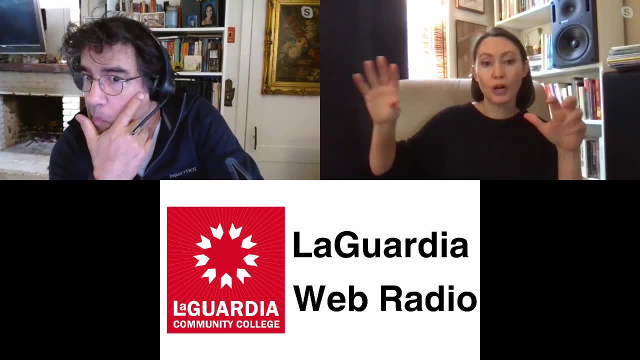 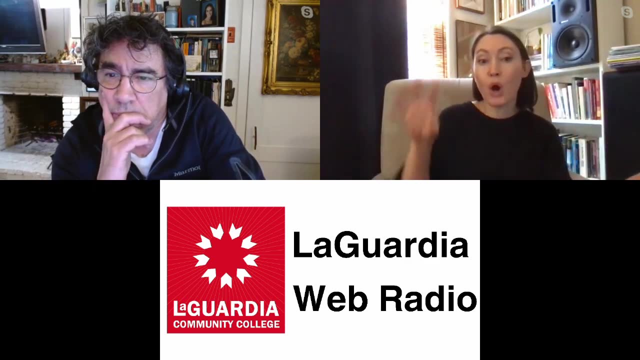 And you can- and this is something you're talking about- doing K through 12,, right? So in philosophy for children it's done K through 12.. And usually programs will focus on a particular age. Um, usually you know who they have access to most. philosophy for children: programs focus in fourth through 12th grade, right. 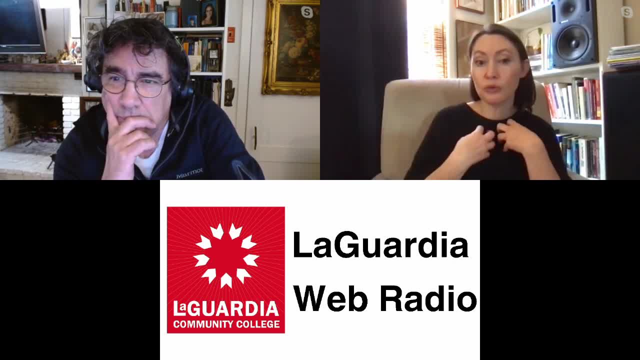 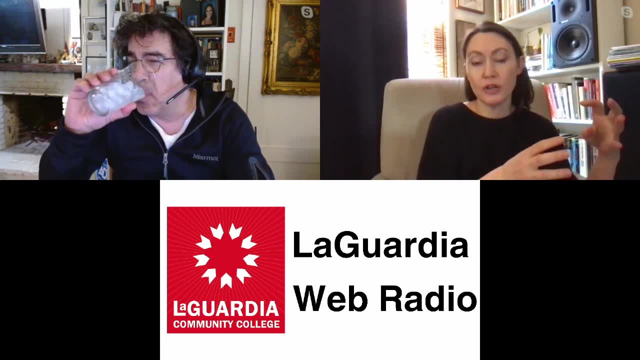 So they tend to focus on older kids. Now, there's two unique things that we do at LaGuardia. One of them is that we focus on those younger children. So I am primarily working. either depends on the semester, but I'm either working with the children. 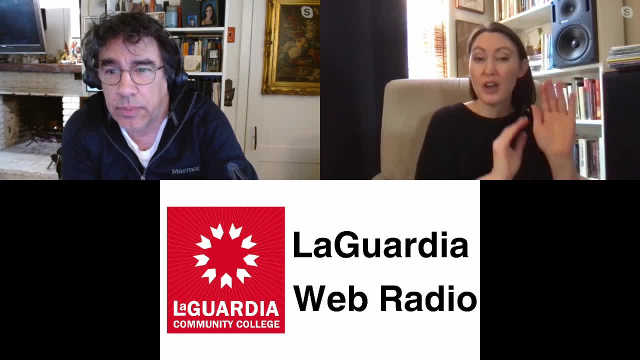 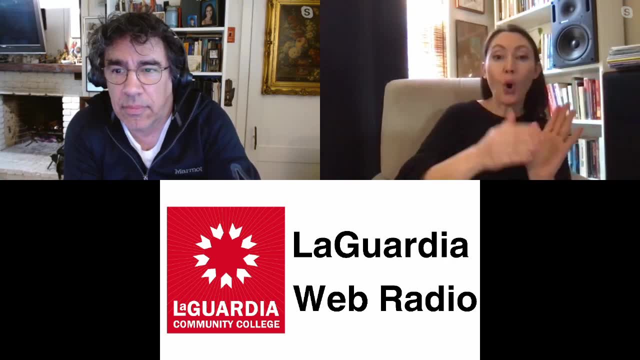 So I'm working with the children in our early childhood learning center, And so we're talking three to five year olds, So pre-K children, um, or if I'm working with the DOE, I'm working with first and second graders. 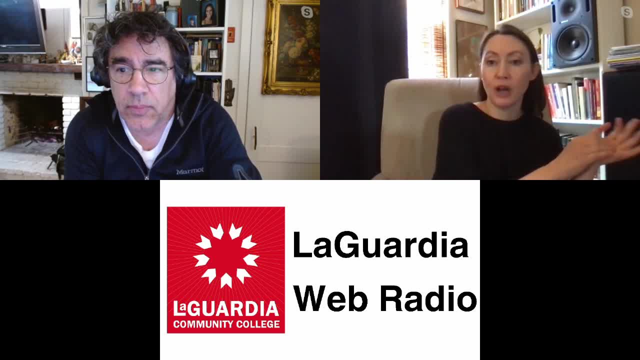 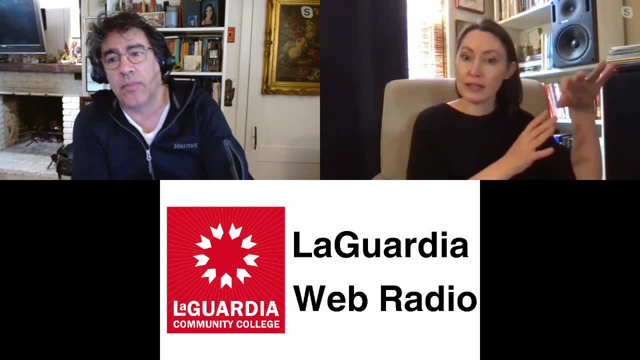 So on the, on the earlier end of where philosophy for children tends to see itself, um, as starting. So that's one of the unique things that we do at LaGuardia. I can talk about the other, But do you want to? you want to ask more about it? 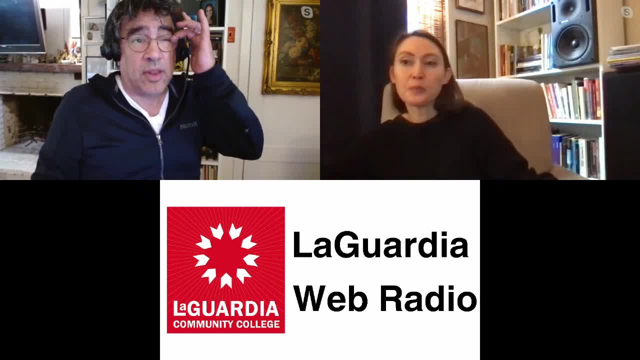 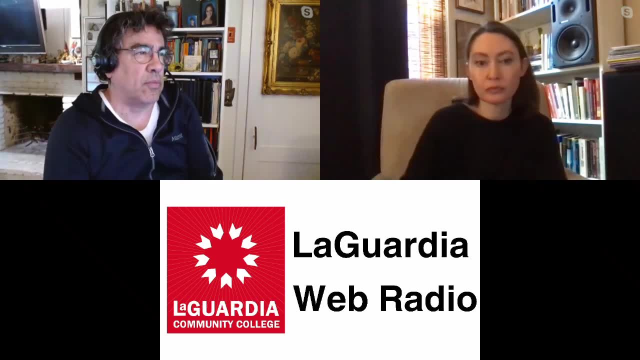 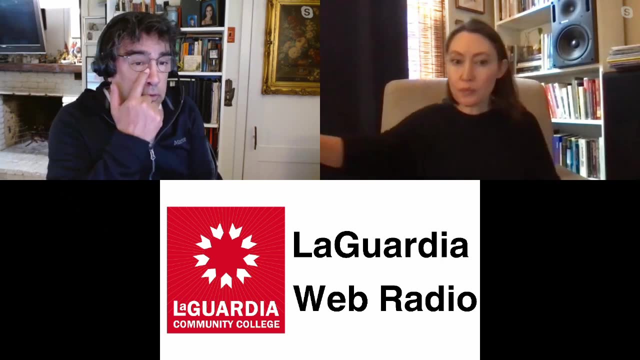 Well, you can and no, I'm just interested because, for example, uh, you and I work together with college now, uh, and and the, probably the, the cohort for humanities. the biggest course for that cohort is critical thinking, uh, which is a course I've never taught. 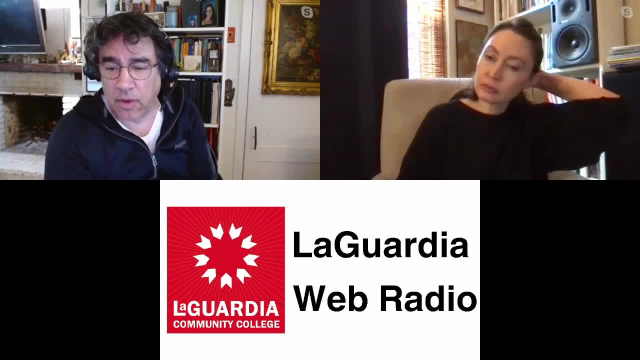 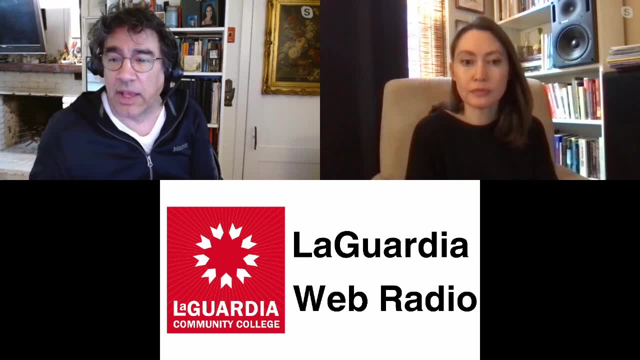 John. John Chafee, the former director of philosophy, had offered me a course and I could never do it And I have always regretted it. And then I, when I started looking at it, I always said to him I wish I had taken this course in college. uh, it would have helped. 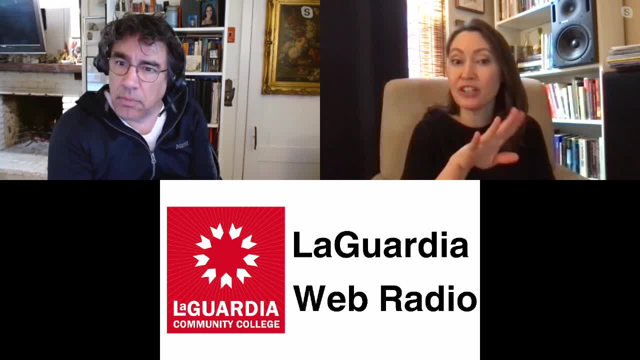 Uh, but in that course, Separate, totally separate issue. Hugo, You and I should talk about photography, because we're we're updating that critical thinking textbook and we need more pictures. Sure, We can always talk about it. Sorry, Go ahead. 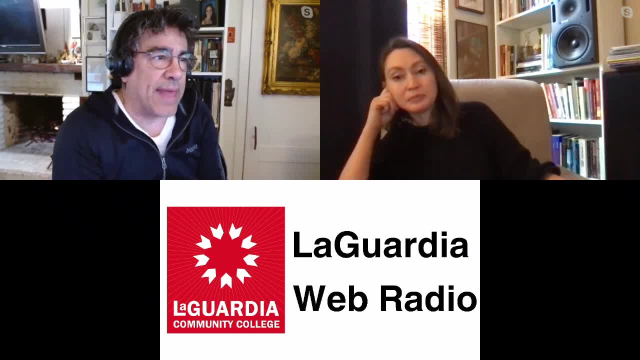 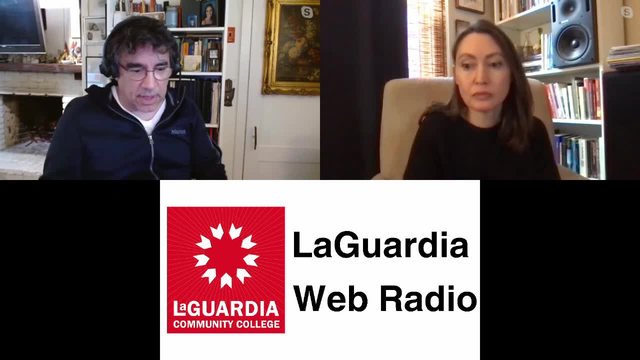 Uh, no, that's, that's fine And uh, but so in that course, I think that the students are in the tell me, if I've kept, I'm, I'm, I'm uh, painting the wrong picture about it. 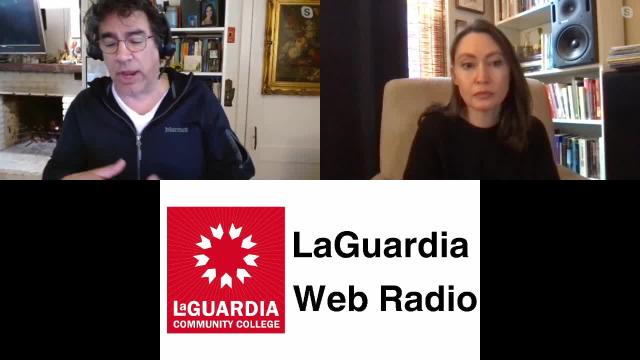 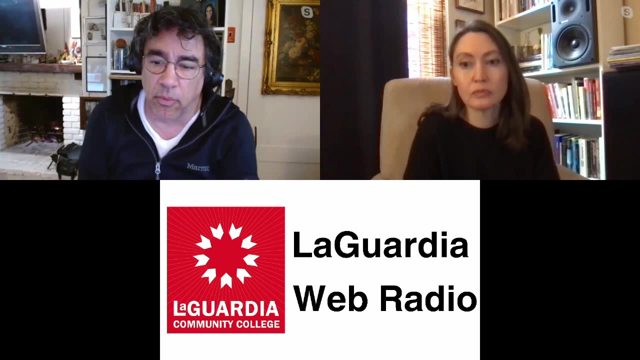 There they are. you are sharing uh approaches to thinking, philosophical thinking, and you do relate it back to some of the folks who were instrumental in the development of these ideas, at least concretizing them. and whatever, whatever it is in text or history historically. 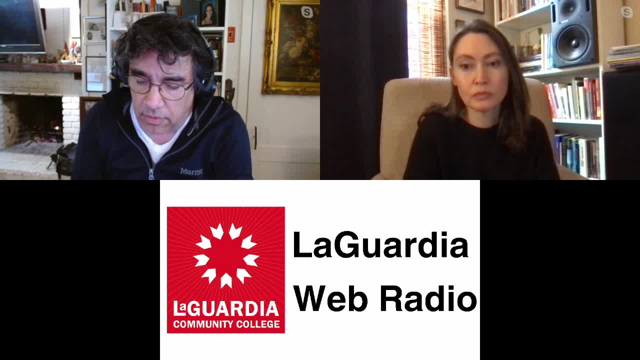 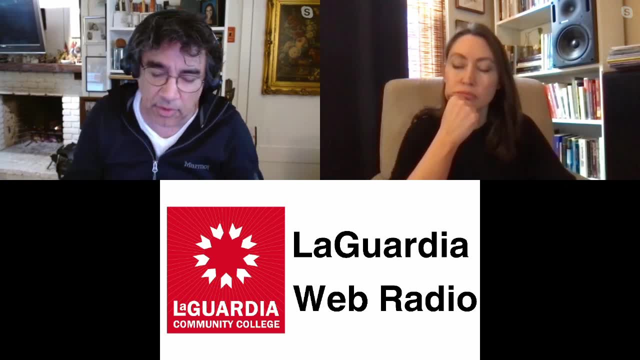 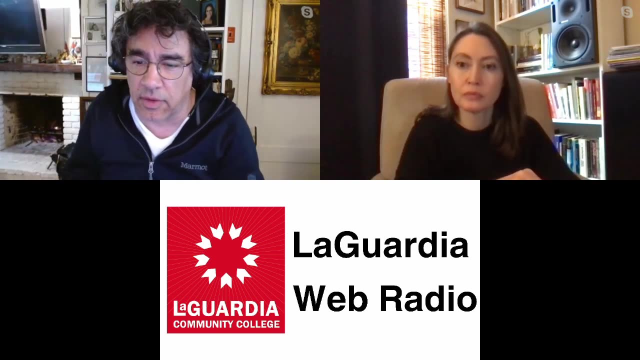 But, uh, but then you, when you move on to study philosophy and the intro to philosophy, uh, we're learning about the history of the, simultaneously the, the players, their thinking and how it played out historically. So it's, it's, you know, when you're saying philosophy for children, again, it goes back to this idea that we're- we're just, we're using the tools of philosophy and the approaches to philosophy, rather than teaching it as a discipline. 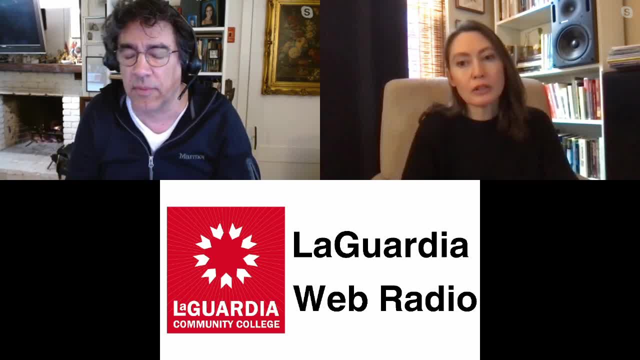 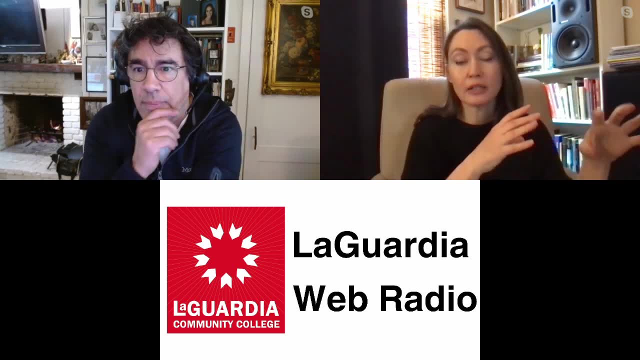 Yeah, Um, Dansham is up in the chat. Okay, For example, if the historical context of all things, So I do there, I have used um, Especially dialogues um from Plato, things like that that are much more accessible. um in translation. 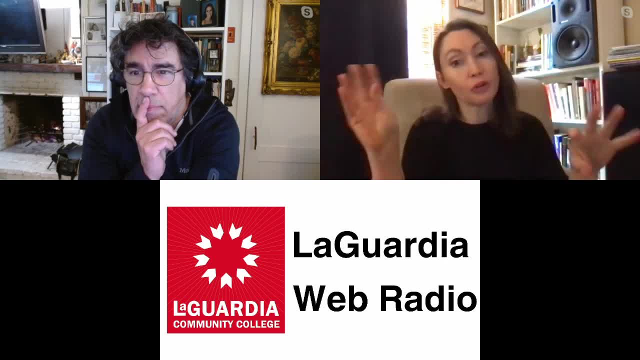 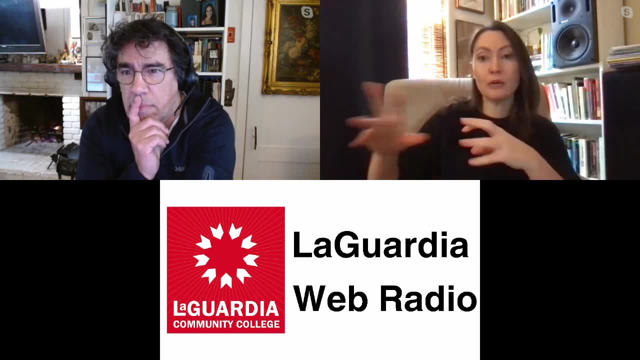 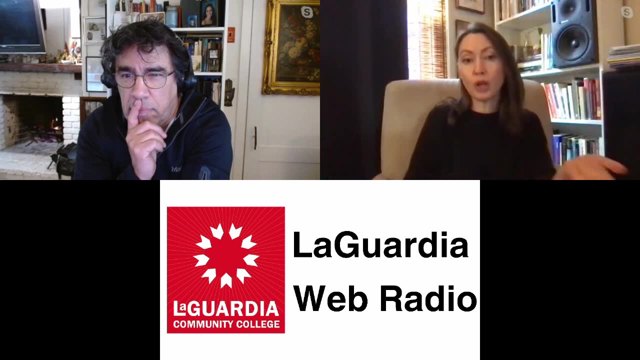 I have used those with older children So, like fourth, fifth, sixth graders and high school students, You certainly can use those texts with, especially if you excerpt them, you know, making it more accessible, focusing on one particular problem rather than a global understanding of the dialogue. So you can. 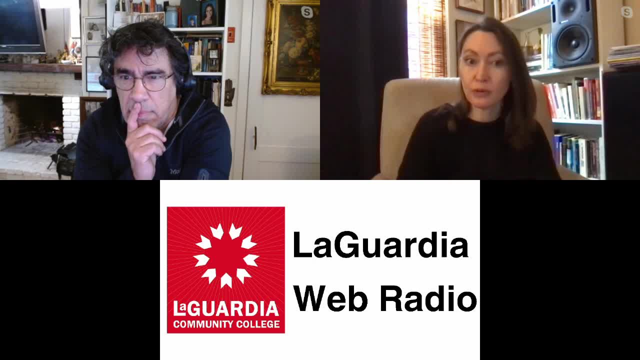 do some work in the history of philosophy with Philosophy for Children students. I have found it to be more powerful and more accessible for these especially younger, younger, younger children to do things that are much more, that are more like picture books. right, They love picture books. 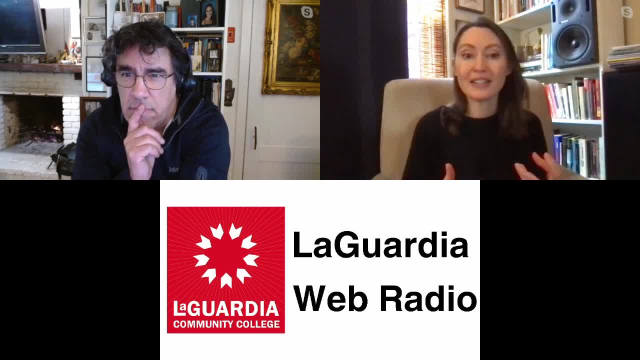 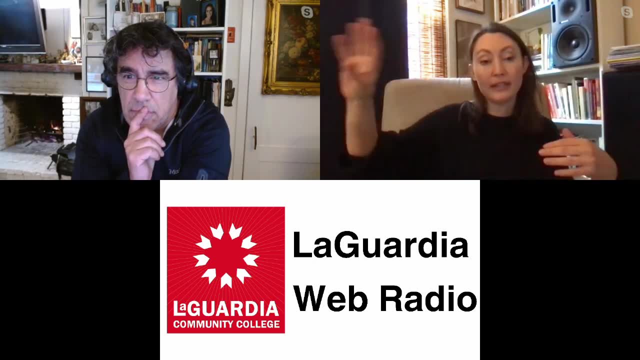 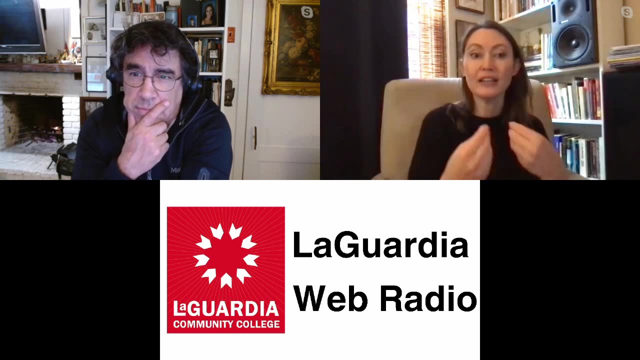 but they also love to play with toys, And so right now I'm doing a philosophy and puppets that I'm doing with the DOE, and we have a picture book, but then we create a puppet and then we use the puppet to engage in dialogue about the philosophical questions that emerge from that. 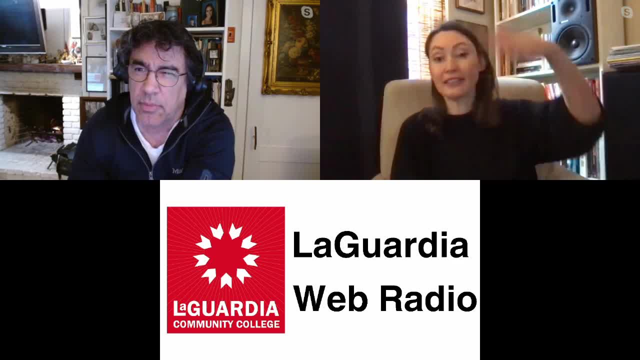 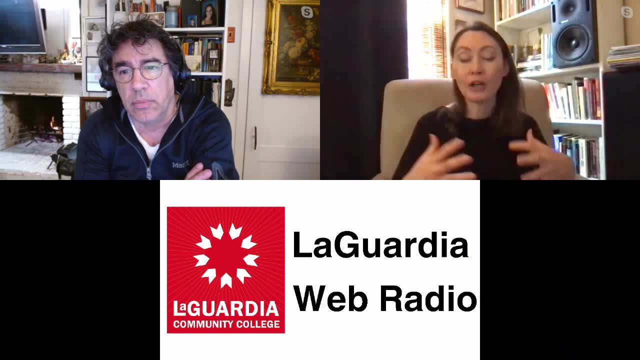 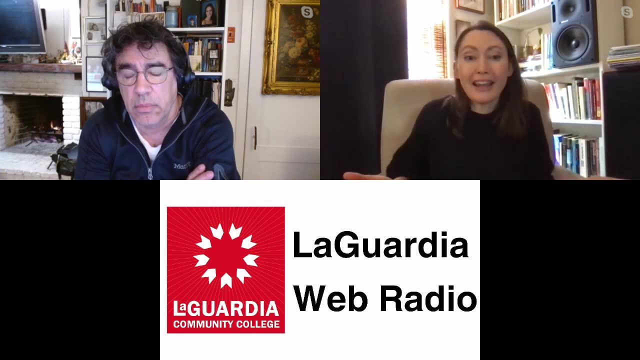 particular book. So we last week, with these students, we read a book called Scribble Stone, and Scribble Stones is all about a rock that wants to express its own individuality. but it's just a rock and it's kind of just sitting there and it doesn't have any way to right express. 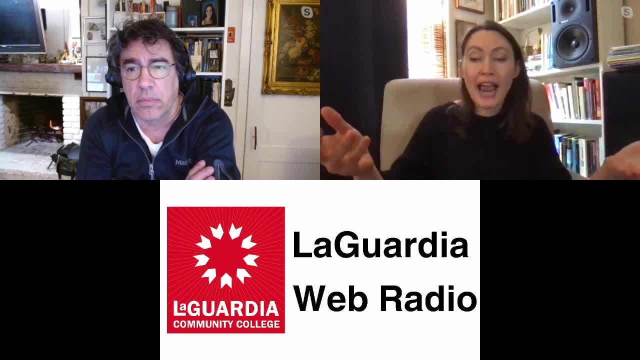 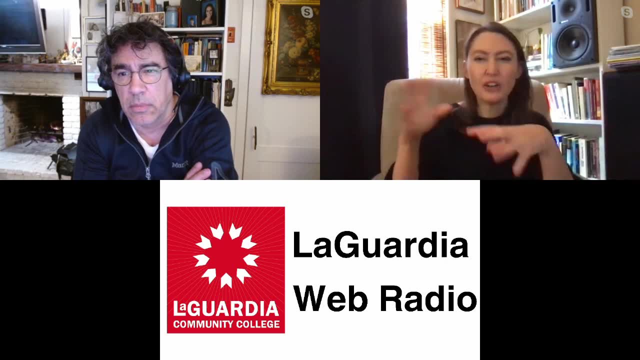 its own individuality. And then it's on a table and it gets paint splotch. It gets a paint splotch on it And over time it gets more paint splotches. It gets kind of messier and messier And as it, 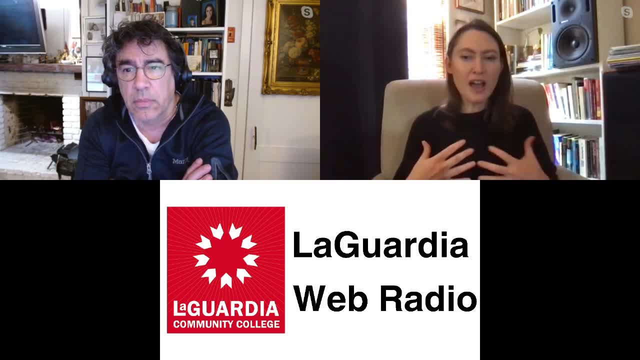 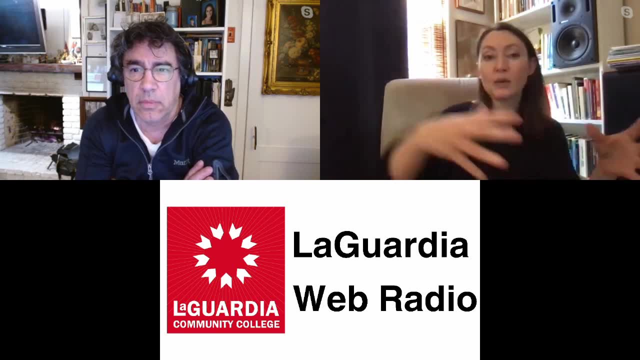 as it gets, messier. it actually is like: oh, this feels good, Like this feels right, Like this is an expression of of who I am and this is creativity, And so it's. and then it goes out and it kind of meets other rocks and they're like: 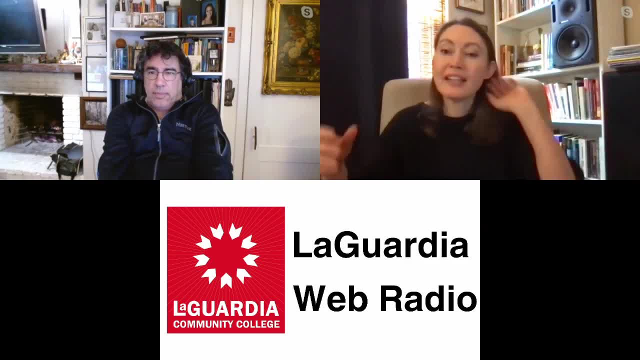 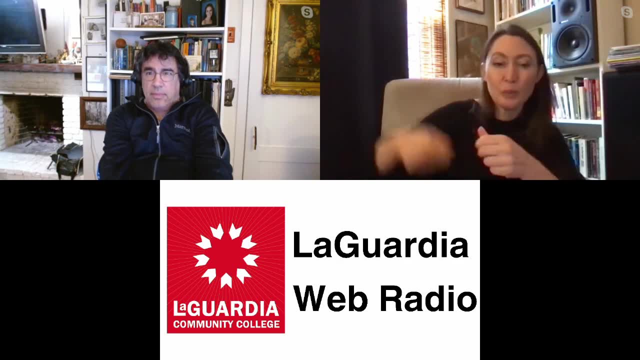 you are very colorful And they're like: yeah, that's the point. And so we make little puppets that are like basically like little pet rocks with little googly eyes. We paint them, put them on sticks, So they're little sticks. I should get one of my rock puppets I can show it. 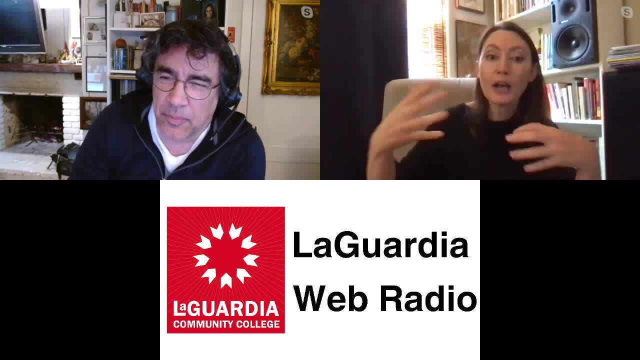 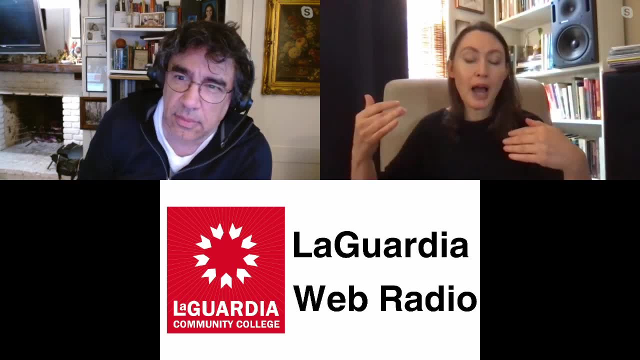 to you, But we make the puppets And then we talk about the, the themes that arose in the book. So we talk about like: well, what is creativity? Who am I? One of the great conversations that we had last week and keep in mind, these are kindergarten. 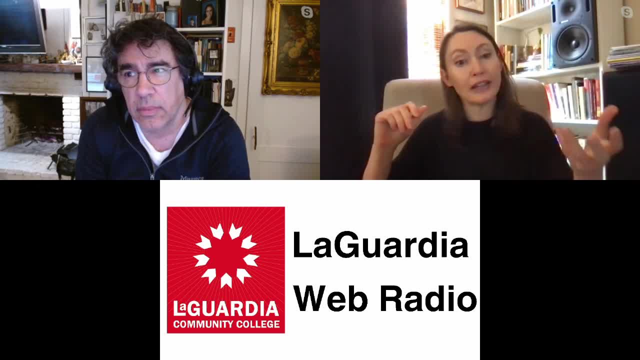 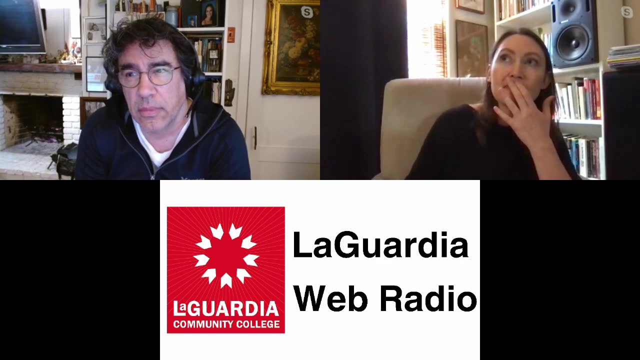 and first graders We talked about feelings, right And so like the feeling of being yourself, also whether rocks have feelings, And one of the one of the children was very, was very clever. She said: I don't have feelings like people have feelings, but maybe rocks have rock feelings. 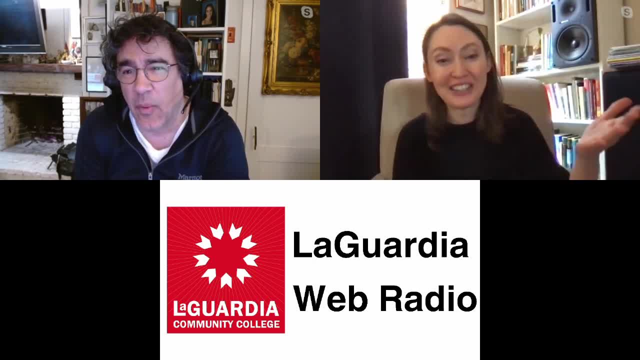 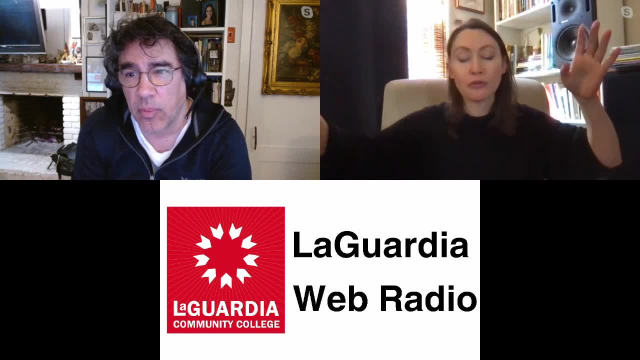 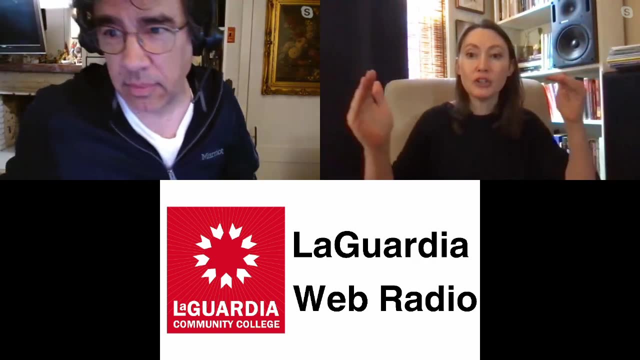 and trees have tree feelings and people have people feelings. But so you see already that even this child is- I think she was one of the first graders- but she's already trying to take a complex concept and break it into different possible components to be able to talk about it. 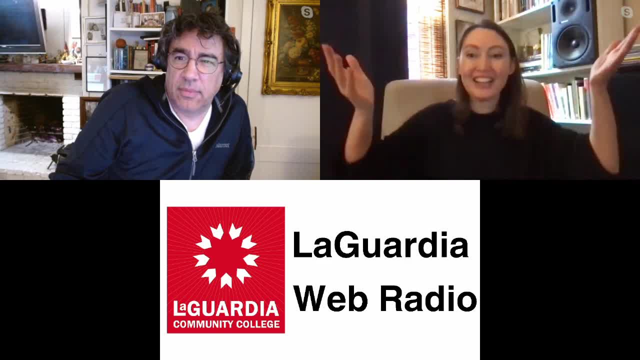 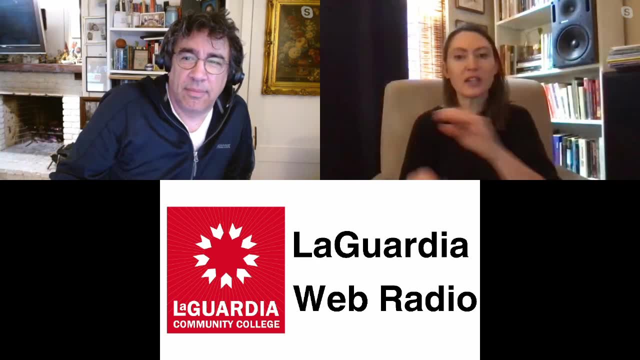 in specificity depending on right, The, the, the thing it's attached to. So not just feelings, but like specific feelings for this thing, feelings for this thing. What do we mean by this? Well, it's much more complex than maybe the surface. 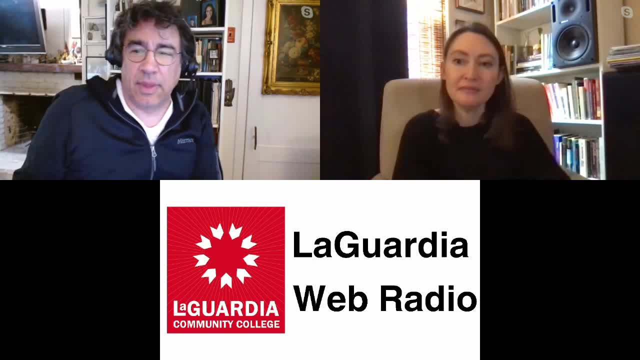 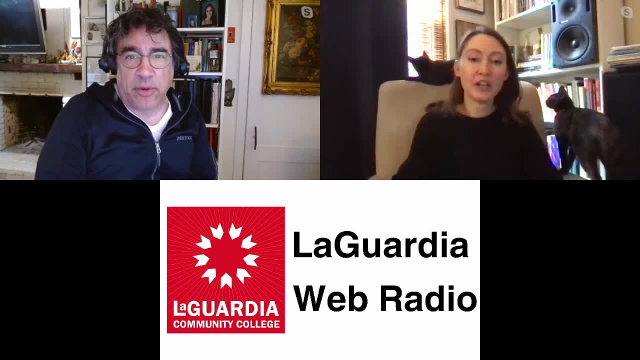 would give us the impression, because it's just one word. Hugo Fernandez, Let me do a quick station break. So the show is What's Going On? I'm your host, Hugo Fernandez, And today my guest is Dr Sherry Carr. 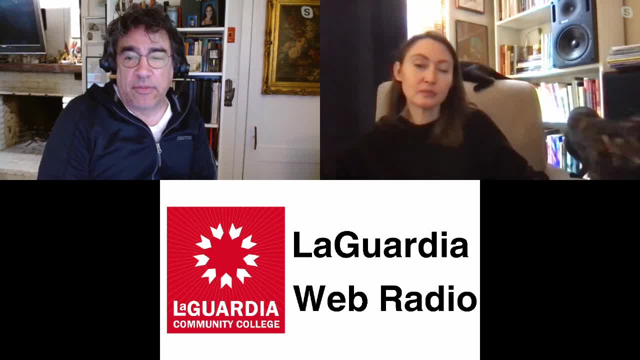 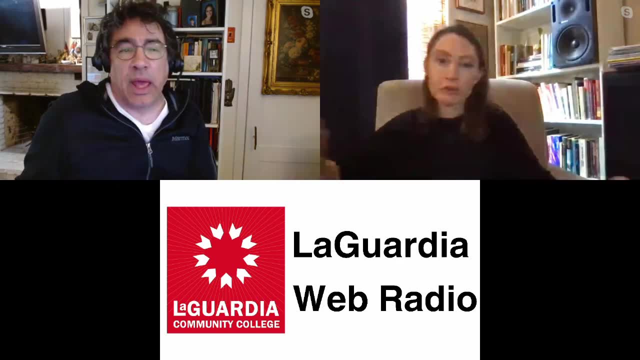 who is the coordinator of the Philosophy Program in the Humanities Department of the Division of Academic Affairs, And Dr Carr is on to discuss her work in the area of philosophy for children, And one of the things that ran through my mind I was kind of doing a reverse thing. where have you heard? have you ever heard? 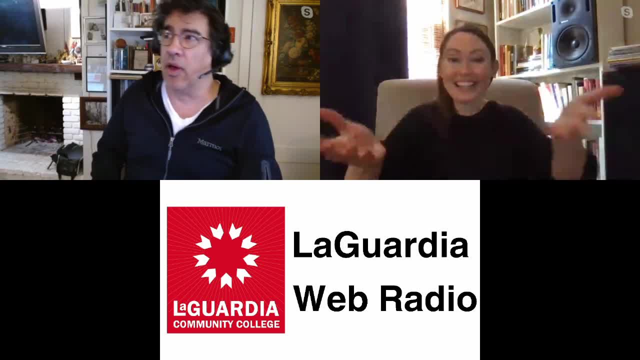 of the book The Tao of Poo. I have. I never read it. Tell me Well. I mean, it's been and I've read parts of it, but I don't have. I'm not an author. I used. 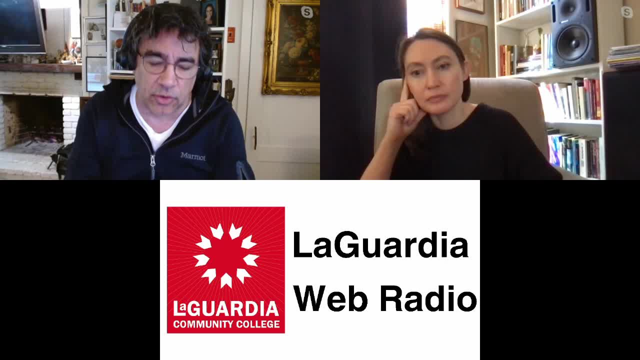 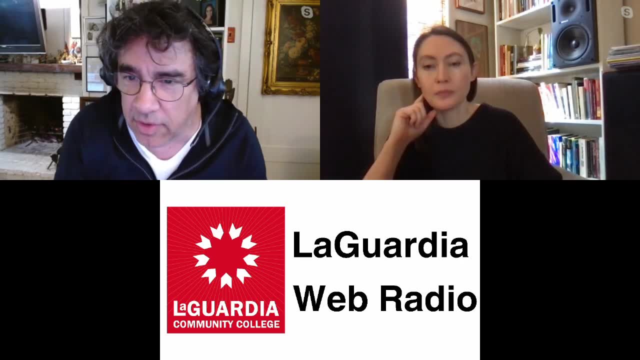 to have friends who keep it in their back pocket. Nice, Oh, that loved it, because there what you're doing is you're taking a children's story and you're extrapolating thinking, or that can be applied as an adult. Yeah. 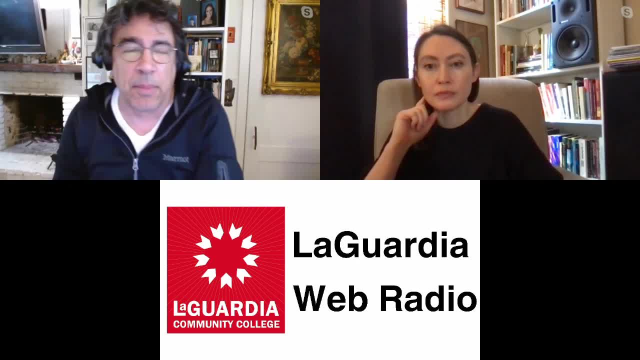 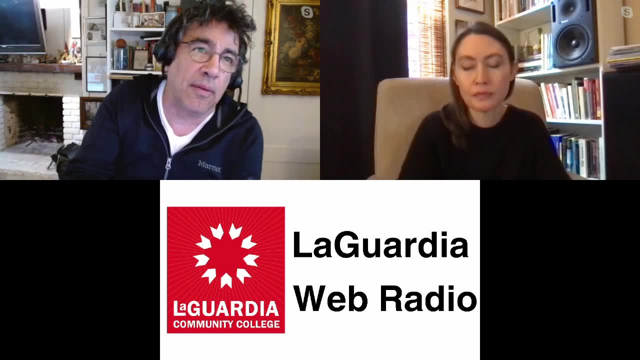 In that case, I also think. I also think about you know, we talked about this before because I, I, I I'd used the phrase psychology accidentally and you had to correct me into saying: look, we're talking about philosophy today, And but I remember years ago, in the sixth grade, 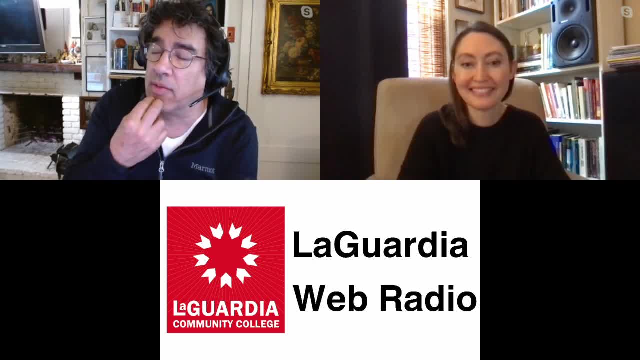 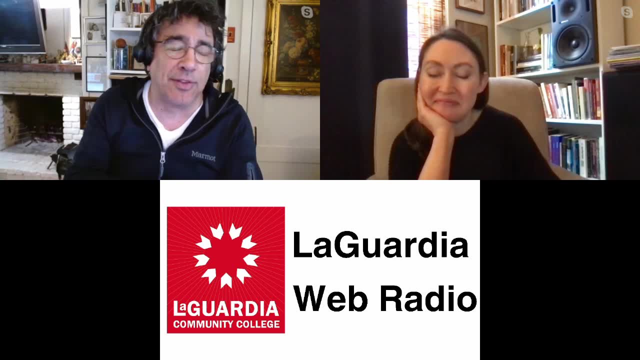 when I had a child psychologist show up to our course, our class, and talk about the warm fuzzies. Yeah, I don't know if you ever heard about the warm fuzzy world And I always, I always tell this story as a as an adult, because he, the, the psychologist, took us through. 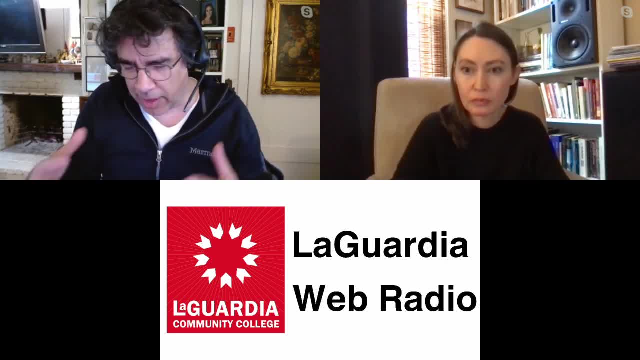 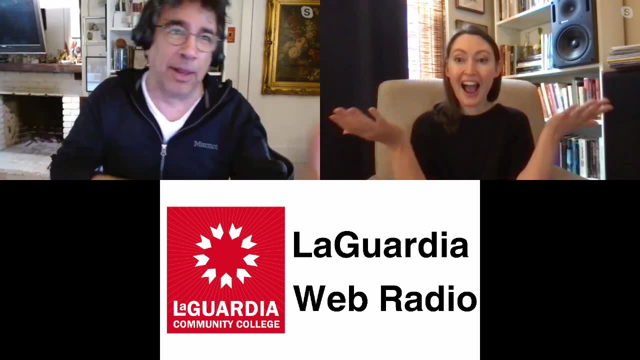 the whole thing And, of course, has created this incredible, complicated problem for the land of the warm, fuzzy people. And then and said: I'll be back next week, kids, And I don't ever remember him coming back. So as a child I grew up and I became an adult and I'm saying like 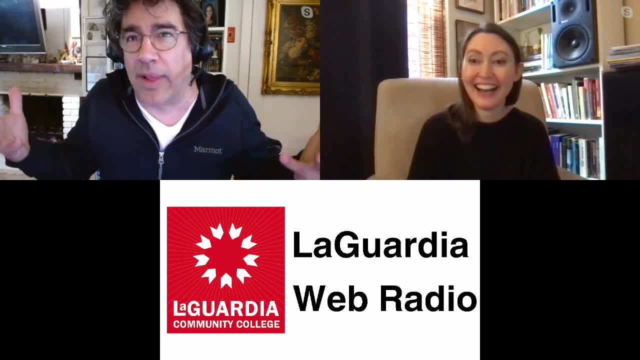 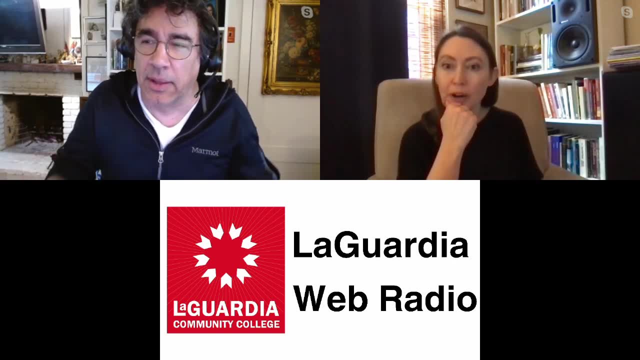 you know how is that supposed to? so eventually, yeah, exactly. So in the end, as an adult, I had to, I had to finish, you know, I had to come up with my own ending Right? And so, every once in a while, I tell the story to people, to children, In fact. 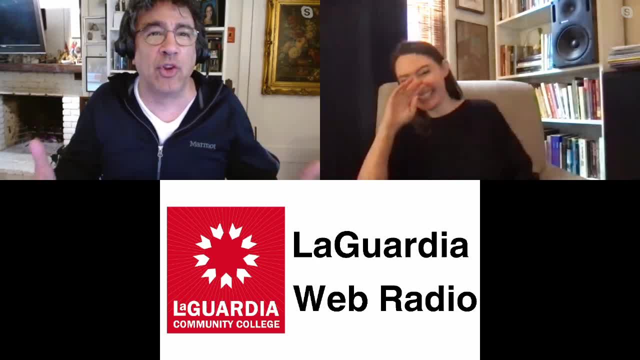 my daughter hates it because I bring it up all the time- but it's like: how would you have ended? How do you end? Yeah, How would you have solved this problem? How would you have ended the story? Right, It's something, you know something. it's funny because some people don't get it And then some 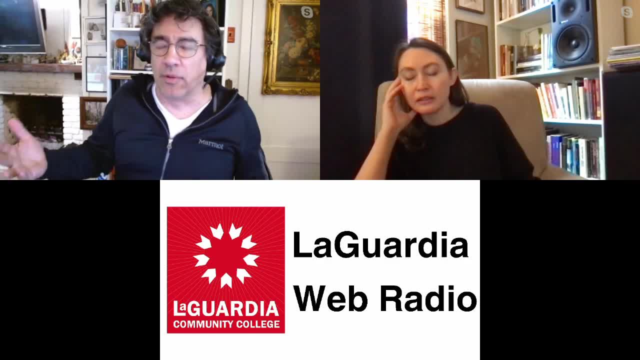 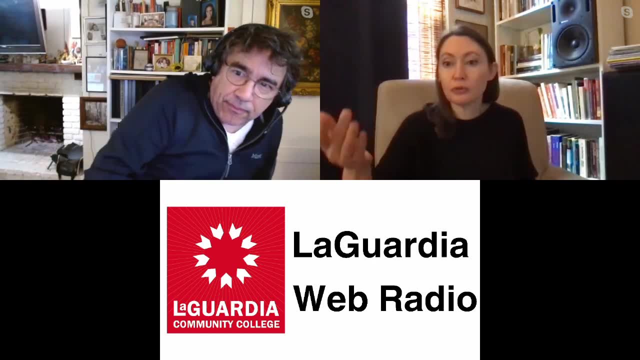 people. just you know they come, they come up with the same answer that I had to struggle. you know a decade or more to resolve, But I think that's a great essential model for philosophy for children. where you're like, I'm going to open this story. 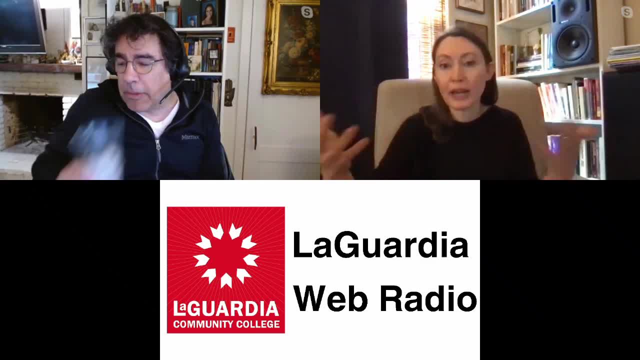 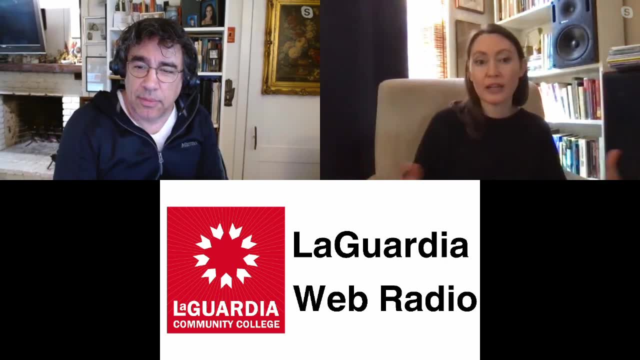 but then you're going to finish it And then we can talk about your various ways of finishing the story And like: what do we like? What are we not like? What are the reasons that we chose this, What are the reasons that we chose this other thing? And let's compare those together. 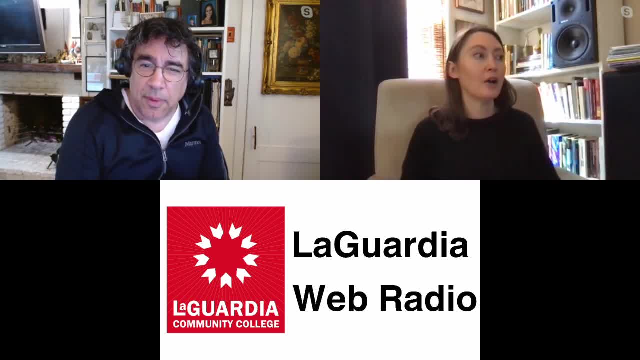 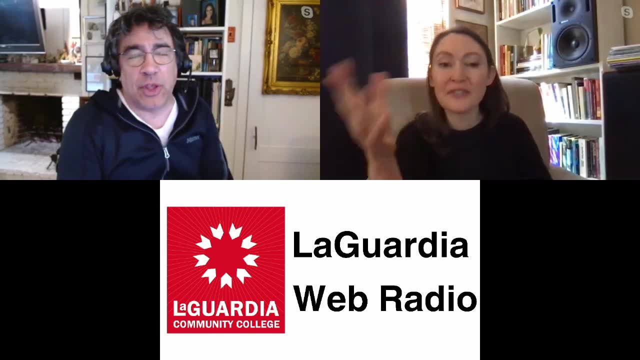 and see what we come up with, something that's maybe like collaborative. I'm sorry that you, that you, that you had to lay on this for a long time, But I struggled with all those. Yeah, it's funny, though. You know what was good about it: It because you know. 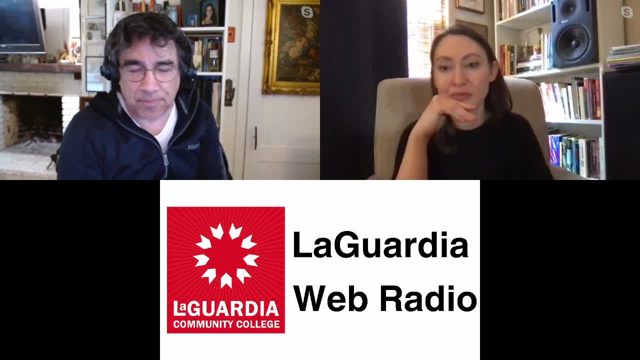 in the end I was like: I'm going to do this, I'm going to do this, I'm going to do this, And in the end, the answer you come up with becomes your ethos, Right. I don't know if it's. I'm not saying it's the right ethos, It's just it's mine. 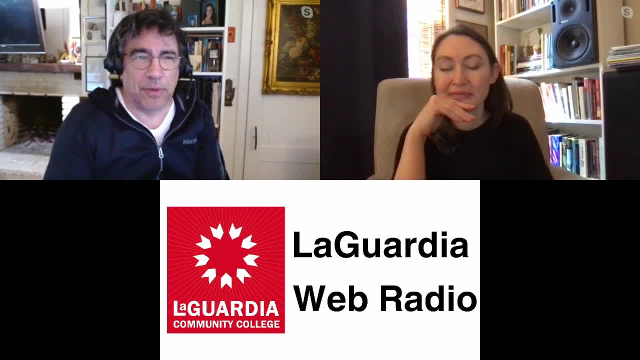 Right, Sometimes that it gets me in trouble. I I've thought about it like while we were talking here, just thought about it. It would be: you know when you get into, you know how, when you're interviewing people, for you know like we do through these search committees. 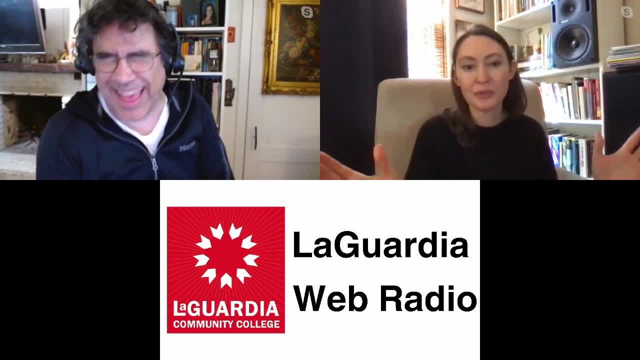 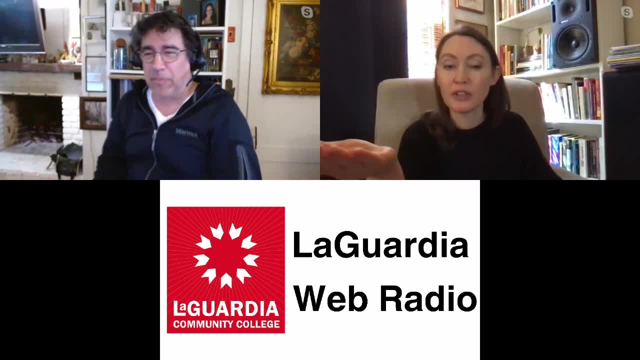 you know, telling them a fairy tale and say, okay, how would you? and you would know exactly who you're dealing with. Yeah, no, you would, you would. And here's, here's another cool, cool model for philosophy: for children is like taking a classic fairy tale, like you. 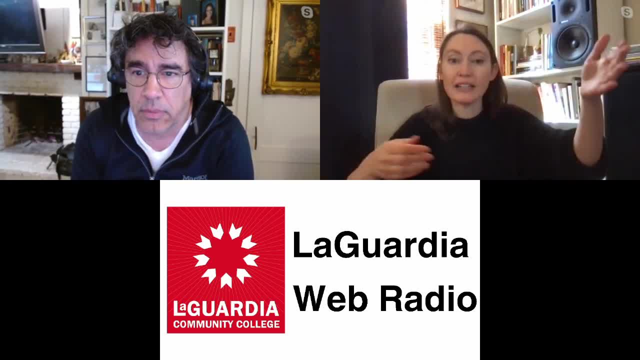 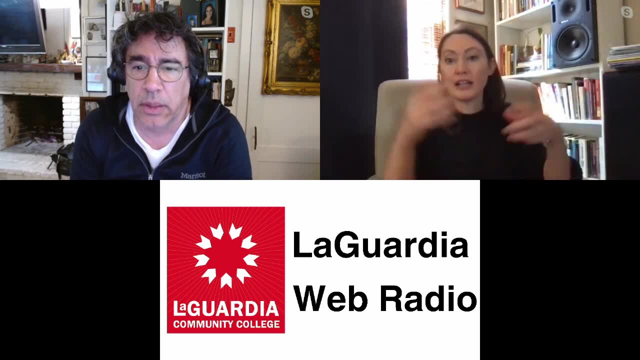 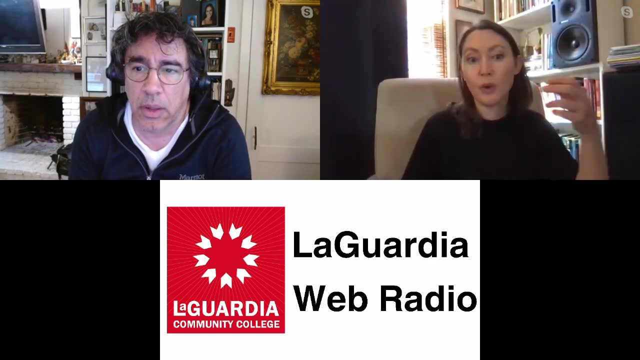 know your Cinderella or your Snow White, and telling the story and then asking, like, well, what would you change if you were going to retell this Right? So not just like here's an open ending, but like, what would you change about the story that we all know very well? 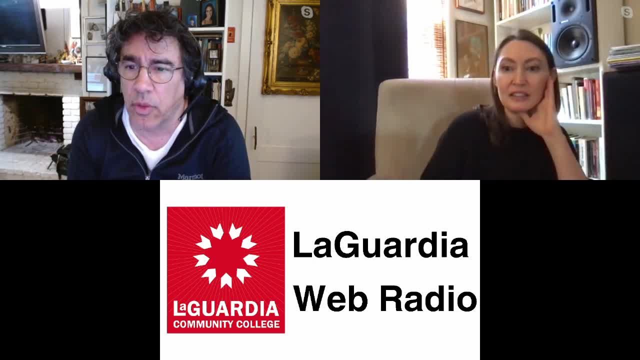 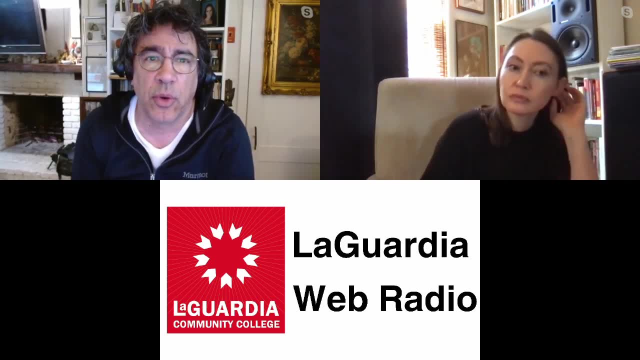 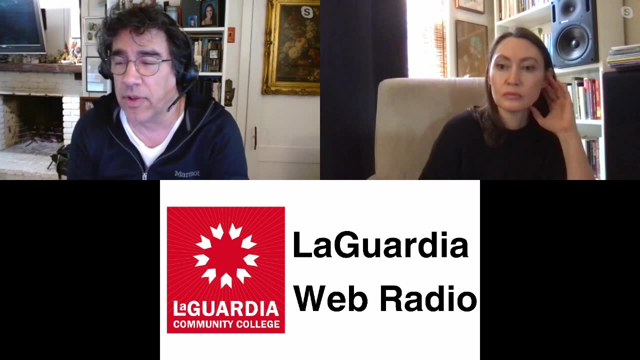 Yeah, John Gardner, you know the, you know the work of John Gardner was a oh a writer And he retold the story of Beowulf from the perspective of the monster. And I don't know if there's anything to be gained from that for children as well. You know to tell the story. 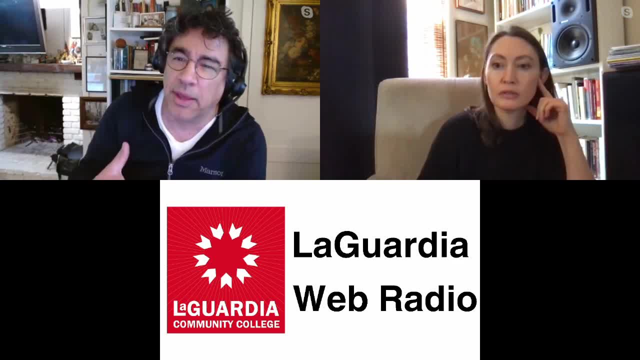 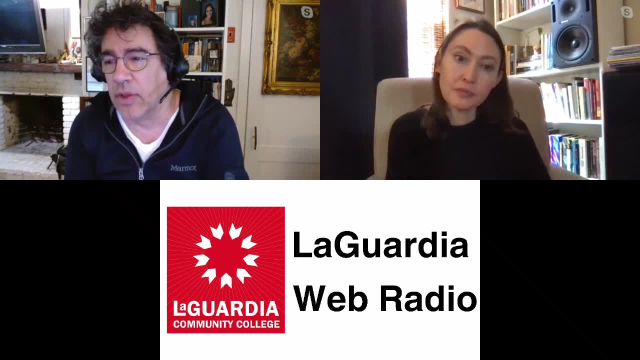 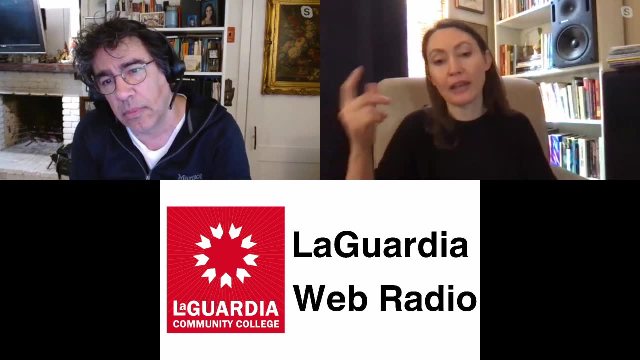 you know again, Cinderella, what would, what would? what would the story be from the stepsisters and Cinderella and the things that they're trying to do? Maybe there's more to be gained from that. Well, isn't that? isn't that the kind of move that something like Wicked makes? 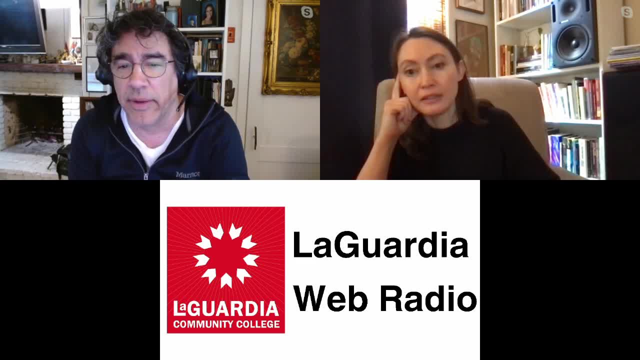 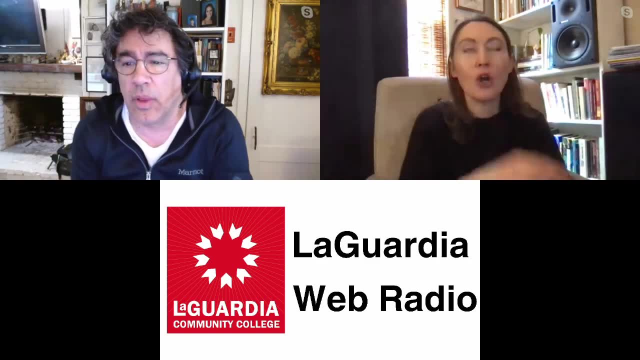 Oh, exactly That's exactly what. yeah, So I guess it's all being done already, Right? I mean, yeah, there's plenty of work to do out there. What's the methodology And in what ways do we want to change it? And what does that say about who we are or who we want to? 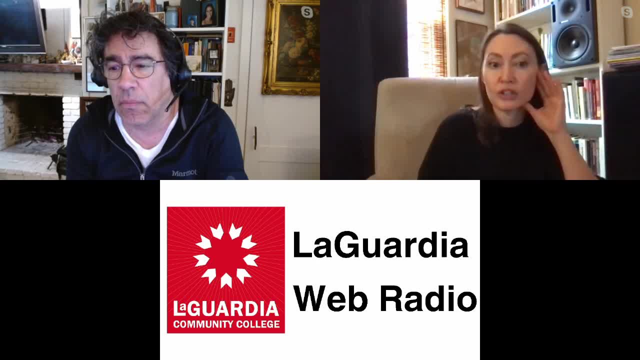 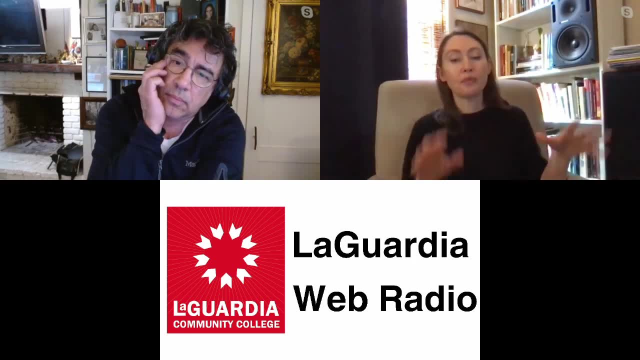 be. Those are, I mean, those are the really urgent questions. So what, what kind of success have you had with this work here at the college? So there definitely have been people over the years who have tried to do an assessment of like. 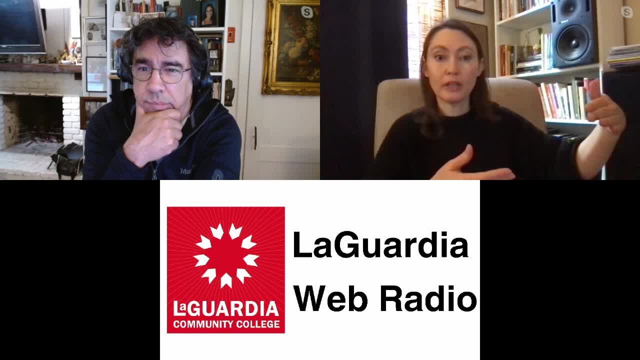 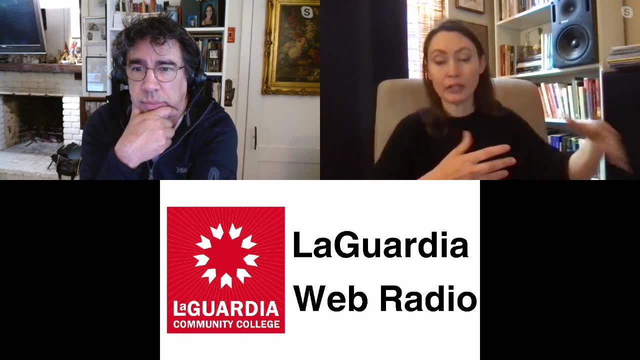 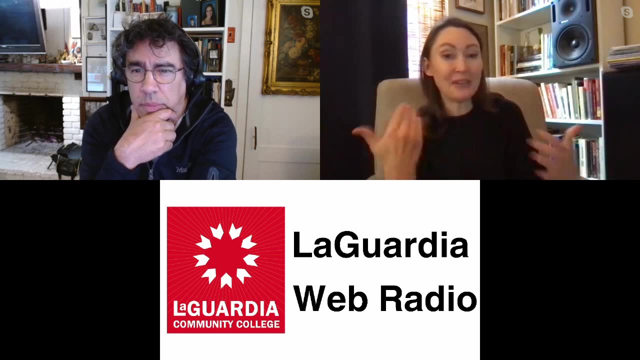 how does, if it does at all right, how does doing philosophy for children support students, children in their growth? you know, academically I do not do that kind of research, primarily because I don't feel comfortable not coming from a background in social science. 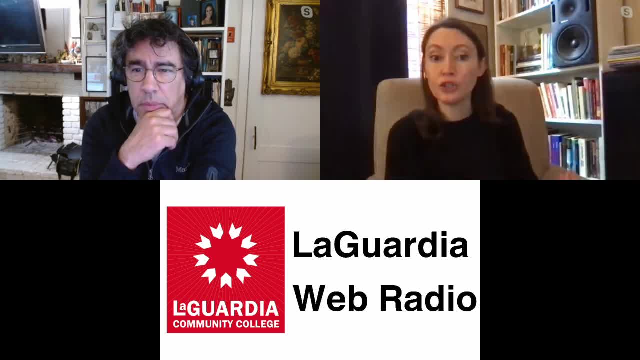 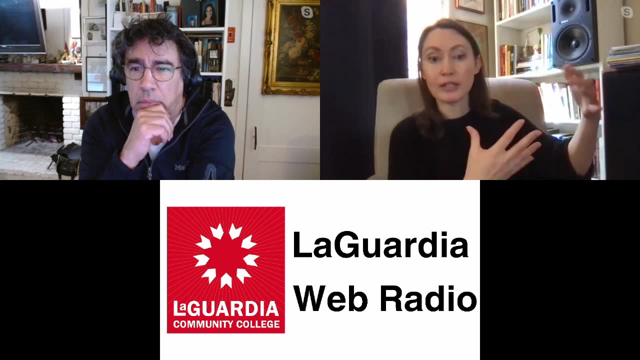 you know, developing that, those kinds of research projects. But what I do is- and this is what the other thing that's super unique about the philosophy for children work that we do at LaGuardia is that we have interns right. So I have an internship that has students. 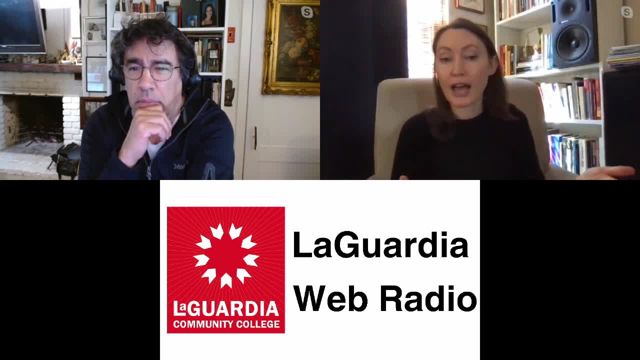 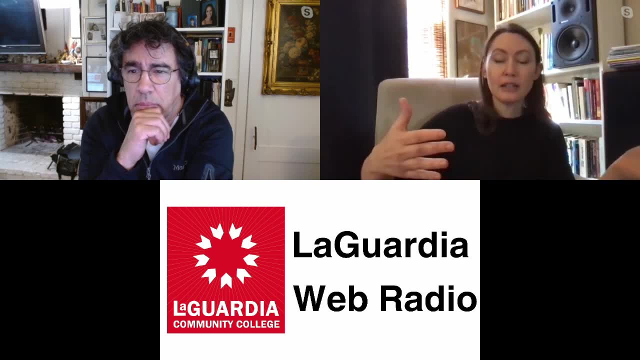 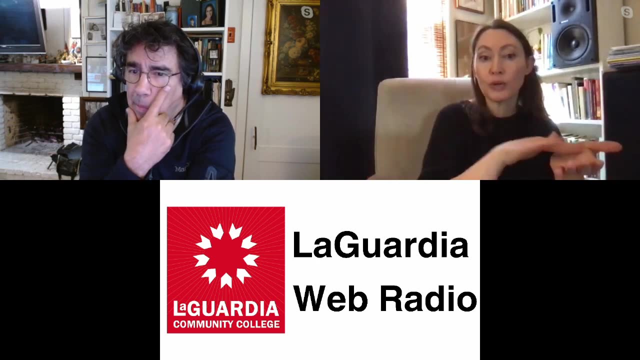 work with me, shadow me in the philosophy for children classroom, develop their own lesson plans, read, write, like we discussed, and they get a you know trial by fire right in the philosophy for children world. And so the research that I've attempted to do that was sort of beyond the philosophical research of 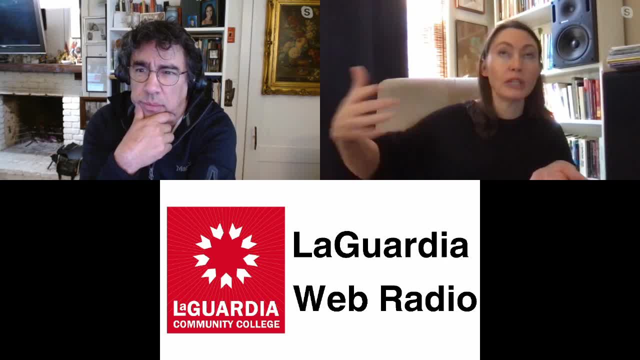 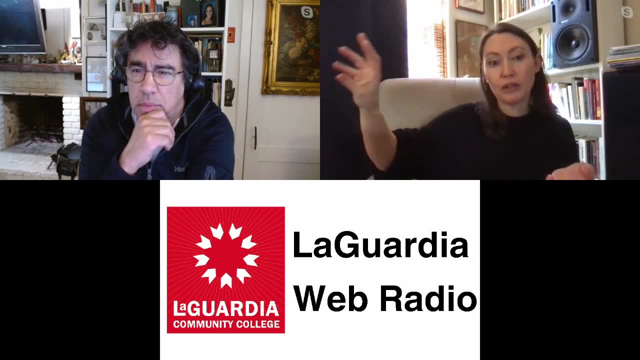 like okay, so what can this tell us? How do we relate to these concepts And how do we want to change them, Is asking not how is this improving the academic performance of the children, but how is this affecting the academic performance, learning and growth of our students at LaGuardia? 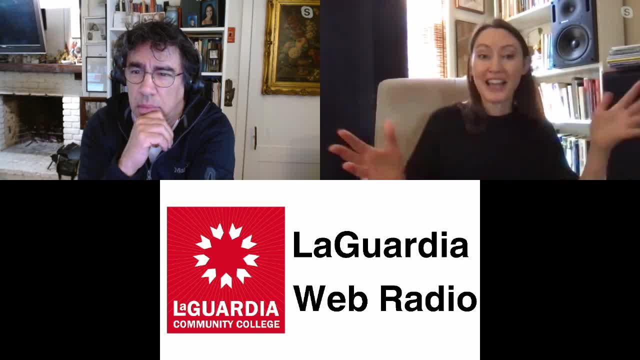 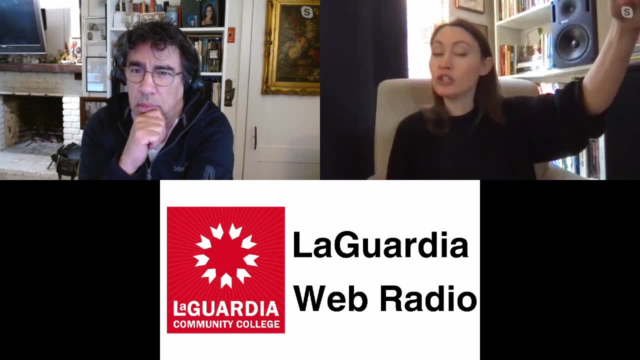 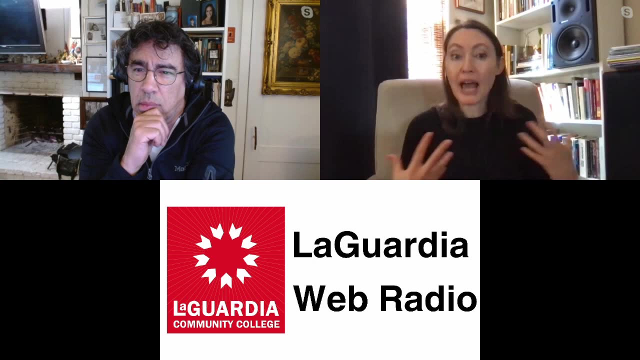 So the ones who intern for me, And that's that's very unique right That it's typically the case that in philosophy for children you don't start to get to do philosophy for children in the field until you're a grad student, And so that was my introduction to it. right was as a grad. 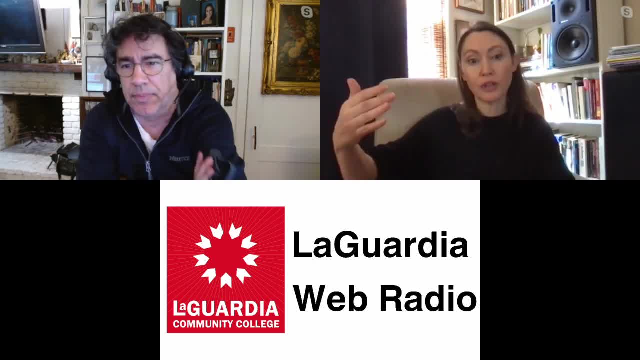 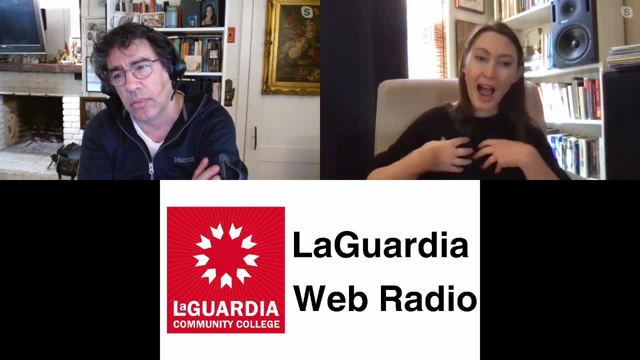 student. I already had a lot of background in philosophy in many classes behind me before I ever walked into the classroom with the children. I'm a little bit radical here within the philosophy for children world but I think I do genuinely think that everybody is a philosopher. You know, some of us have like thematized that more or less in our lives, But everybody's a. 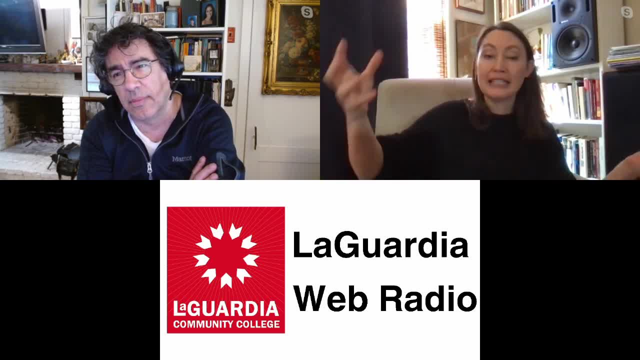 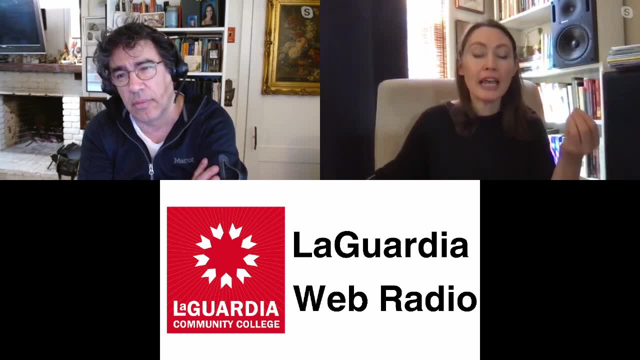 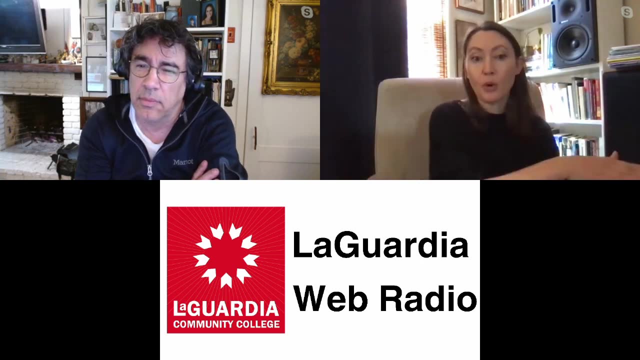 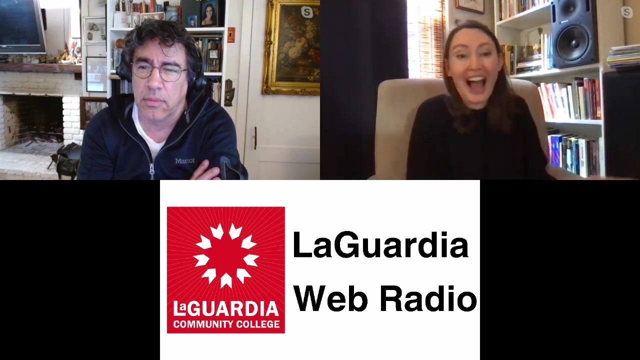 philosopher and you don't need a deep background in the history of philosophy in the Western context in order to engage in the type of deep, rich philosophical thinking that is what really matters, And so what I try to do with my interns is to say: listen, you know you've taken a philosophy class because otherwise you wouldn't be in my office, So let's try to build on that so that you can engage in these kinds of dialogues with children who also don't have a lot of background in philosophy but can still engage in these philosophical conversations. 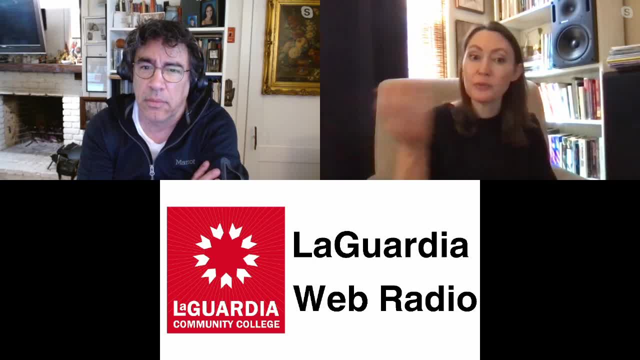 And some of my best interns have actually come from the art field, because they're coming with a lot of creativity, a lot of willingness, this to play. And I'm not an artist, but I've had the students from art who've come to be my 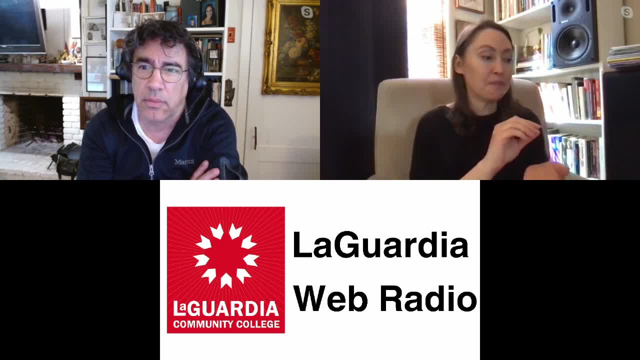 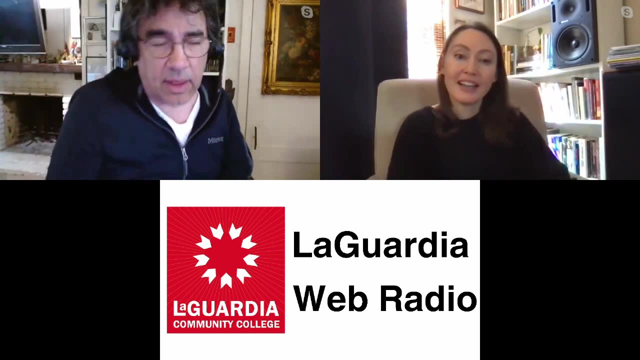 interns who have developed different puppets for me and different coloring projects and different painting projects for the children, which have been wonderful. Yeah, just listening to you I think about. I told you I can't. obviously I'm not a philosopher. 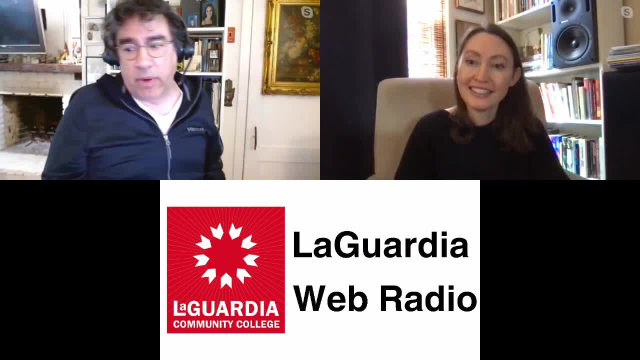 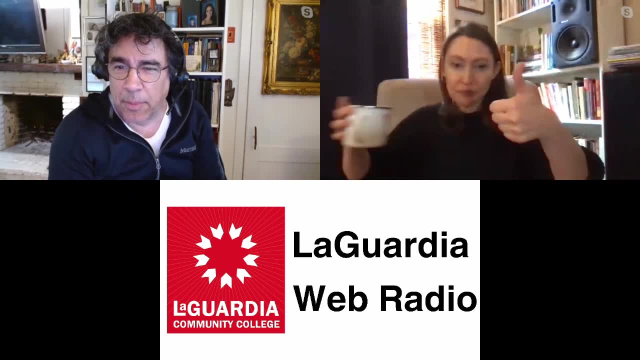 In fact, I never took a philosophy course when I was an undergrad, which I guess I'm sad about, Though I do. I have been watching Dr Brown's videos that he's still got up on YouTube, Consciousness Live. He's in season six. 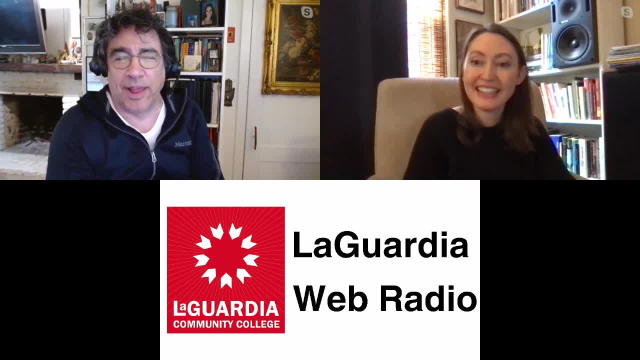 No, I'm talking about, like you know, his intro to philosophy. Oh nice, The old lectures he did like 10 years ago, And I just love it because you know, suddenly you're thinking in a way that you don't typically think Most of us walk around and take. 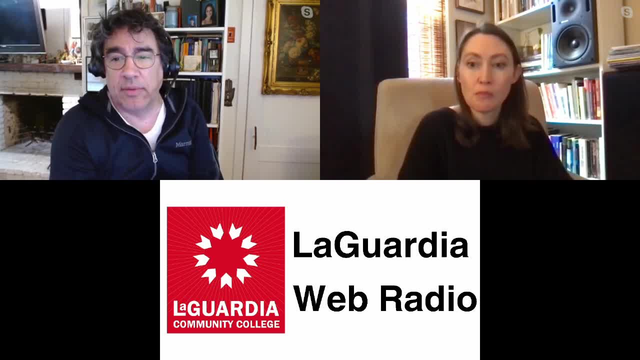 everything for granted, Mm-hmm. But I have been a parent and you know I just I can only use the example- my daughter raising my daughter, And you know it's that thing about. you know, kids ask the funniest. 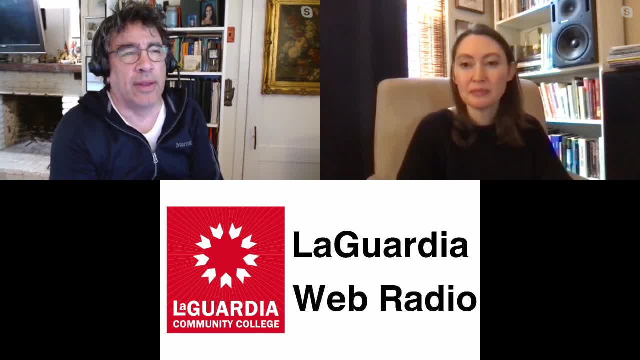 questions and blah, blah blah. And I just remember our dialogues with each other and she'd ask things And a lot of times, you know, sometimes I'd have the answers, Sometimes I would encourage to look things up, Sometimes I would base it on what I thought I knew. 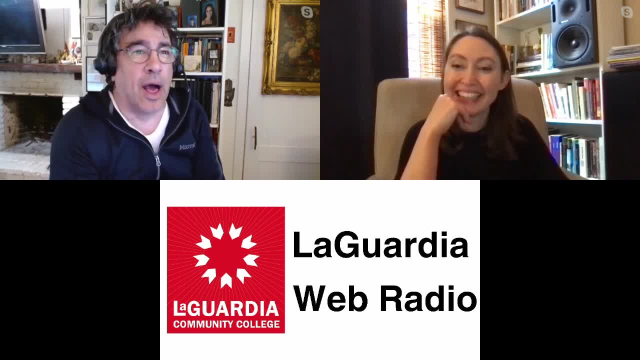 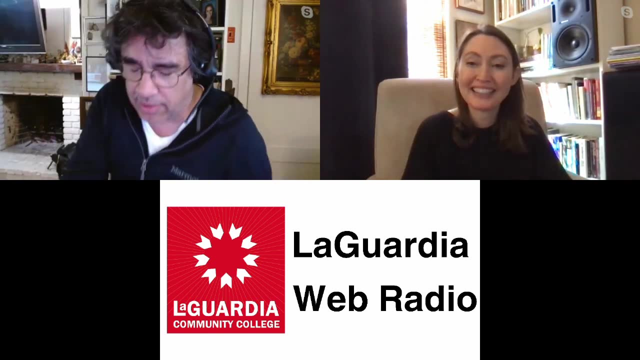 Yeah, And my and over the years my daughter got into a habit of fact-checking me- I love it- And bringing up and saying, like dad, this: you know, like I once had a Napoleon quote about: no child has ever been, no child has ever been raised correctly And she said: 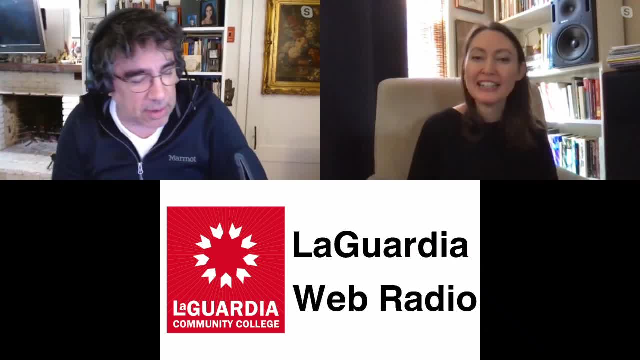 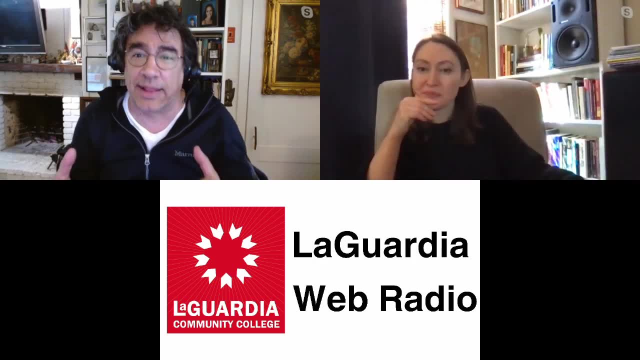 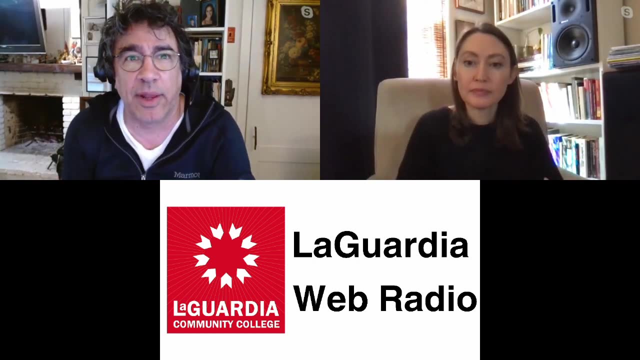 Napoleon didn't say that. dad, Did you just make that up? I could have sworn he did, And somebody told me he did, And I can't, I can't find it. That's the problem, I can't find where it is, And but then sometimes you know, things will happen where you know. 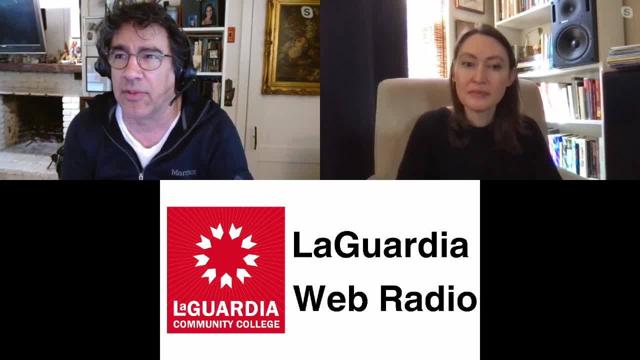 she'll use some little tidbit. I've told her and in a class and and impress the teacher and say, oh, that's my dad And this, you know, Jeopardy headset. She turned out pretty good, You know. 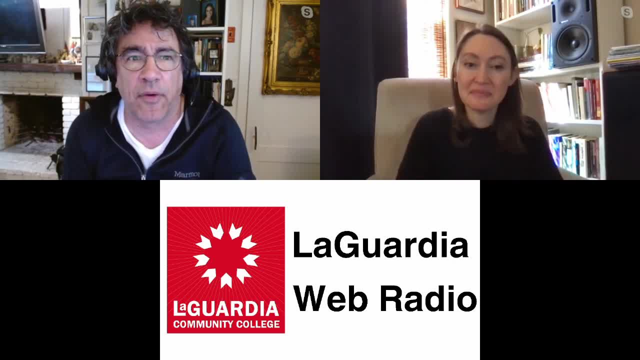 she became an investigative reporter and did that for a while And I can't, I can't. I guess I got to take credit for everything, but I just wonder how much credit I can take, or those dialogues that we would have, Because you know parents, you know what do parents do. 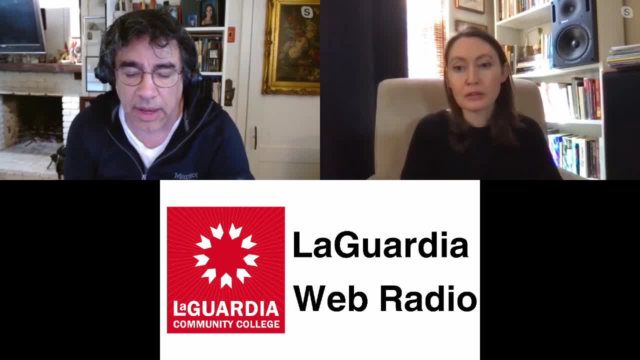 when children ask them very tough questions. Not even- I'm not even thinking about, just like you know, who was the first president or whatever. it is those kinds of questions just about. you know tough questions in life. You know. why is this? Why is that? 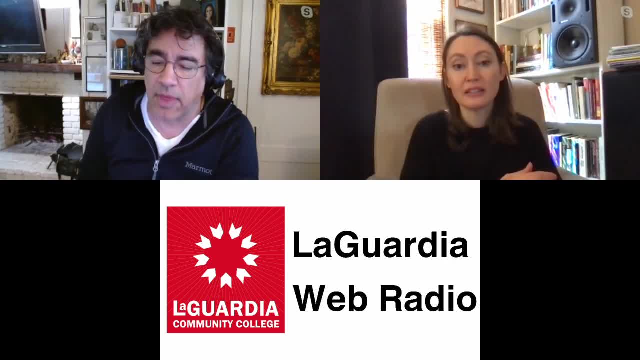 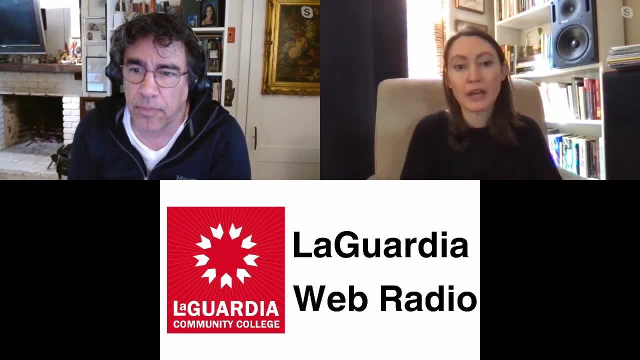 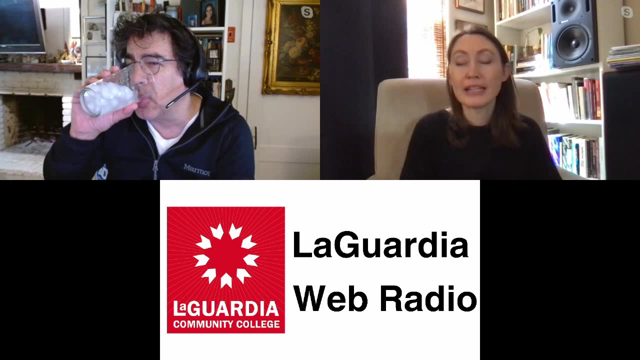 The philosophical, mystical type of thing. So is this something that could be taught to you know parents, for parents to use in everyday life? Yeah, definitely, There's skills that you can develop in these kinds of conversations, I think that it's actually, I think, pretty straightforward When children ask: 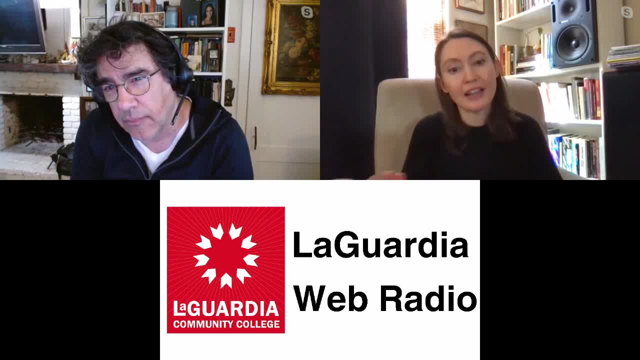 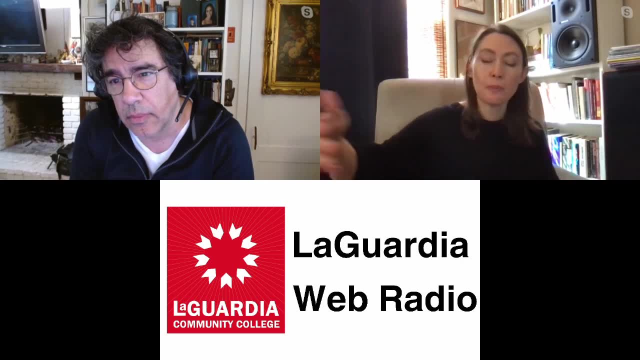 empirical questions like: who's the first president that just look it up right? Give them the information or teach them even better. teach them how to look it up. Make sure that you have a dictionary In the house, that they can look things up and they're not going to get sucked into a screen. 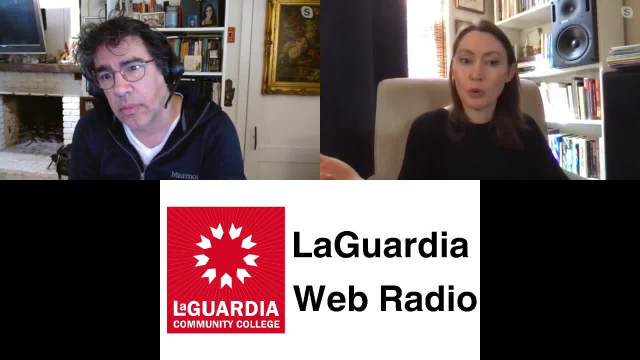 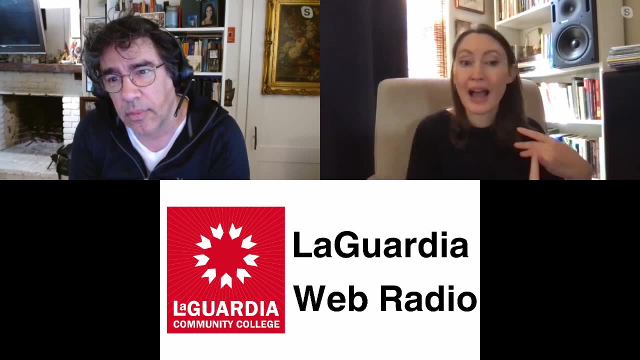 But when they're asking those more philosophical questions, questions like these are the ones I get from my kids. Where did we all come from? Well, what happened before that? How do we know What happens after you die? I had a long conversation with my child who's? 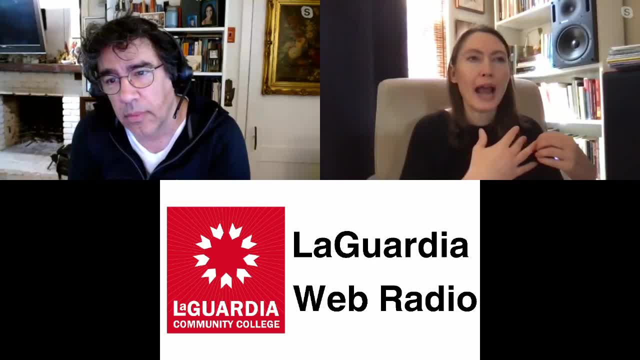 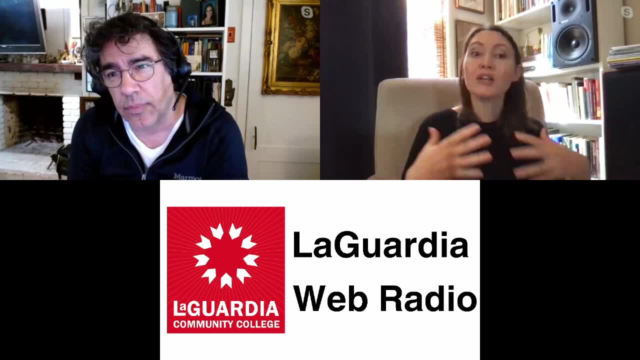 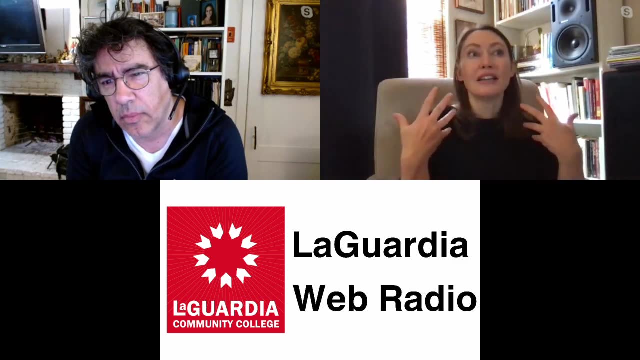 five About what happens when the sun explodes, which is an empirical question, but also a philosophical question about, like, what is our relationship to our own deaths? And those are tough questions And the way that I try to approach them is the first thing that I try to do is say: you know? 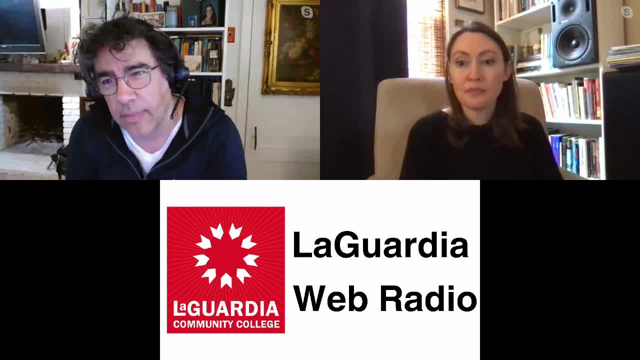 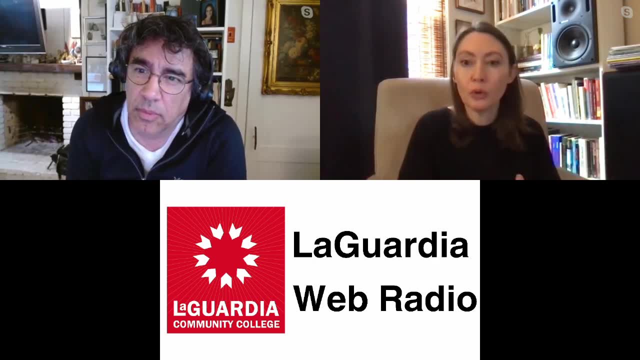 I don't know. What do you think? You know, I don't know about us, what's going on? Where do you feel like you're at? So I start the conversation where I definitely have thoughts about all of these questions, but I want to know where they're coming. 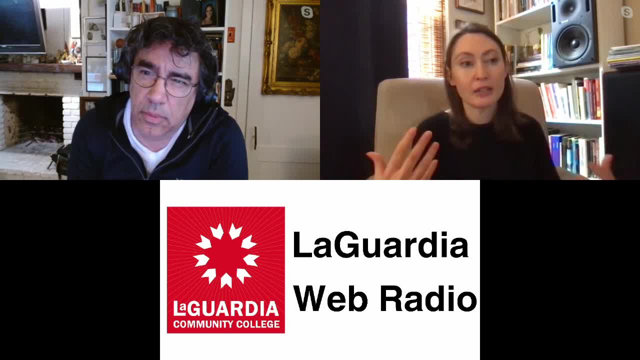 from first. I want to know what they're starting out with first. So my child says: What happens after you die? I say: What do you think happens after you die? They tell me or they'll say I don't know. 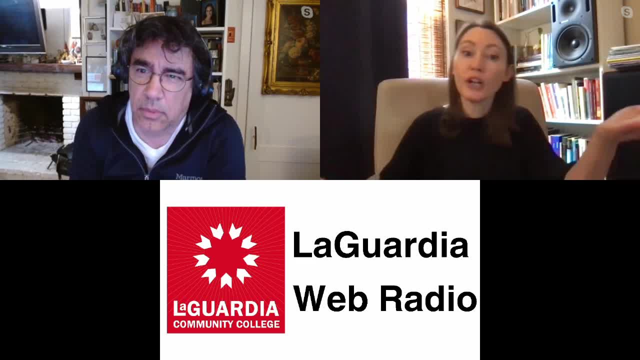 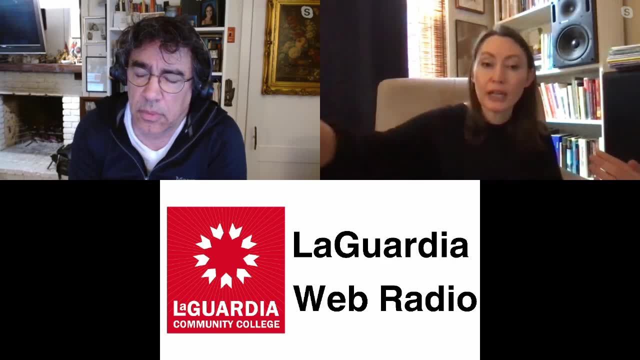 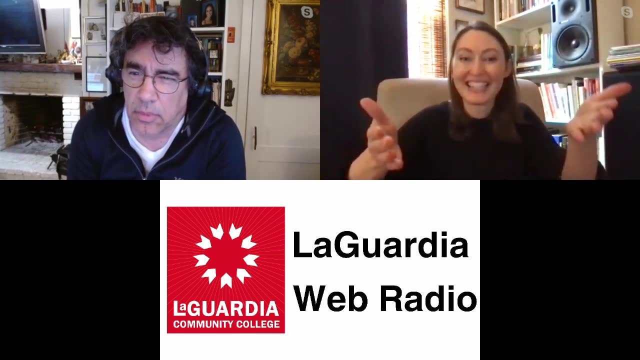 And I'm just asking you, And then you know we can start a conversation. Well, some people think this: What do you think about this? And then you're opening, as you say, like you know, you're entering into a dialogue where it's not just: I have the answer. Now, you know it, Unless there is an answer and you can just tell it to them. 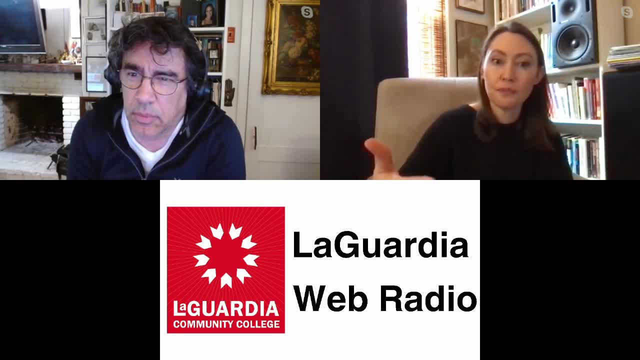 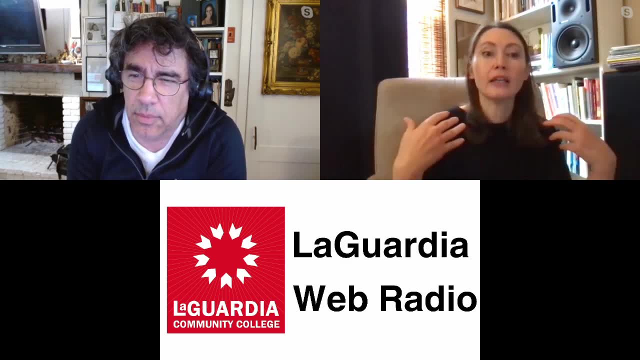 That's an expression of my values too. I'm teaching them and I'm modeling for them this process of listening, of dialogue, of looking for different perspectives on an issue and trying to come up with some sort of answer that we can both agree on. 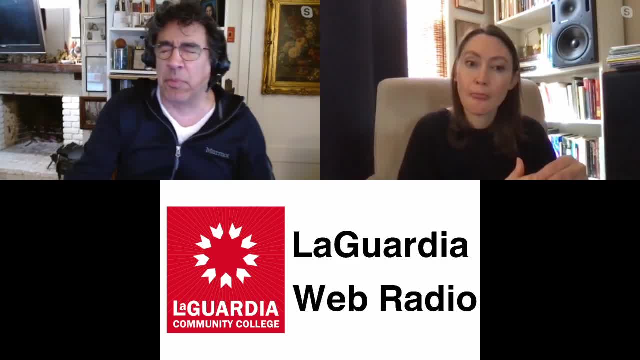 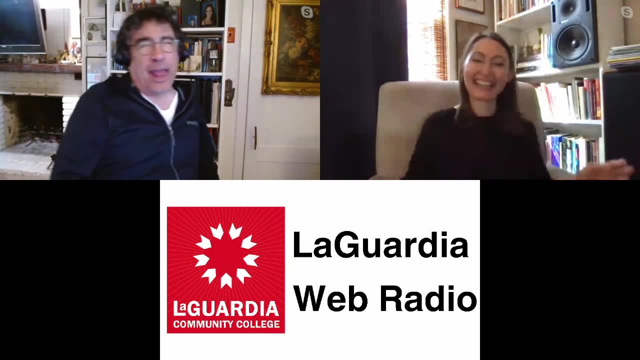 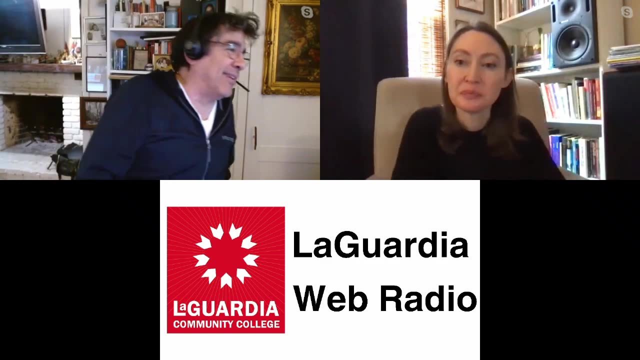 I wish I you know, because I'm thinking about tough questions. my daughter asked me And the toughest one is: is Santa Claus real? And let me just say I did not do well, And how did you answer? I can't go on the record for that one. 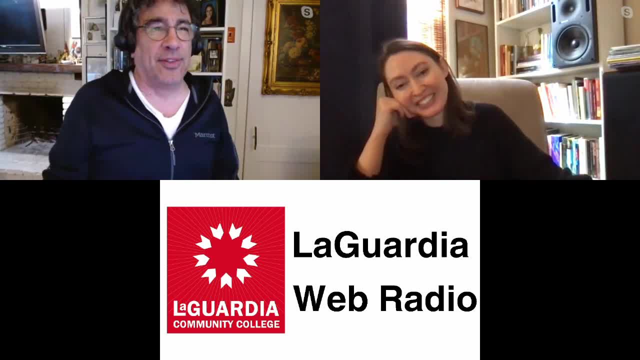 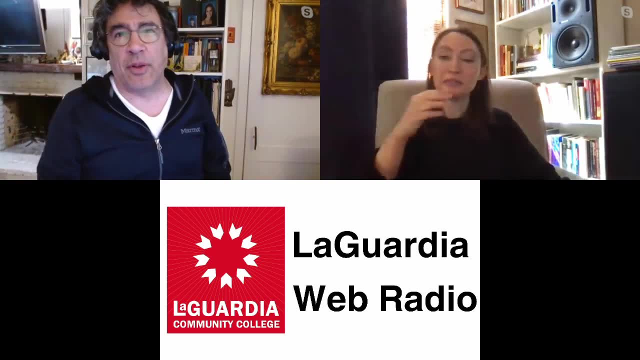 But let's just say I've regretted it ever since And I've learned a lesson, And you know I'll certainly speak to parents off the air. Let's put it this way: My answer, what the answer should have been, or ideally would have been: 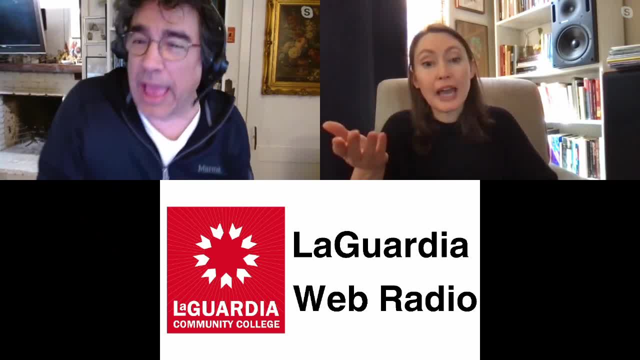 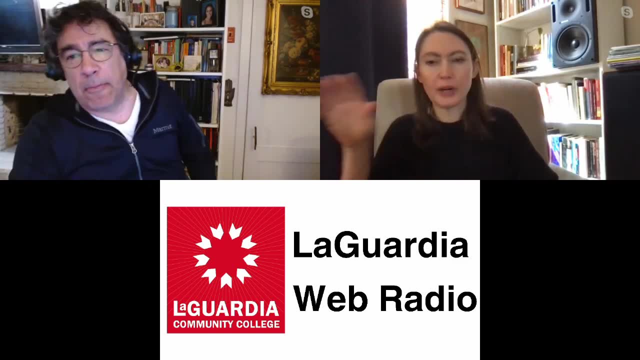 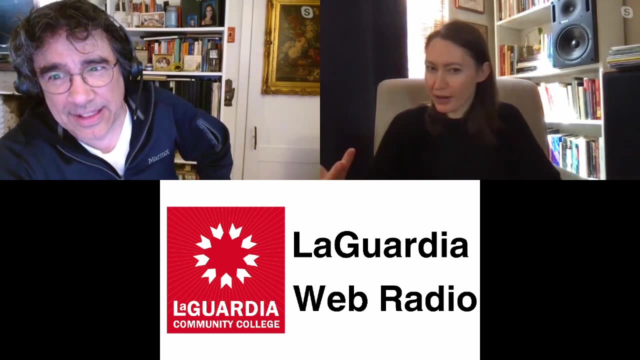 Is he's real if you think he is? So I did get that question from my child last year. for my younger one, not the older one. I feel like the older one has actually like gotten the memo that as long as you believe Santa is real, Santa brings you presents. 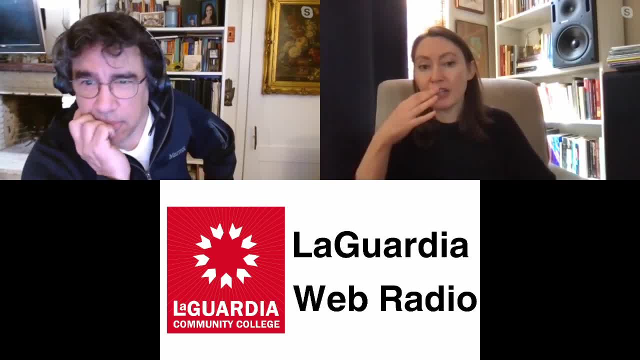 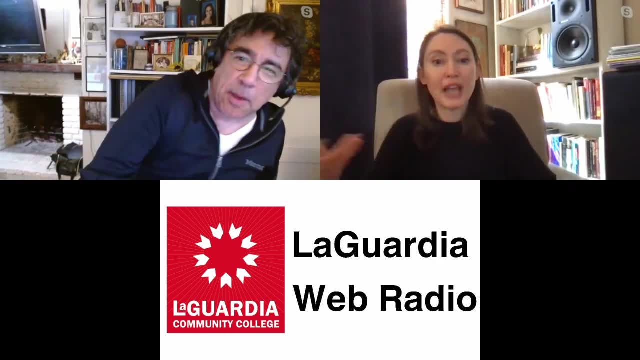 But the younger one asked me- you know she's five- and she asked me: is Santa real? And I said: well, it depends on what you mean by real. So let's talk about what's real. And so then we had a conversation. 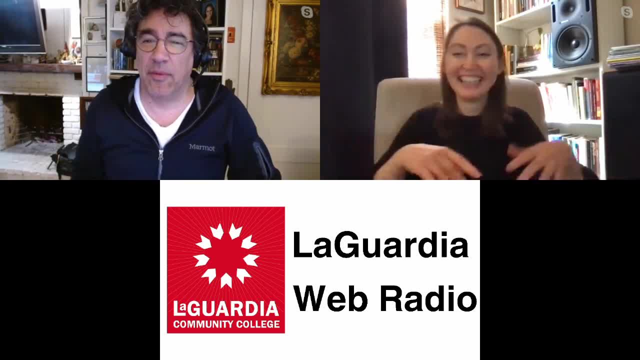 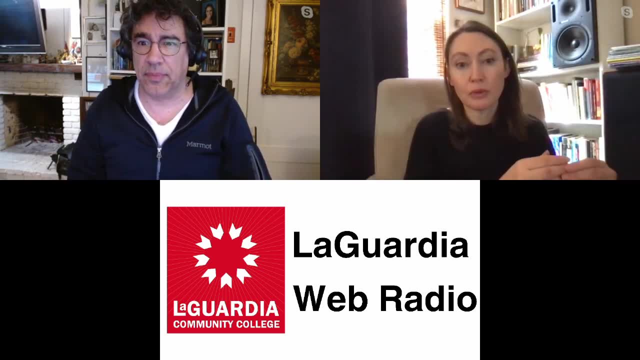 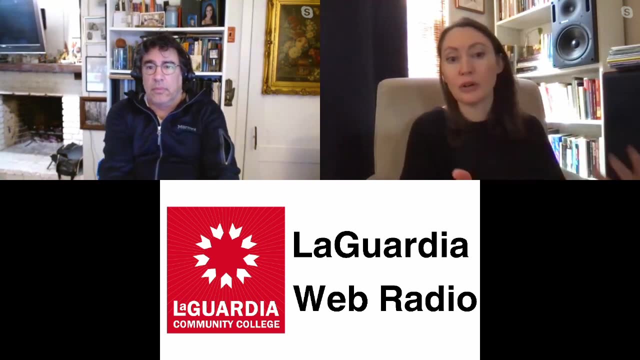 She hates, she hates it. She just wants me to tell her the answer. She's less inclined to these kinds of conversations, But yeah, we had a conversation about what counts as real And you know, I think Santa is real in the sense that a kind of like spirit of generosity or like magic in the world is real. 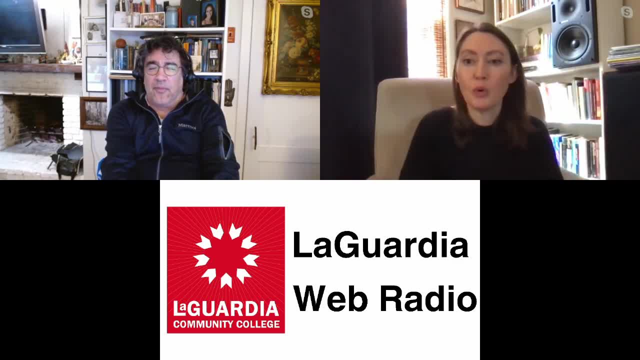 It's real when we believe it and it's real when we make it. when we make that happen, Is there like a joke, Is there like a jolly old elf? somewhere You can just say: you're getting presents, aren't you? 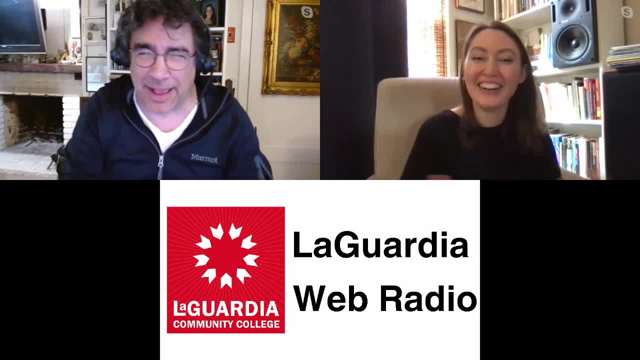 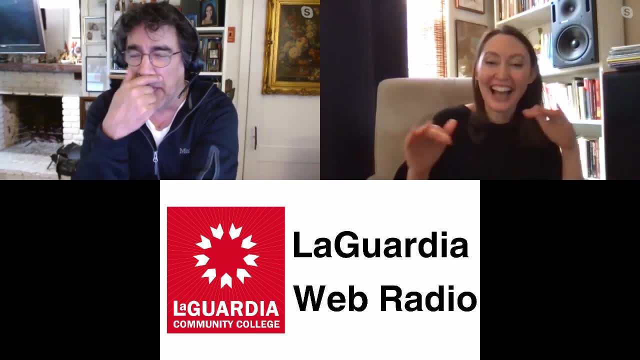 Yeah right, This is the parent who doesn't want to have that kind of just says you're getting presents, aren't you? So stop asking questions. You know you have that little. yeah, exactly, You have that whiteboard on your door. 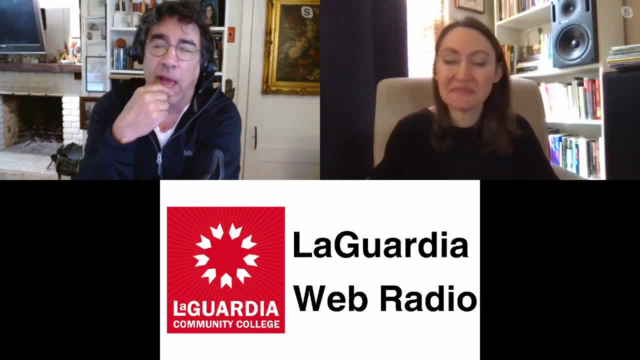 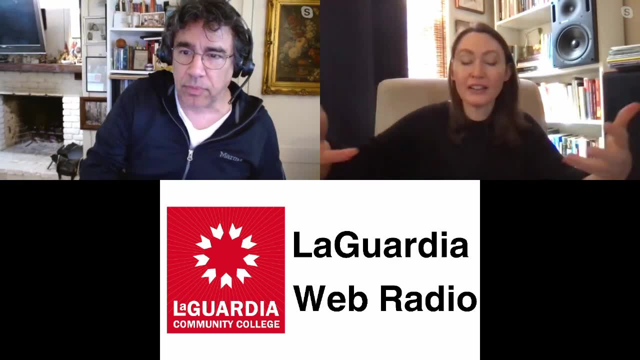 You know, outside your door you have that whiteboard And you had that question. The word real was in there And my response to you was going to be: define real, Right? No, that's exactly: Define reality. That's the right response. 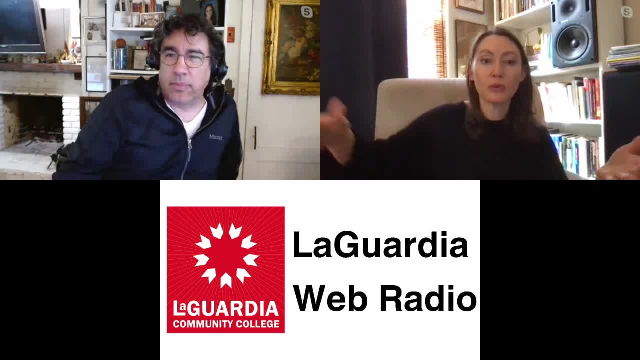 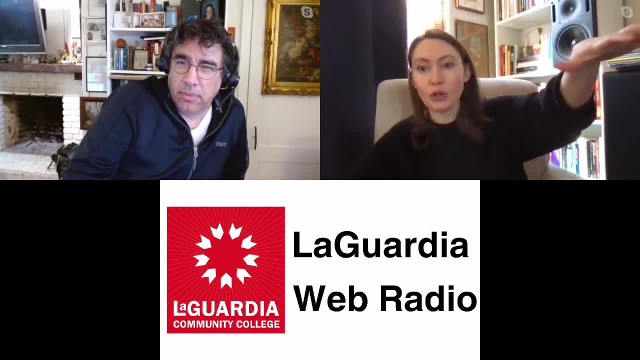 Whereas, like, what do we mean by real? And if we mean by real something that has, like a existing right, correlate in the world that we can like, see, touch, feel, right then Concrete Yeah. 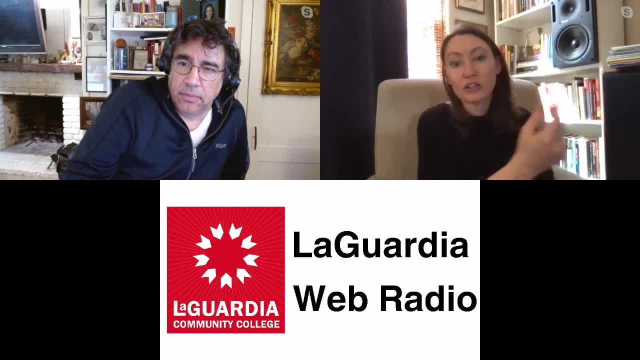 Or in some way we can like measure it Then, like there's lots of things that aren't real but that we still talk about, and we still and still have an outsized impact on our world Love, Yeah right. 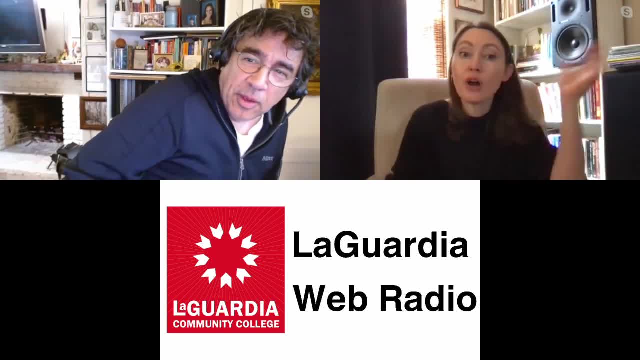 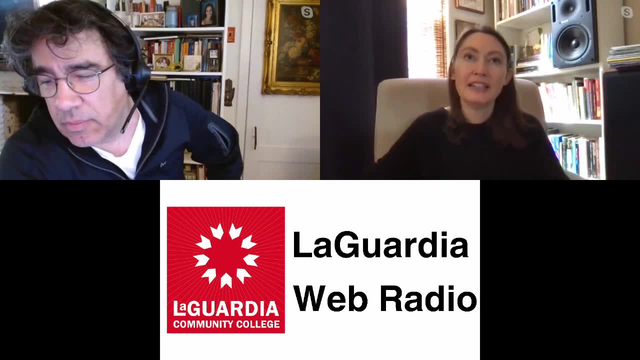 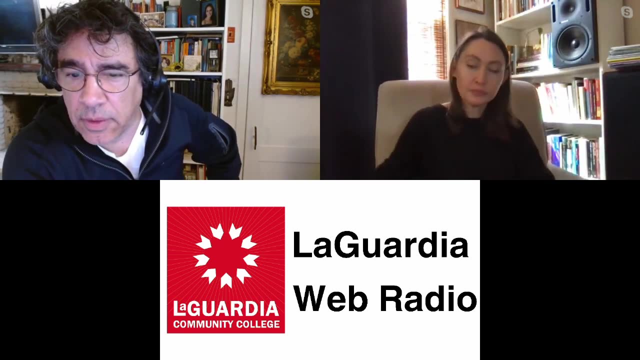 And compassion, which there isn't enough of Trust, Justice, Right, I mean Right Your ideas, So they're abstract. We're in the last quarter of the show, So I wanted to give you an opportunity to talk about the future of you know. philosophy for children. 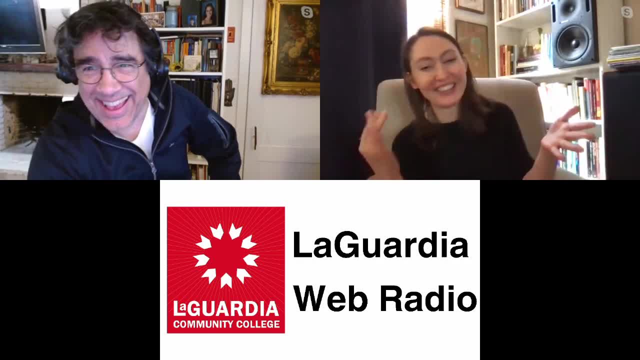 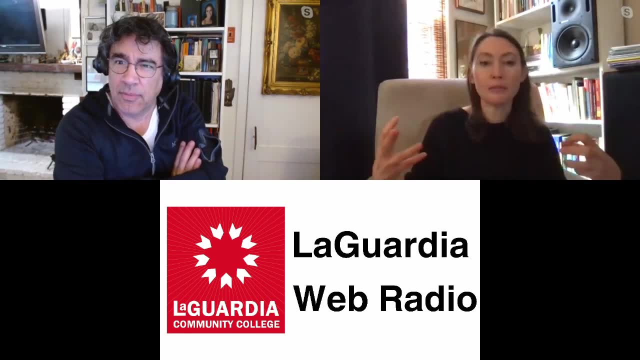 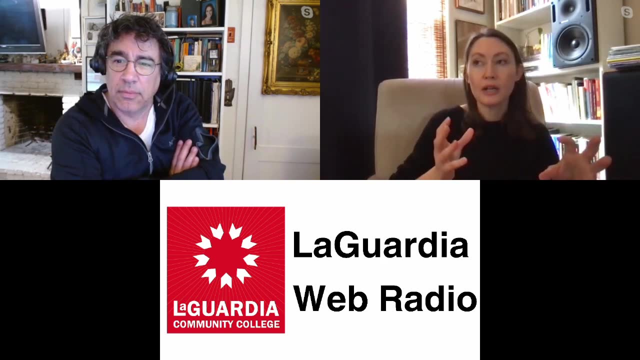 Is there any future? Yeah, I mean, I think What I would like to see are So. the philosophy program at LaGuardia Is really part of this ongoing process that we have of growing- is that we're trying to pivot towards a more community-based philosophical approach. 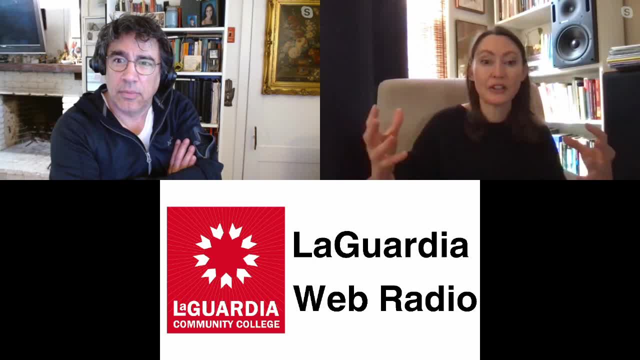 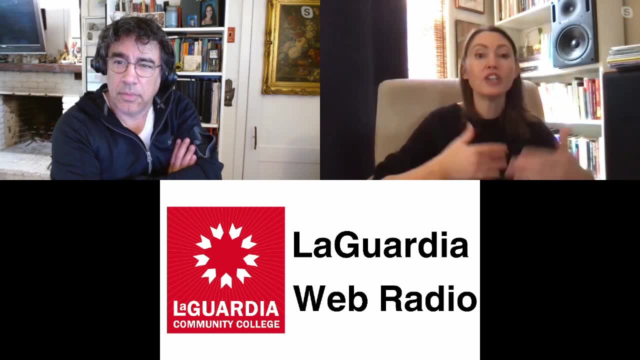 So in the fieldwork it's called public philosophy, But that doesn't necessarily mean it's like out in the public, Like philosophy for children counts as public philosophy because it's engaging with the community outside of academia. And I see, especially as a community college, that one of the things that we really need to do is to engage with the community outside of academia. 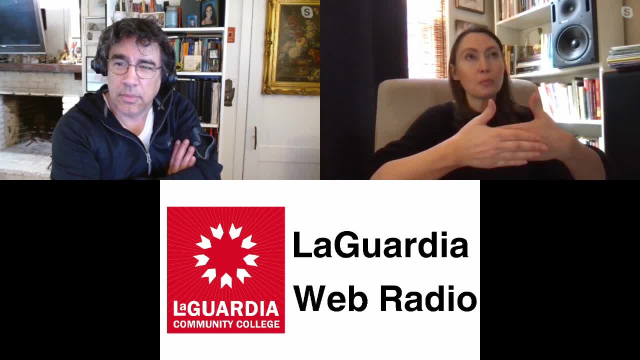 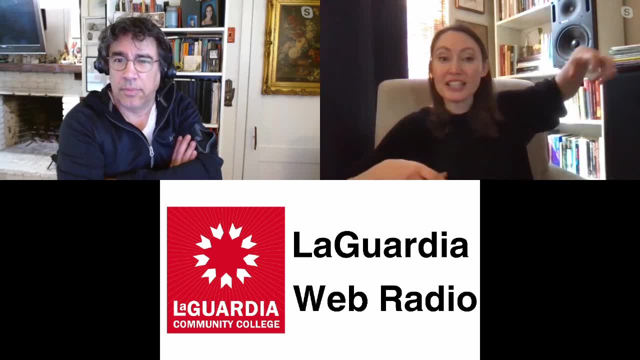 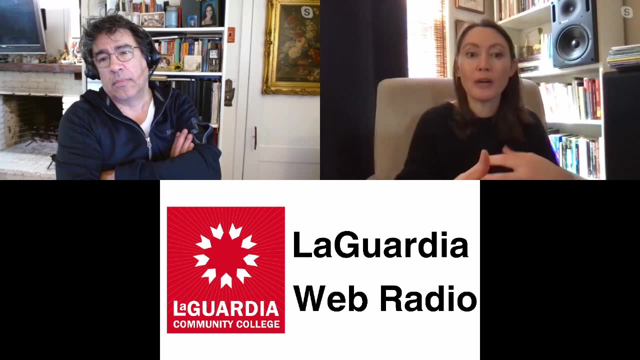 And one of the things that we really want to do is we're kind of at that, We're in that sort of liminal space between right, the community and like the kind of elite college system. And so community college is like exactly where a community-based philosophy sort of program I think could really thrive. 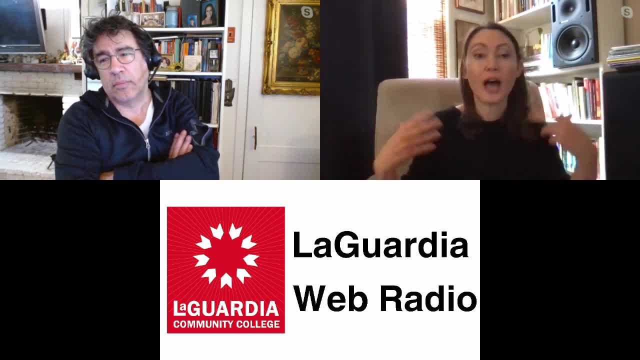 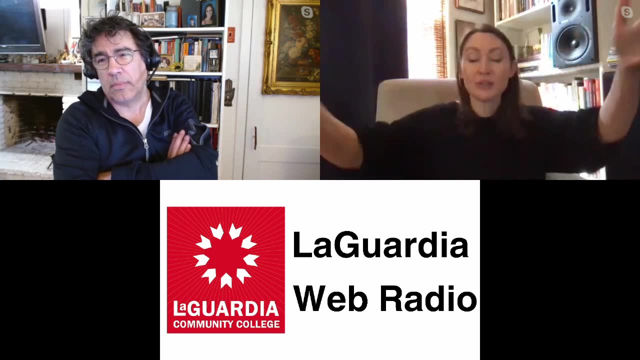 And so we're pushing in that direction through lots of outreach that we're doing. So I do the philosophy for children program. Shannon has been active in philosophy. She's been active in philosophy in the prisons. Andrew has been working with the Queens Library to do these kind of public sort of outreach, sort of let's all get together and talk about philosophical questions. 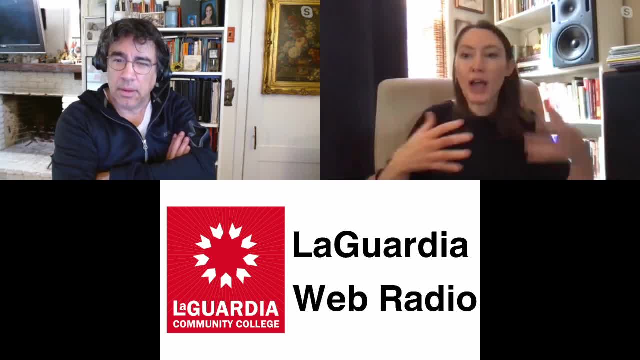 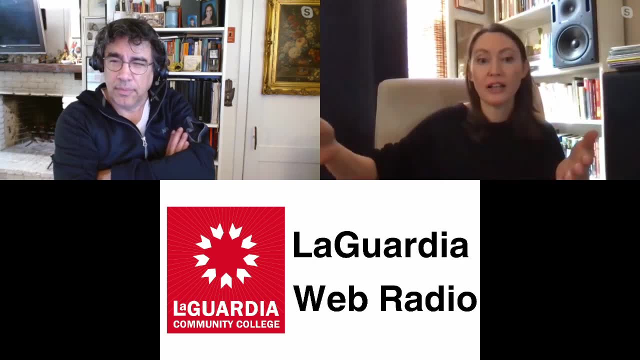 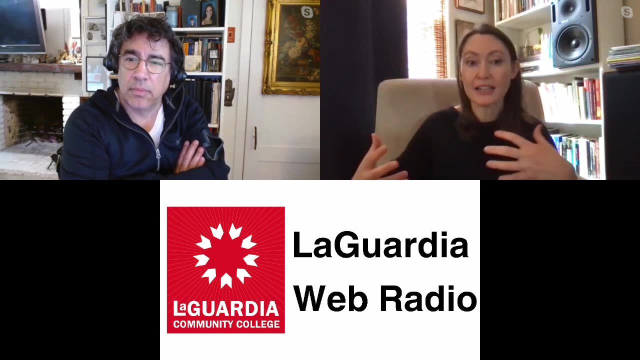 And, of course, Richard, with Consciousness Live. Lots of us are doing these kinds of public philosophical projects And we're trying to develop more internships to be able to get our students to not only be able to access, But also to be able to get them to be able to access the science of philosophy. 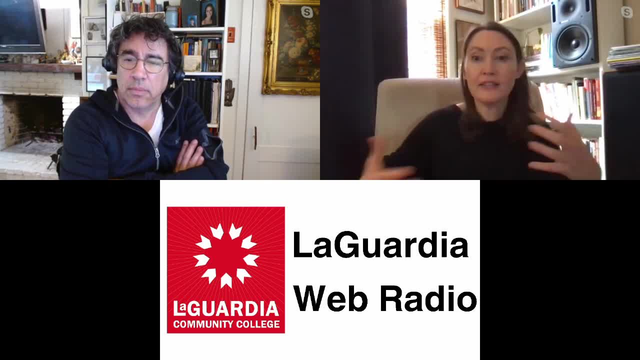 And so I think that's a really good point And have training in this kind of approach to philosophy, but get course credit for it too, so that they can go and do the philosophy in the prisons, They can go and do philosophy in the Queen's Library, They can learn how to create a philosophical web series. 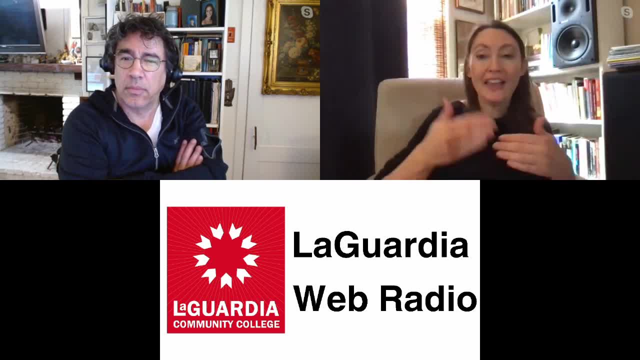 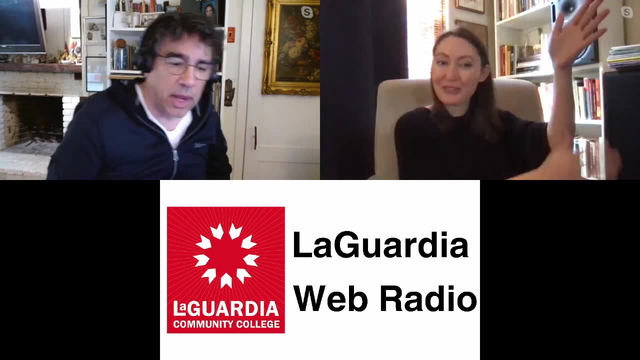 And that's going to give them genuine academic credit And they can then use that right as they go on and continue on, either in philosophy or in the other disciplines that they choose, and bring that experience to bear in those other fields. So that's where, that's where I see our program. 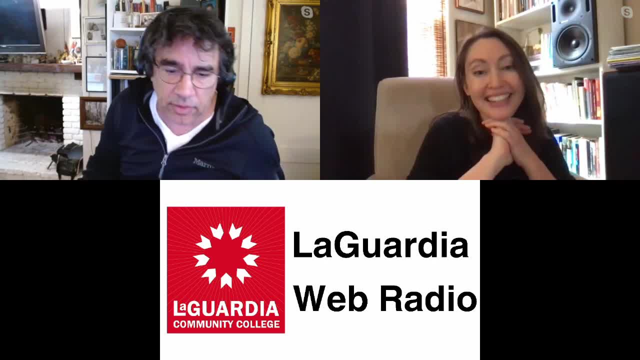 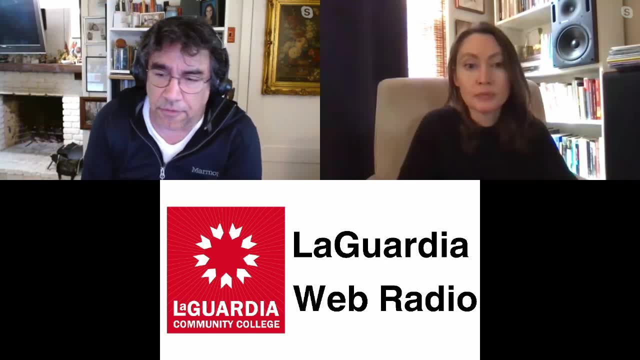 You know I used to run after school programs in the Bronx, a couple of them. You know usually you get the kids at three o'clock or sometime like that. You feed them, you help them with their homework and then, you know, you try to come up with activities for them. 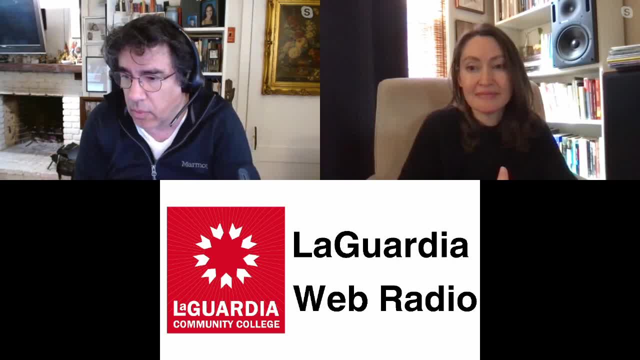 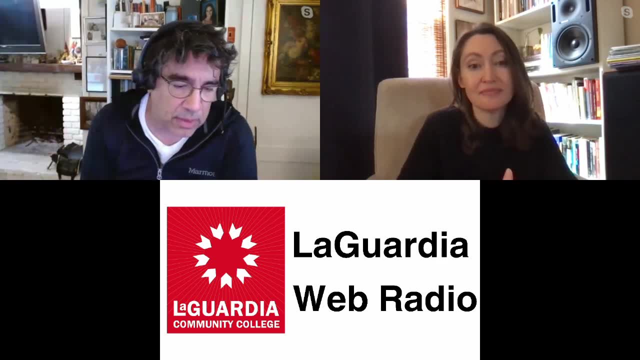 And you know, depending on your population it's you struggle with what people feel comfortable doing. But I could see something like this, you know, or you could see something like this, Or you could see something like this. Or you could train the caretakers, the folks that take care of the students, to have have times like this. 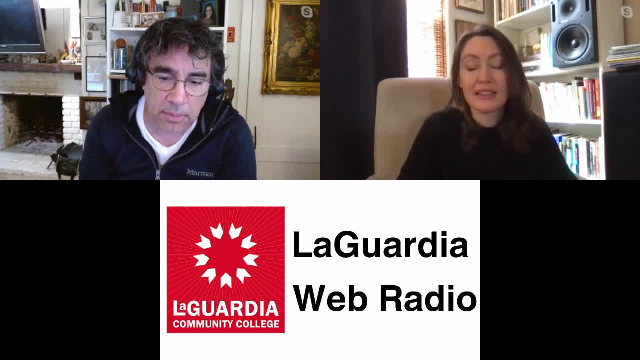 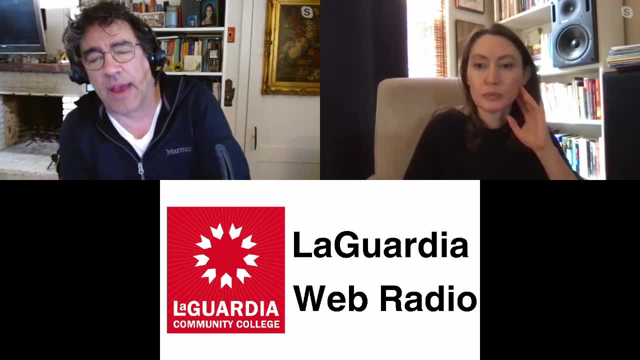 Everybody. let's sit on the rug and talk about. it would be an amazing if it can't be put into the curriculum of the regular school day. It would be something fascinating as after school. Is that something you'd be interested in? Yeah, absolutely. 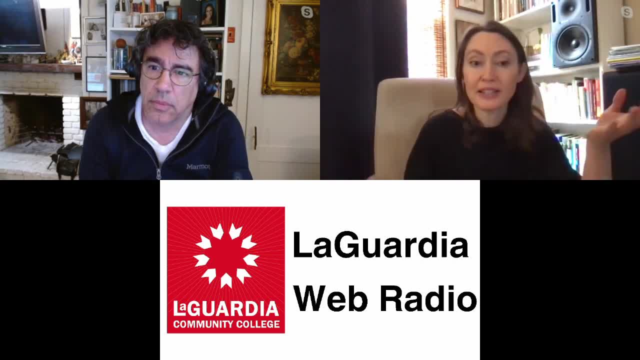 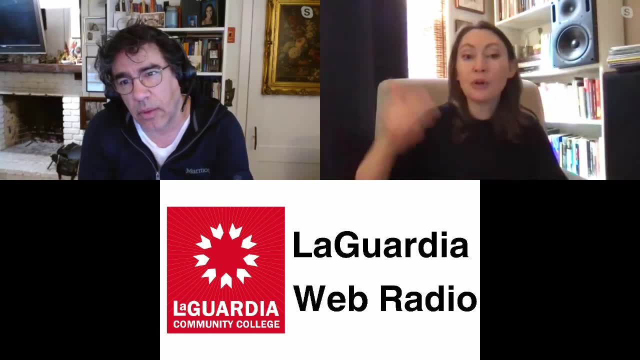 And that's what. that's what I'm doing this semester with philosophy and puppets. It's an after school, It's an after school enrichment that you know it's just me, So you know I'm I can't be everywhere all at once, but would be incredible to be able to connect with other educators who are interested in in similar sorts of ideas, to be able to create something that has a larger footprint. 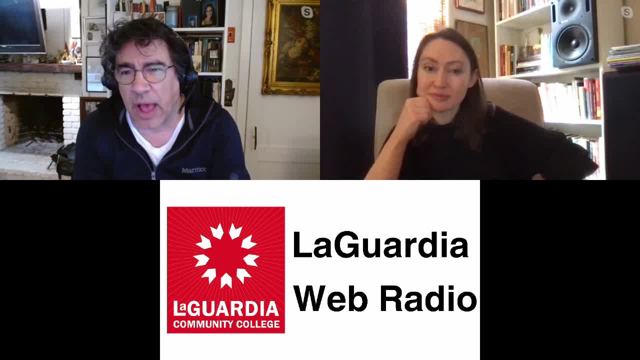 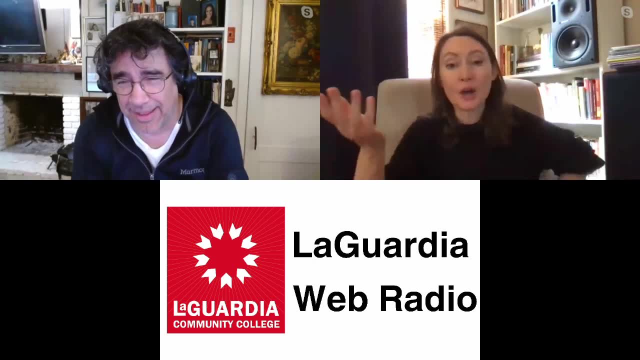 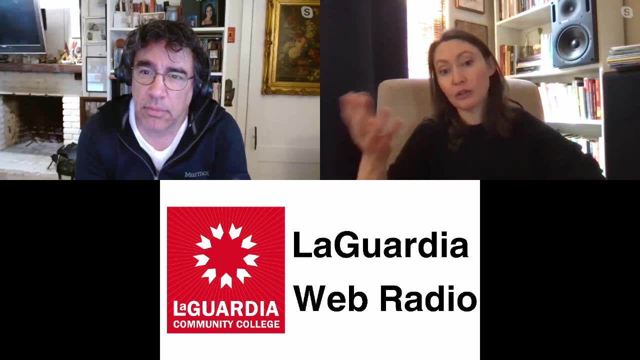 More. Yeah, Have you ever come up with a Socrates puppet and tried to? There are Socrates puppets out there, But so I. my bit from last week was a kind of Socrates puppet, though I called him Pierre for obvious reasons. 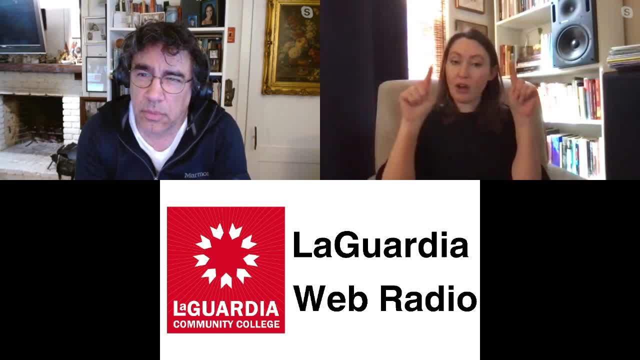 But he had googly eyes and he had question marks all over himself and a little white tuft of fluff right at the top. So very good, And a shabby little robe. You know, he didn't have a robe because he's a rock. 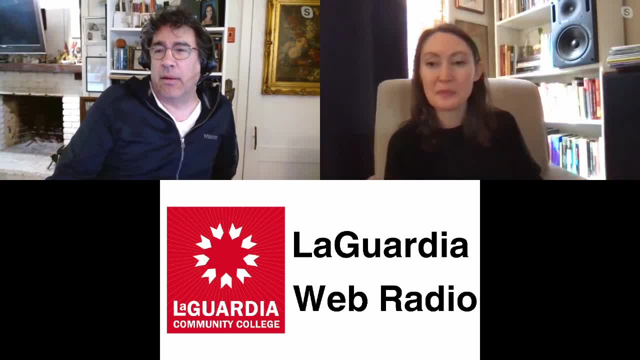 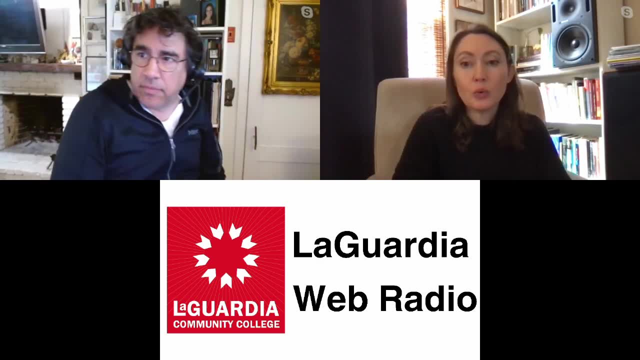 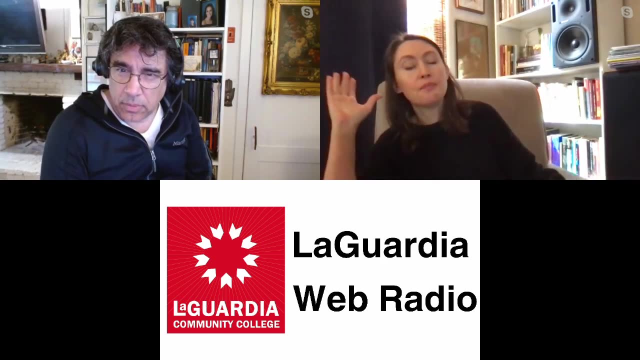 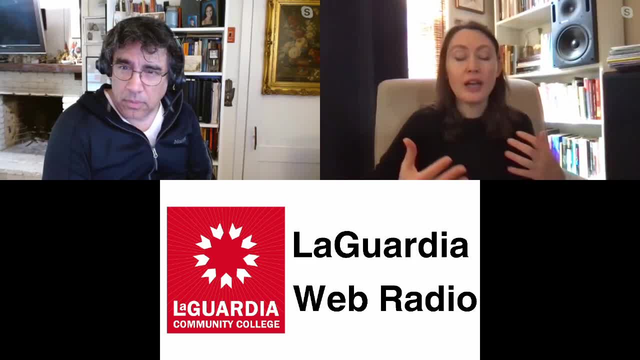 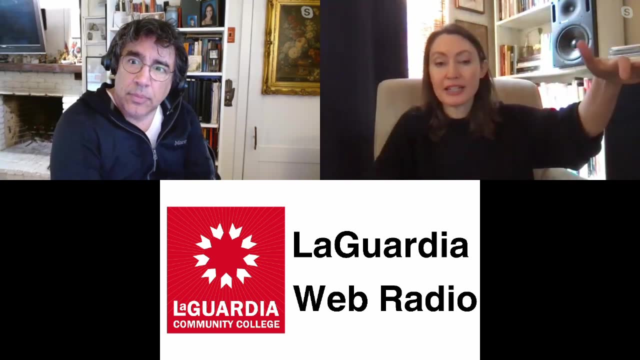 So this is an organization that I'm part of that emerged from My work and Cone Am's work. She's in psychology with the Early Childhood Learning Center and in the Early Childhood Learning Center they do a lot of outreach with our student parents. 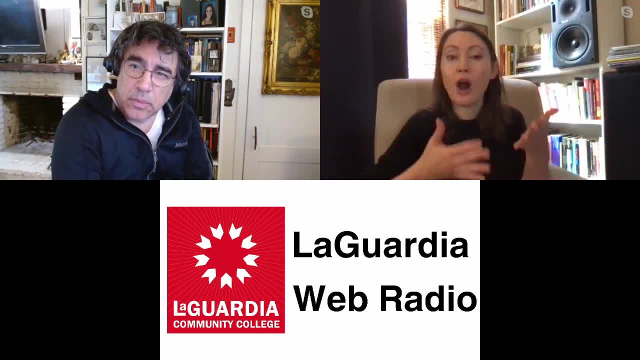 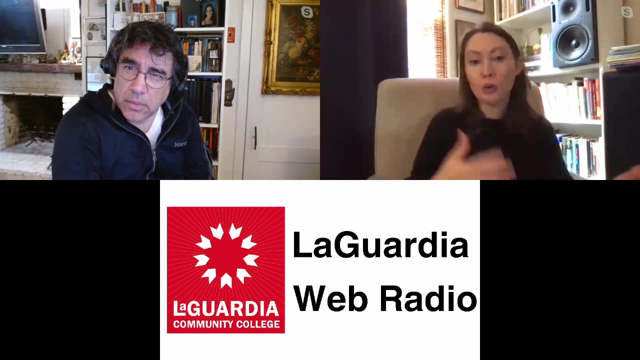 It's primarily student parents whose children are in the Early Childhood Learning Center. And when Cone and I both had our children were very young, we were kind of had this first person view of Of the ways in which LaGuardia was in some ways like very child friendly and in some ways could really improve its child friendliness. 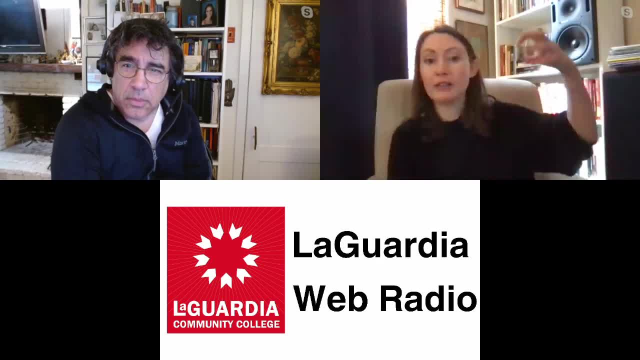 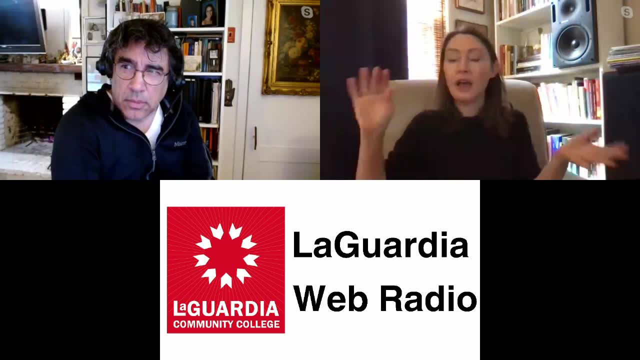 And so this is really Cone's baby- creating the student parent initiative at LaGuardia, where it's a group of faculty from across many disciplines who've come together to try to create a much more welcoming and supportive space for student parents, And we've tried. 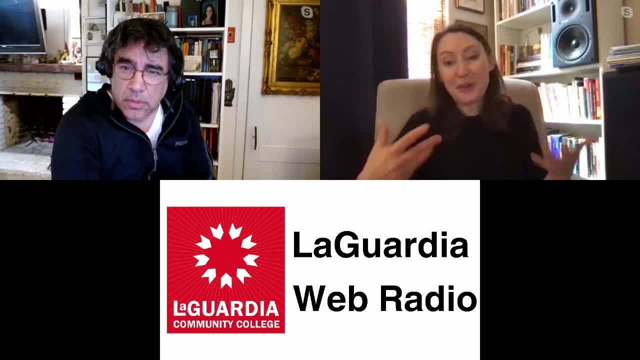 To do that by creating a more child friendly experience at LaGuardia. So we advocated for the of nursing stations on campus. So you may have seen there's actually nursing stations on campus. used to not be the case. We're working now on trying to get those changing tables in all of the restrooms, not just in the women's restrooms. 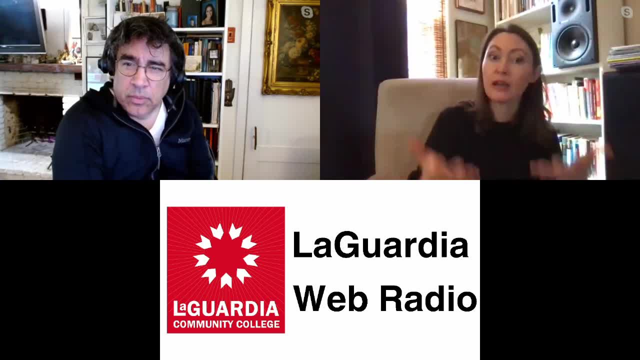 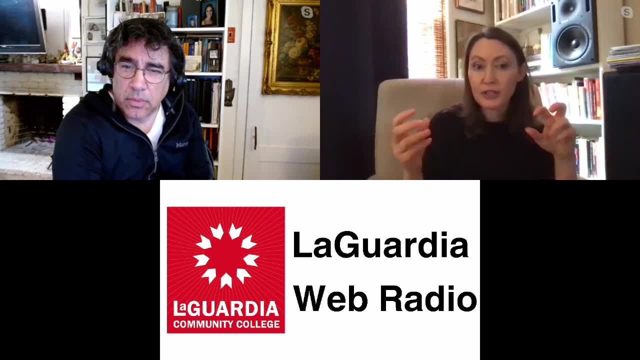 So that you know, Our student parents who are men can also bring their children and change them. We have sort of semi monthly power hours in which we invite student parents and really anybody who's interested to share stories and learn about resources on campus. 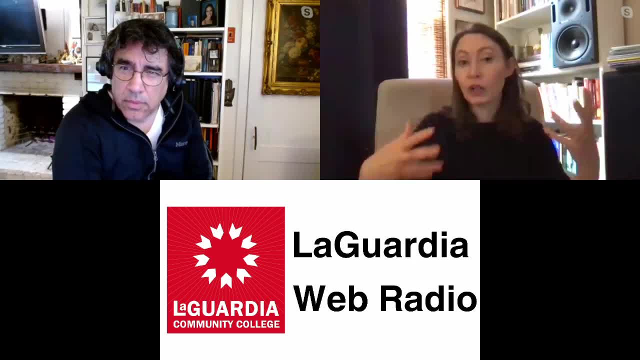 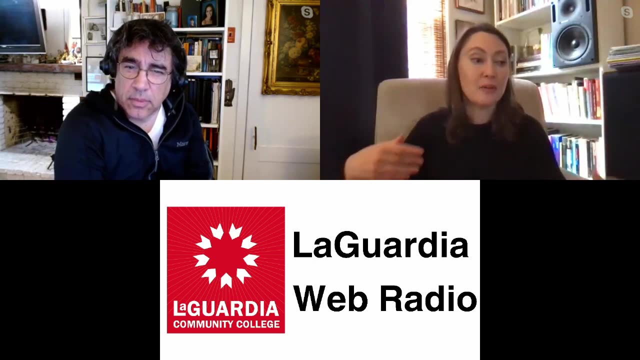 And we are doing a clothing drive that's going to be coming up really soon for children's clothing And, specifically, boutique pop up that will, you know, give away clothes. We'll create a cool space where people who have children can come together and talk and be in community. 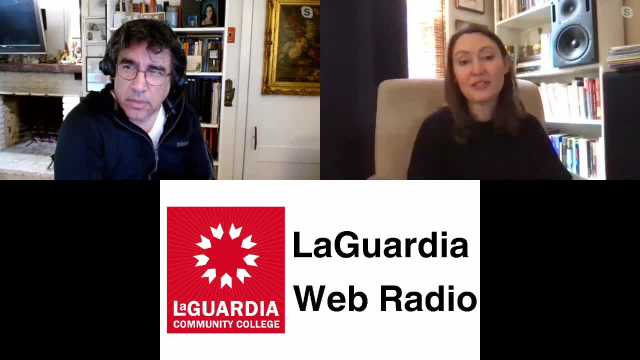 And yeah, so that's what we're doing. These are, these are our initiatives and it's we advocated. I think one of the ways that we were really active on campus was in pushing for that children on campus policy for students and for faculty and staff, and making that to be as open as we possibly could. 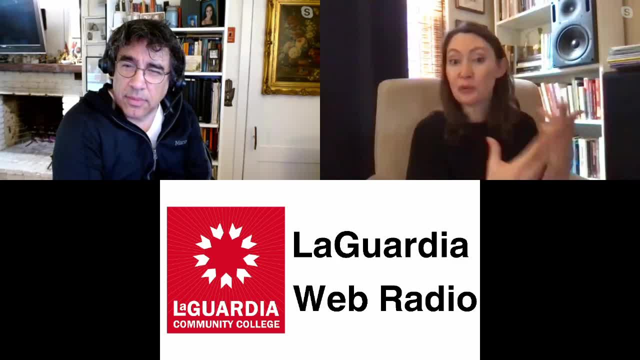 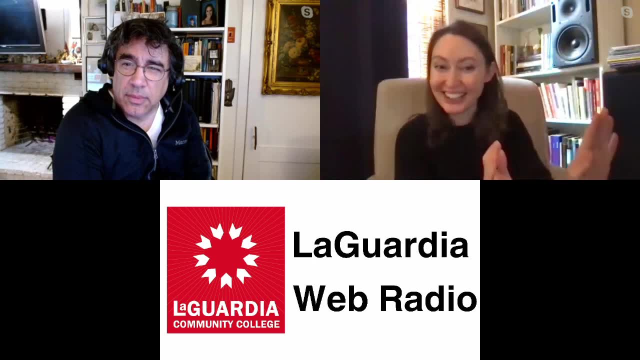 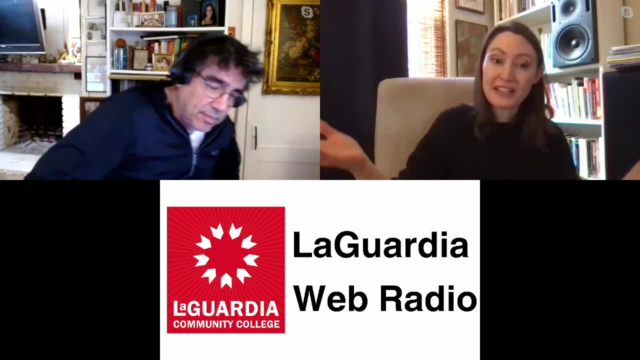 Have it, And I think we were really successful with that, because, as it started, they did not want to allow children on campus at all, And now children are allowed on campus, but they do have to be supervised, So which makes sense. So that's the work that we're doing. 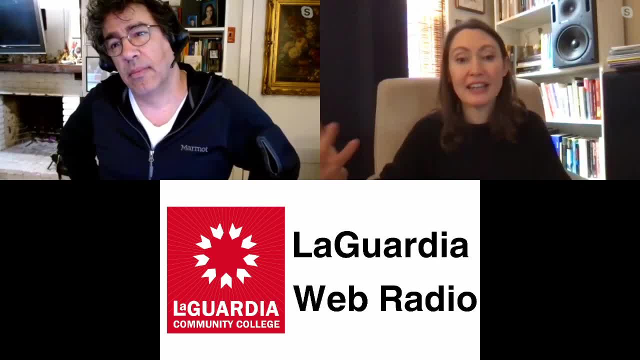 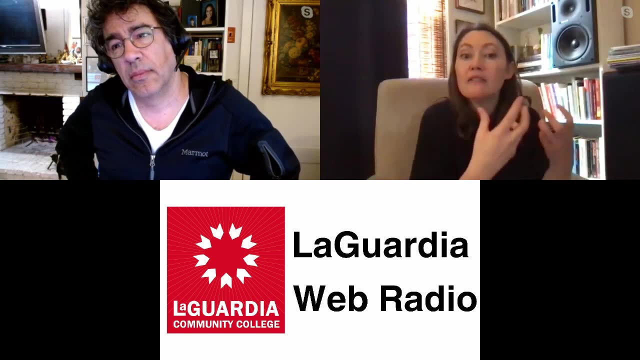 If people out there want to be involved in, you know, making the campus more child friendly. There are a couple of things that we're doing. One of the things that you can do. One of the things you can do is actually put language on your syllabus that talks about what your individual policy is about children in the classroom. 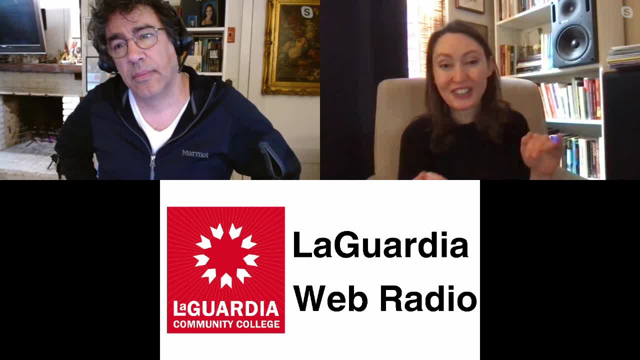 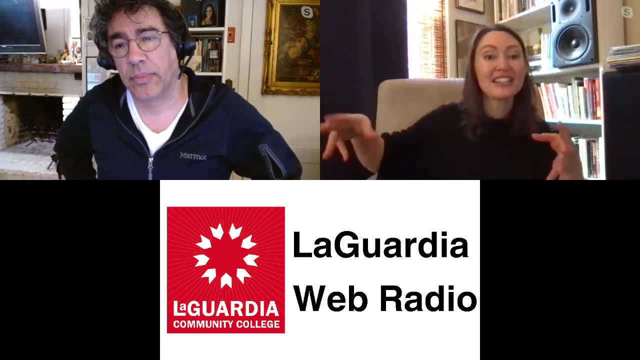 It is typically the case that students not want to bring their children to campus. Right, They're here to learn. It's a kind of escape sometimes from the difficulties and challenges of your everyday life. You get to come and have this, this space. 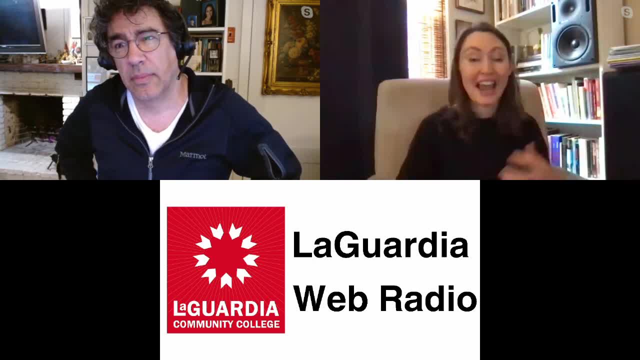 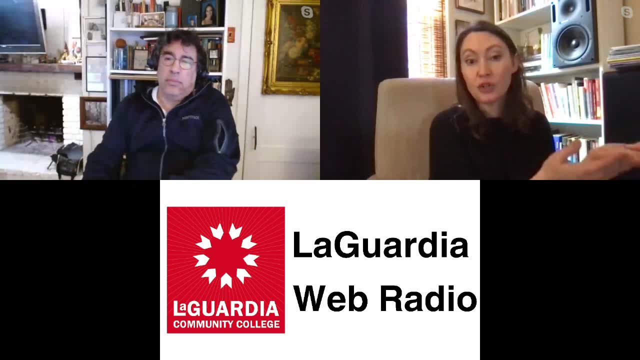 It's also the case That sometimes life intervenes, And is it better for them to stay home with their child if they have to, or is it better for them to bring the child to class? Having something on your syllabus that says that is, I think, really helpful. 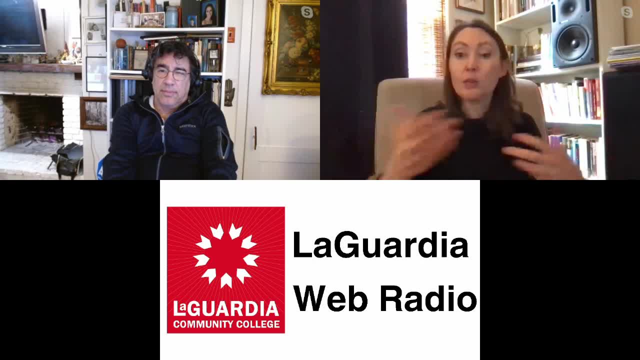 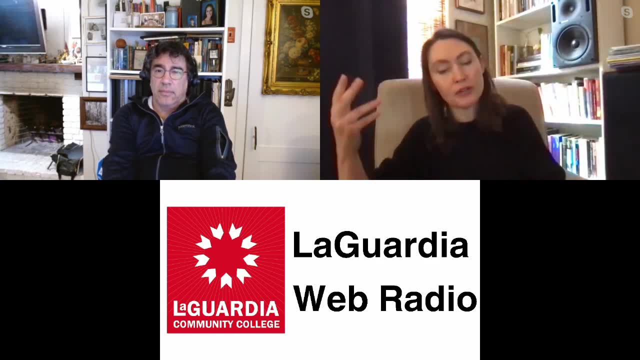 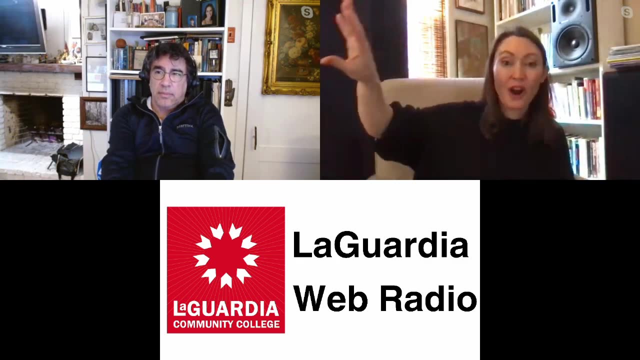 What your specific policy is. Another thing we can do is when we're hosting events on campus, which all of us do, Right, We're hosting events on campus all the time Asking ourselves: are these events kid friendly? And if they are saying that, I know they do this at the, at the astronomy events where they say: bring your families right. 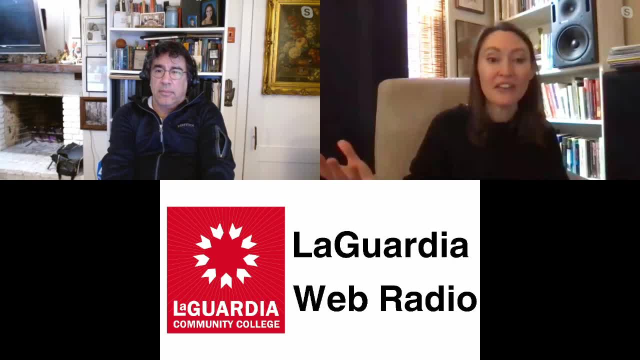 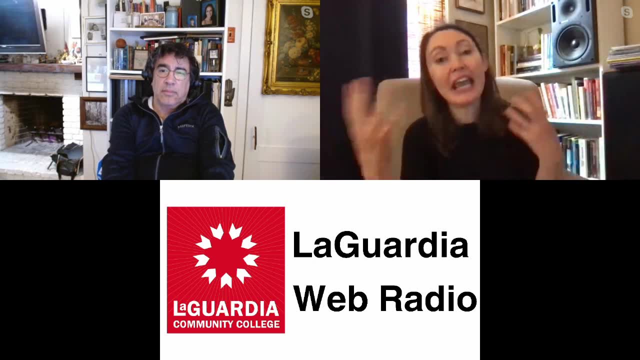 Bring kids. like it's cool, Like this can be a cool community event. I think that I would love to see all of the events on campus saying explicitly, if they're kid friendly, that kids are invited. If they're not, that's OK. 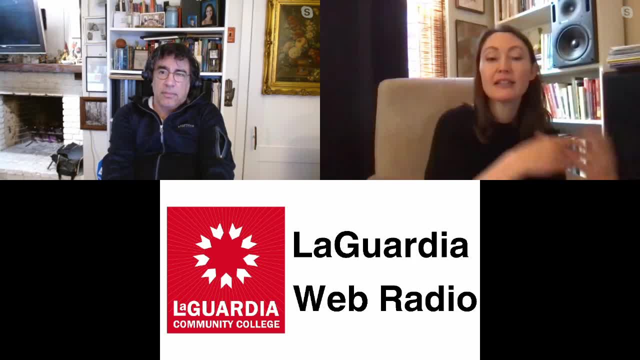 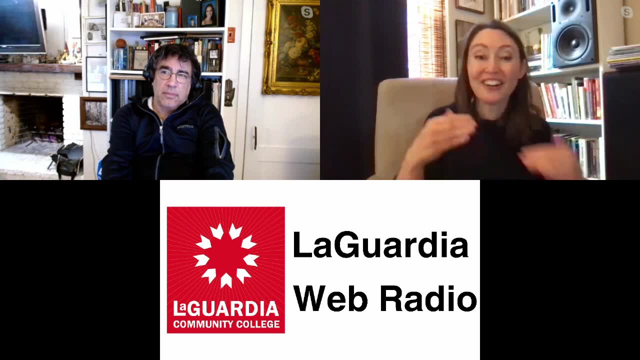 Right, Not everything has to be has to be for kids, But if it is, I think it goes a long way to making that space. I think it goes a long way to making that space a space in which children are welcome, children are encouraged. they are not our current students, but they're future students. 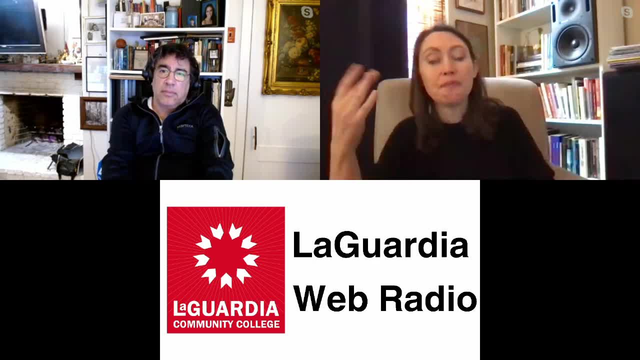 And speaking of psychology, I love Alison Gopnik. she's a child psychologist. Alison Gopnik has this wonderful metaphor of the relationship between the ways in which children think and the ways in which adults think. Children are the kind of like. research and development department. 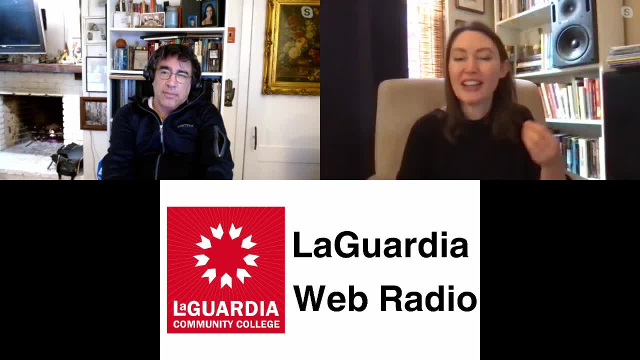 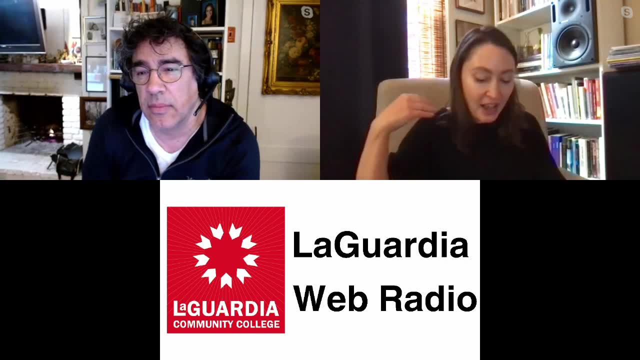 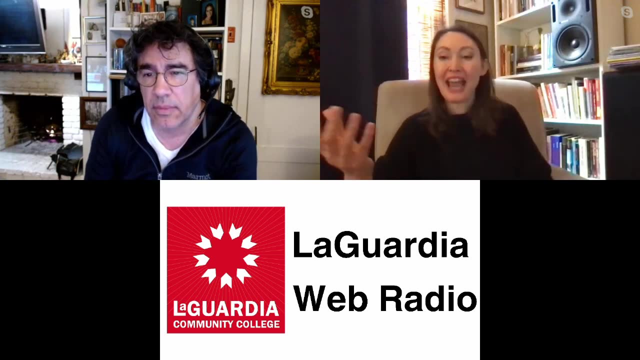 Of humanity right, They're the ones with all the creativity, all the imagination. They're the ones they're research and development. And then adults are more like the are more like the production and marketing department, right, And what would production and marketing be without research and development?